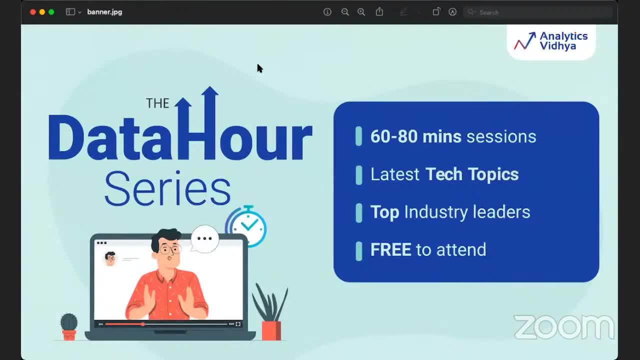 Thank you. Hello everyone, Welcome to the another session of Data Hour series. We'll be starting the session in five minutes. Till then, let's get to know each other. We have put up a poll. Kindly answer the question. 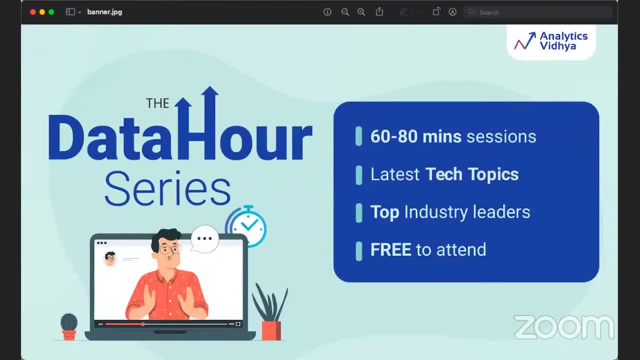 We'll be right back. Thanks everyone for joining us today. We'll start the session in two, three minutes. 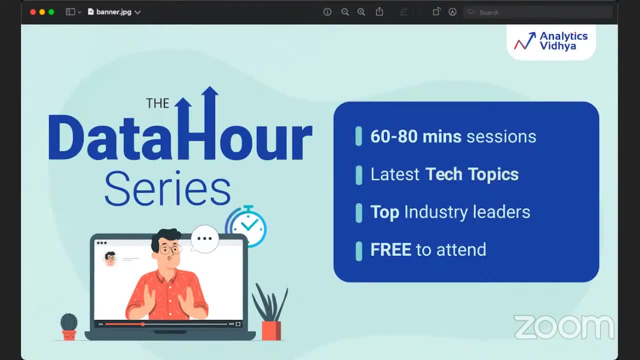 Let's wait for everyone to join and settle in. We'll be right back. Hello there. How's everybody's afternoon going? That's great to hear. Okay, hope everybody have your lunch. Thanks for joining in at this time actually. 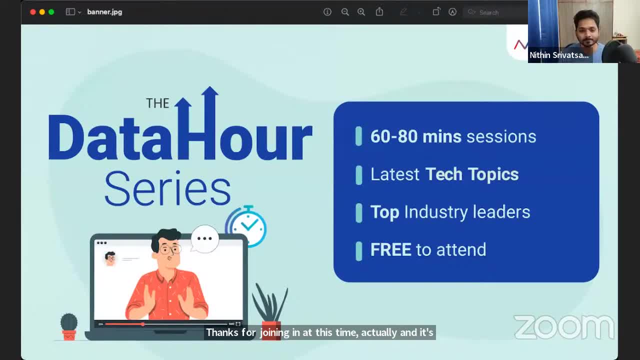 It's lunchtime- almost Good afternoon, Netin. Good afternoon, Yeah. So we'll start with the session. So hello everyone. Welcome to another session of the DataR series. We will start in just one more minute. Till then, let's get to know each other. 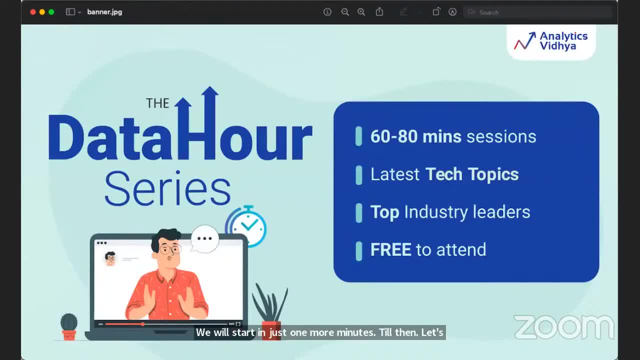 We have put up a poll. Please kindly answer all the question and we'll start the session in just a few more seconds. more, Yes, So hi, and welcome everyone to the another session in the data series. We are thrilled to be here with you this evening for a session full of action-packed learning. I am Diksha. 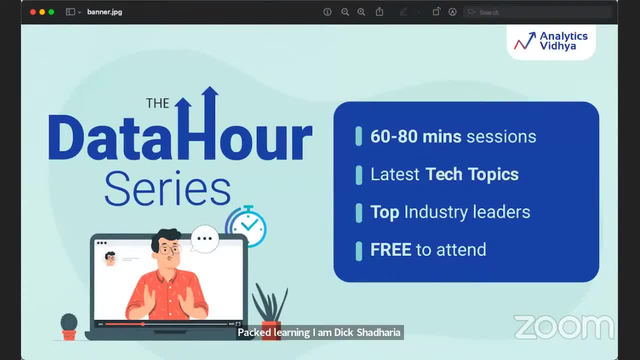 Dharia, part of data science team at Analytics Vidya. For those who have joined us for the first time, a brief introduction to the data session. The data is a series of webinars conducted by Analytics Vidya and led by top industry experts. It's a fun way to understand. 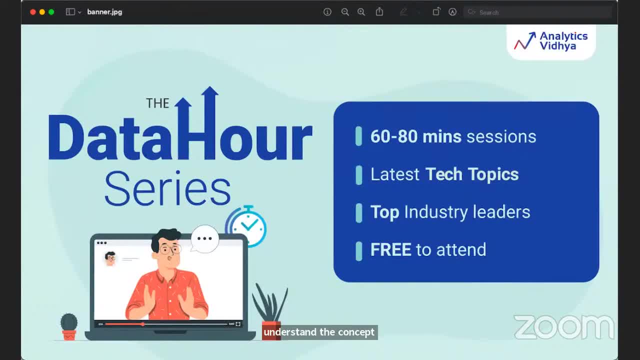 the concept of data science, data engineering, software engineering and blockchain from the leading players in the industry. We are hopeful that these sessions are going to be a great source of enrichment and value-adding for our community members. Now on to our session. 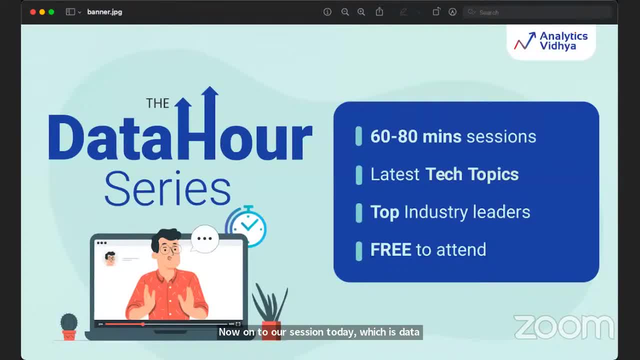 today, which is data wrangling using geospatial data in Python. Geospatial data is a world unto itself, having lots of format, lots of file types, lots of information all within a single file. In this session, the speaker will discuss: 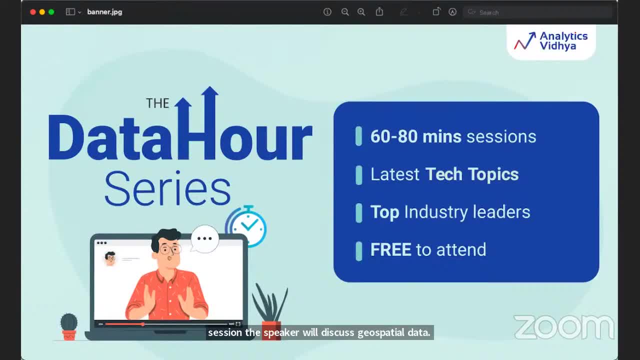 geospatial data, the representation of 3D view of the earth on a 2D plane, ways to access various satellite format, available Python libraries for geospatial data application geofundas and basics of the data plotting. So, before we kick things off and I hand it, 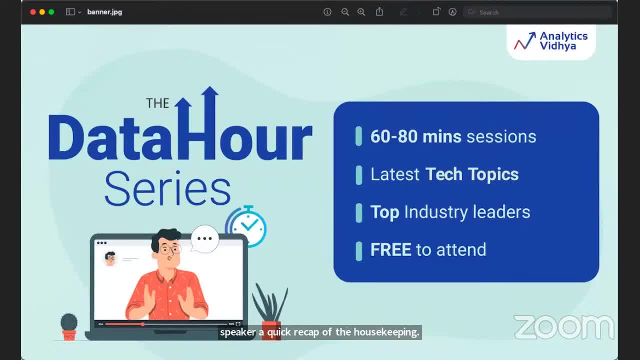 over to our speaker. we are recording the session and the recording will be live on our YouTube channel, The link you can find in the chat section. Please use question answer for asking any question you might have during the session and we will do our best to answer. 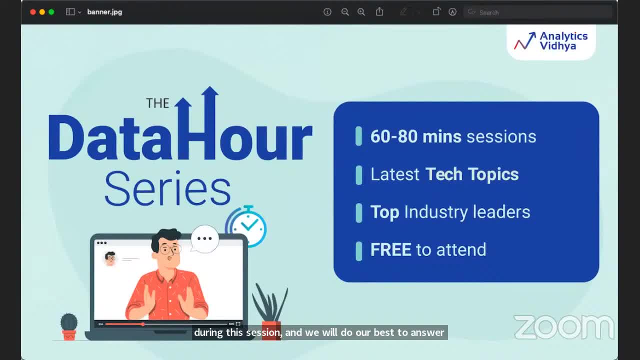 them as the data progresses on towards the end, We will be sharing a feedback poll towards the end. You all are requested to kindly fill up that the form before leaving the session. Now on to our speaker On this session of the data we have, Nitin Srivastava. 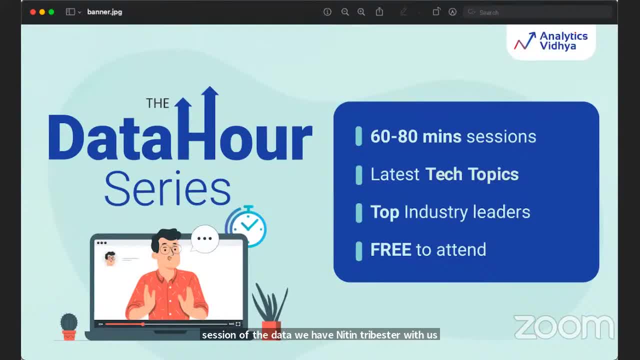 Nitin is a passionate data scientist who loves solving problems. In the last four years of experience, he has built multiple end-to-end pipelines for environmental intelligence in ad tech and digital healthcare spaces and is currently working as senior data scientist at Ambi. You can connect with him on LinkedIn. The link is present in the chat window. We 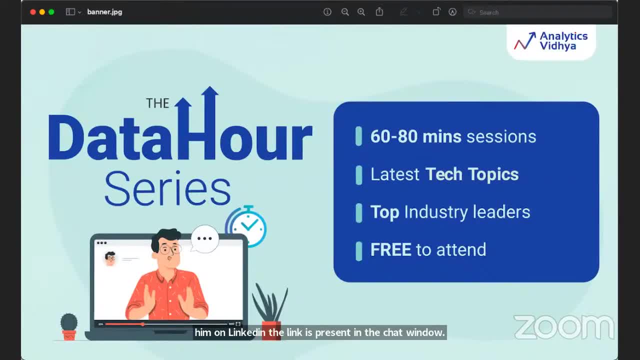 are also hosting this webinar live in our YouTube channel, and the channel link is present in the chat window. You can even follow up from there. Thank you Over to you, Nitin. The virtual stage is all yours, Thank you. Thank you so much, Deeksha. I hope I said that right. Okay, So let me just share. 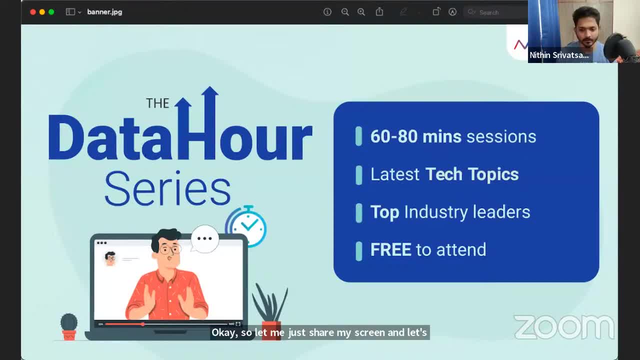 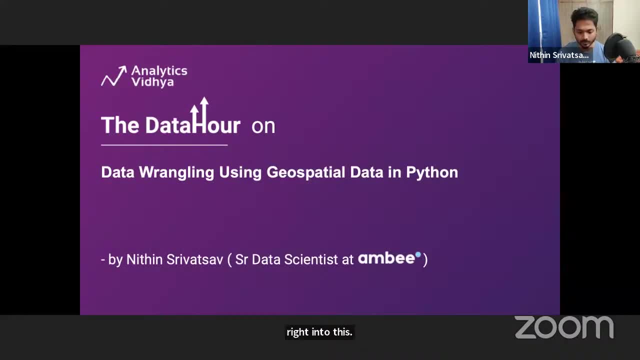 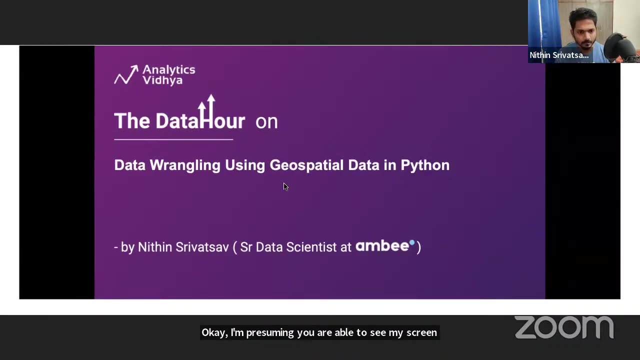 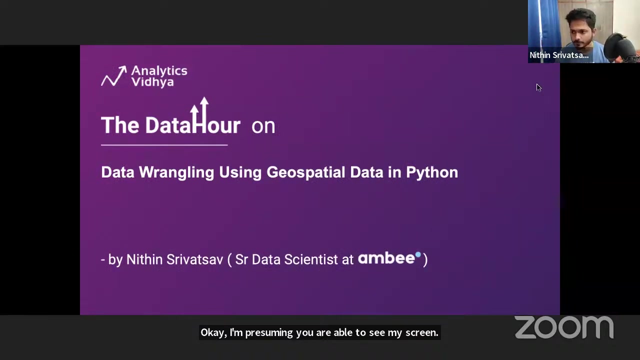 my screen and let's dive right into this. Okay, I'm presuming you're able to see my screen. Okay, Cool Right. So, hey guys, Welcome to today's data session And we'll be working with geospatial data in Python. We'll look at various types of data. We'll look at the 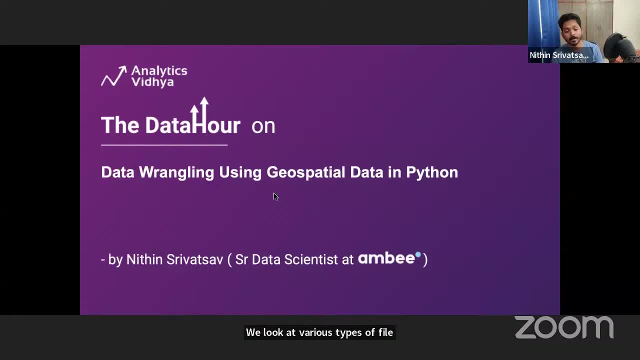 data in Python. We'll look at the data in Python. We'll look at the data in Python of file formats, various types of plottings and we'll see how to access satellite data, how is it stored, and a little bit of plotting on QGIS and it's going to be lots of fun. 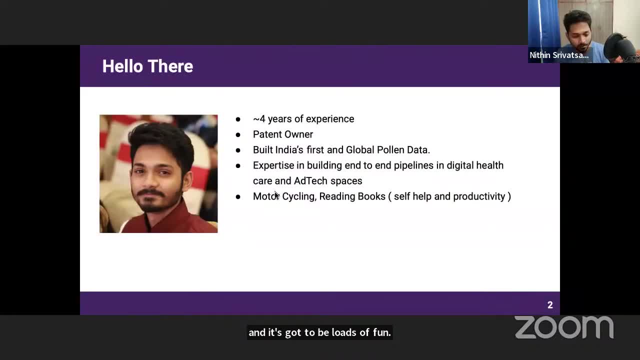 So, before we get started, I'm Nitin Srivatsav. I am a senior data scientist at Ambi. I have close to four years of experience in building multiple end-to-end pipelines, especially in the digital healthcare and attics spaces, and I own a couple of patents. There are some. 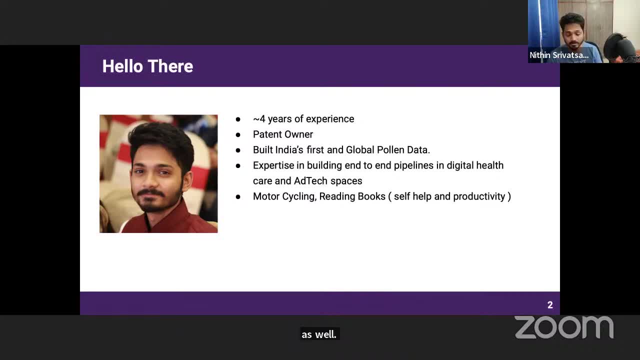 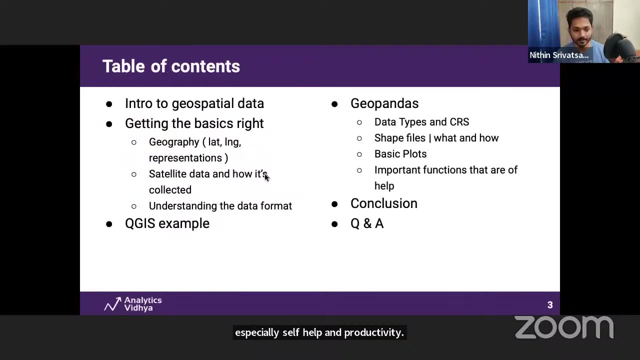 in the way as well, My team and I. we built India's First and the global Poland data, which is available on our website. Ambi Hobbies include a little bit of motorcycling and reading books, especially self-help and productivity. Okay, enough intro about me, Let's dive into. 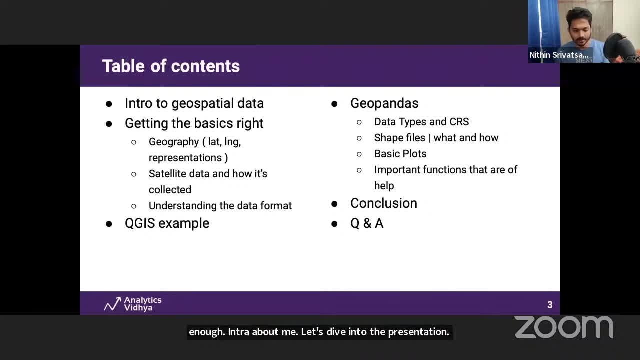 the presentation. So here is what you'll be getting to see in the presentation, The table of contents. First we'll understand what geospatial data is, where is it used, how is it useful, and then we'll get our basics right. We'll understand what is a lat-long. 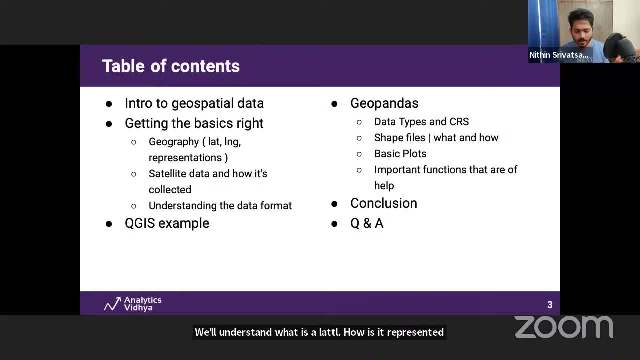 how is it represented? what are coordinate reference systems? how is a 3D view of the world presented as a 2D plane and understanding some specific data formats? We'll look at an example of QGIS and how we can visualize that, and then we'll deep dive into Geopandas. 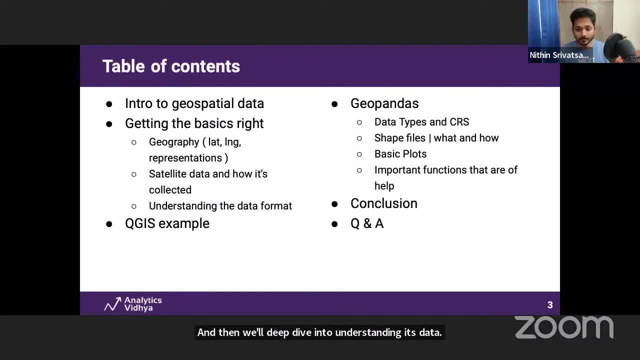 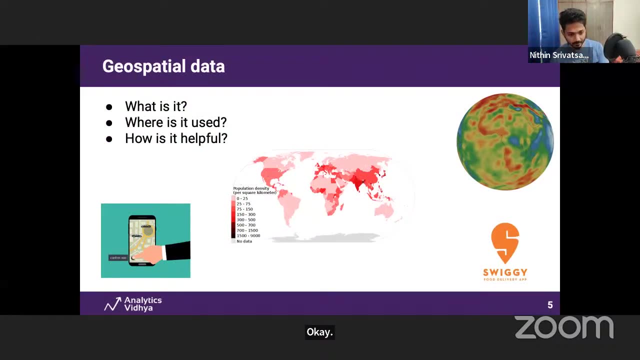 its data types, shape files, a little bit of basic plotting and important functions that are of health And finally we'll conclude and we can get on with the QA session, Right, okay, So what is geospatial data? Any data that can be referenced to a point on globe. 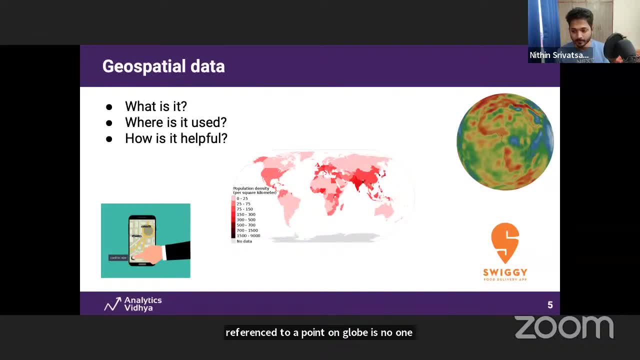 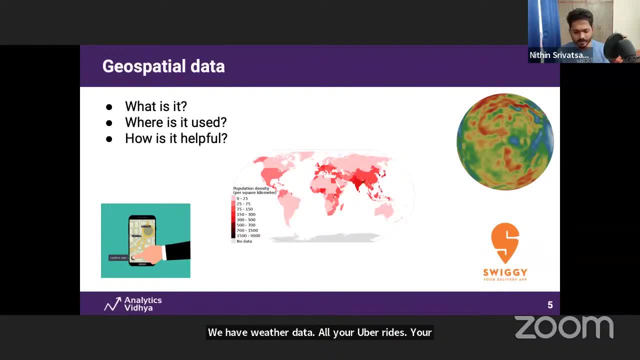 UberRides, your Swiggy Zomato orders your Myntra. Flipkart orders. everything has a data point link to it. So when you make an order on Flipkart, there is your home address which is linked to a point. Now in Flipkart's backend servers they store it in a way which can further be used to. 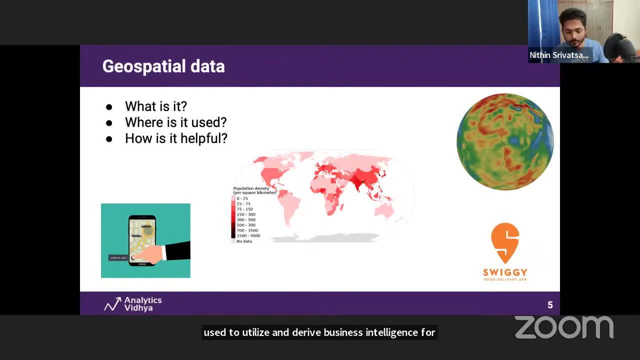 utilize and derive business intelligence. For example, which area took a lot of orders or where did most of your orders go, Where did most incoming come from And what were the products? Everything can be referenced to a point on map And using that we can derive business intelligence. 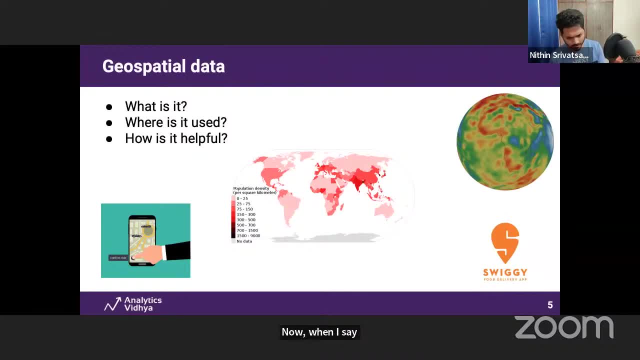 Now, when I say business intelligence, a lot of applications. So say, for example, we have Uber's data, So Uber has collected all your rides of everybody in a locality and they plot it on a map. Now we can understand which time of the hour has a lot of traffic, so that I can add more cars there, so that my order 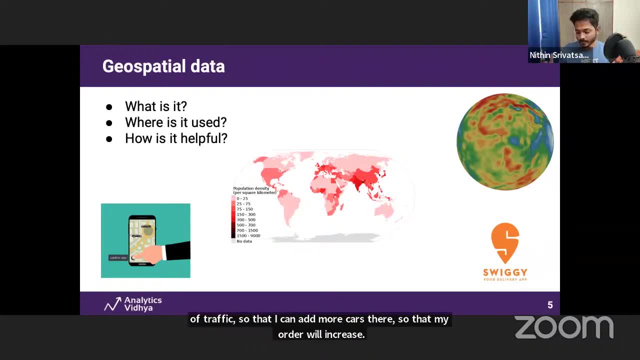 will increase. Similarly, there is weather data. you know, say, you're planning a Goa trip and you want to know what's the weather there, So you go to Google and you check Goa's weather. Now, their backend- there's a location for Goa for which weather data is mapped, which is being 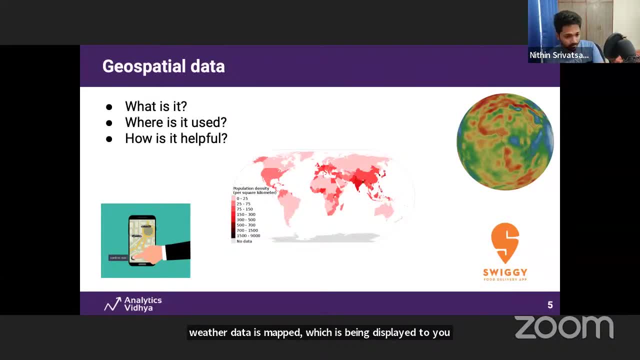 displayed to you. So here are ways. here are the places where geospatial data is used. There are very numerous amounts of users that geospatial data has, say, for example, COVID-19 dataset. You know, back then, when there were there was restrictions and curfew, we could. 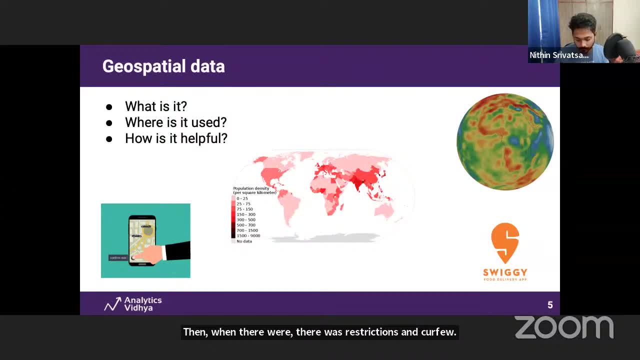 know where a lot of COVID cases were coming from. We can plot an entire heat map of where COVID cases were there. So these are some of the applications that geospatial data holds for us. So now let's look at the backend, or how geospatial data is used. So let's look at the backend, or how geospatial data holds for us. 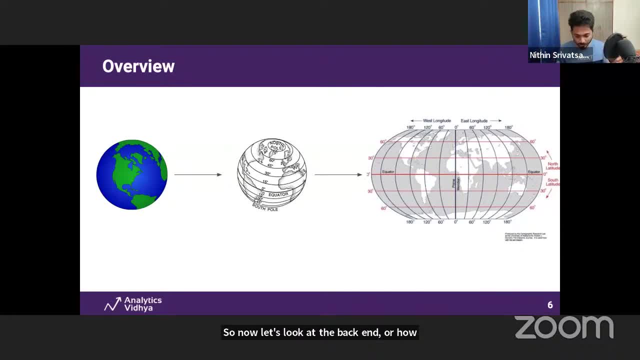 That's how geospatial data works in the backend. What's the fun house about it? So you have your globe, and then that globe is divided into long latitudes. You have your equator, you have your Tropic of Cancer, Tropic of Capricorn, your North Pole, South Pole, and then you have longitudes. So this is. 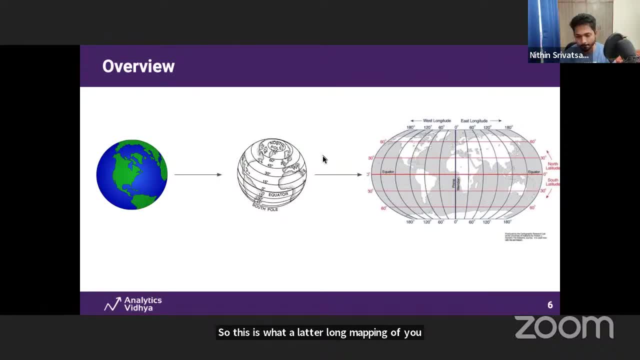 what a lifelong mapping of our globe looks like. But now what if I tell you the map that you see, the map that we have known from our childhood? the world map is not exactly how it looks. it looks like this. the world looks like this. so the sketch you can see is what we see on the world. 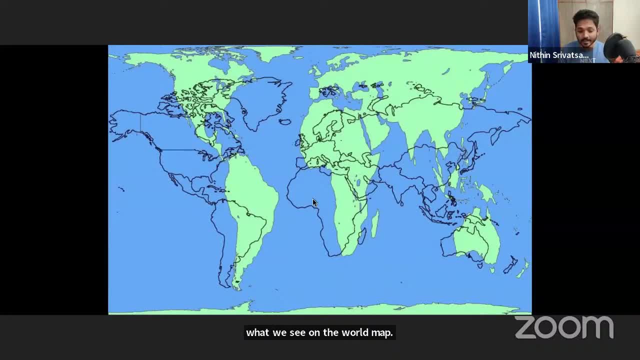 map. but actually, if you take into relative distances into consideration, this is how the map looks like the green part it's it's stretched. but what we do is we use an accepted standard, that is coordinate reference system, and we show it in a concise way that is accepted universally. 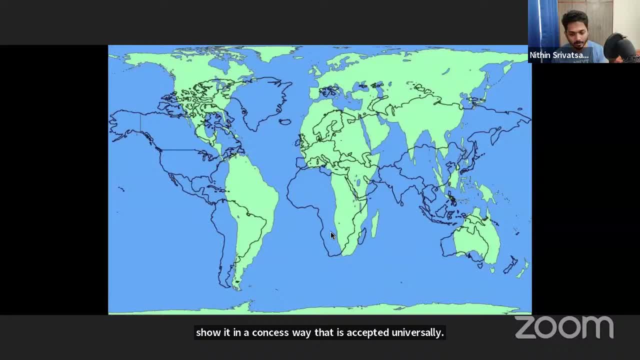 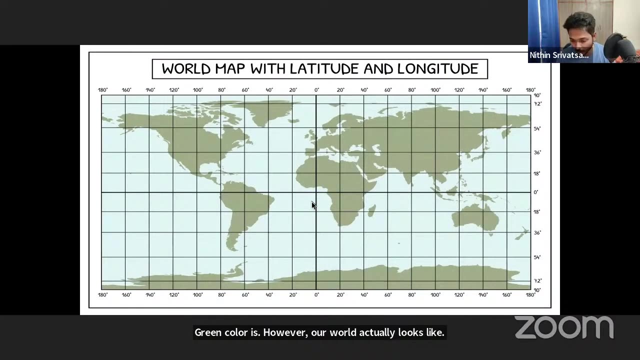 so? so the black sketch is what we see on the world map, but if you look at the relative sizes of how they look, the background green color is how our world actually looks like. so now that brings us to the map, which is lat and long. so everything to the right side of this. 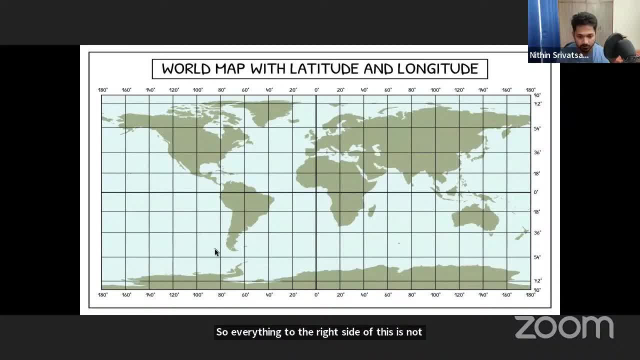 is east, this is west, the top portion is north and the bottom portion is south. this is one way of representing it. say, 12,77 is 12 north and 77 east. so if, if we were to take an example of bangalore which, whose latitude and longitude is 12,77, what i would do is i would go here to 12. 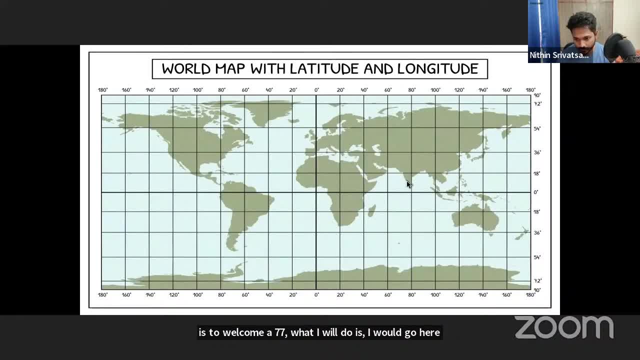 almost, and then i would go to 77 here, and then i would go to 77 here, and then i would go to here, which almost comes down to here approximately location. so this is how we map a lat long to the entire world map. so right side is positive. 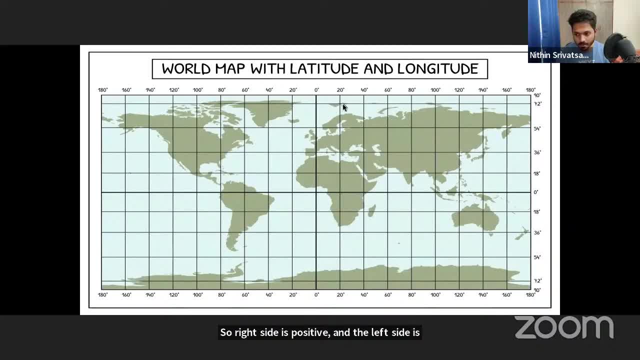 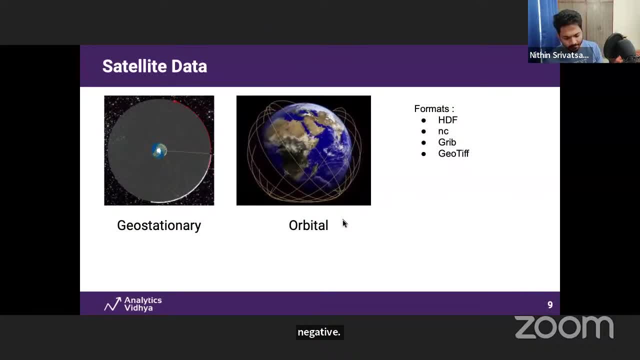 and the left side is negative, the top side is positive again and the bottom part is negative. okay, now let's move on to satellite data. so in this specific website or in this specific slide, we throw here two lines down, here two wireless data. we say the operation data and this is the. 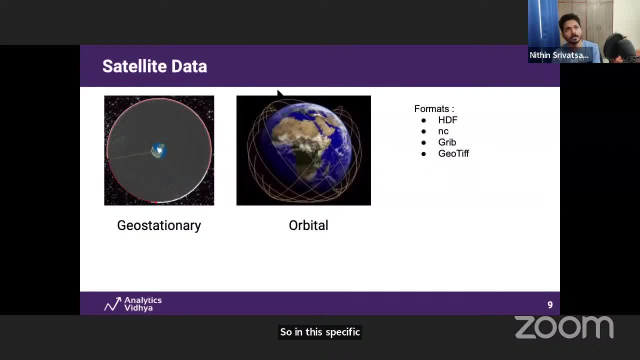 result of that course. here we We'll understand what satellite data is about. Now we will be skipping all the Ubers, Wigi data sets and we'll be looking at weather data, pollen data, anything that deals with satellite data- okay. 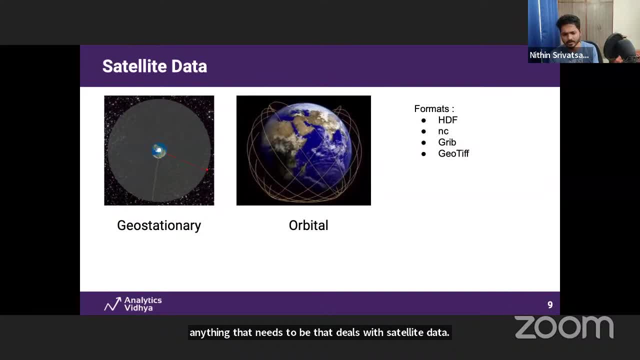 So there are two types of satellites usually which collect the data, which are geostationary and orbital. Now, what geostationary does is it is fixed with reference to the globe, So as and when the globe moves, the satellite moves in the same way. 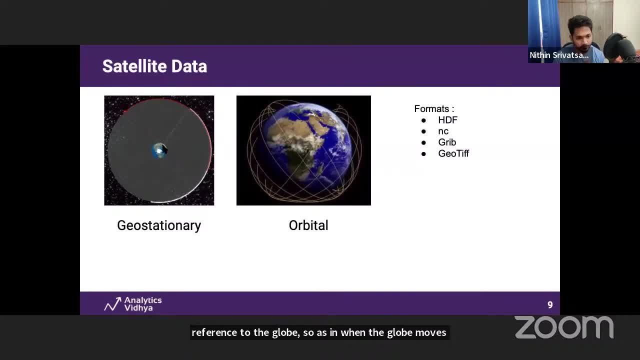 So you can see, here on the left-hand side it is in the same position as the globe, So it is revolving with the globe. So for a person standing on earth he would see the satellite as motionless. but in actual 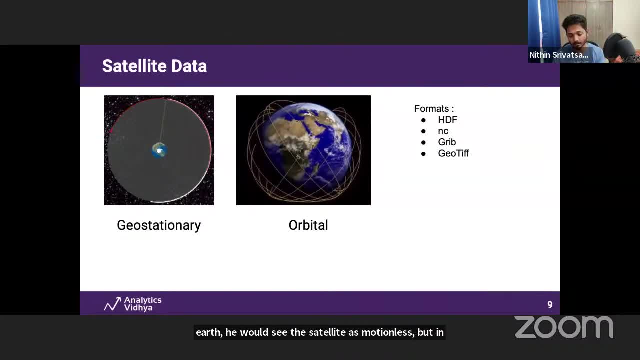 it is moving, And the second type of data sets are orbital data sets. Now, what this do is it orbits. It orbits around the earth in its own fashion, in its own orbit. Now you can see here. So what it does is, if this is the globe, it moves in circular motion around the globe. 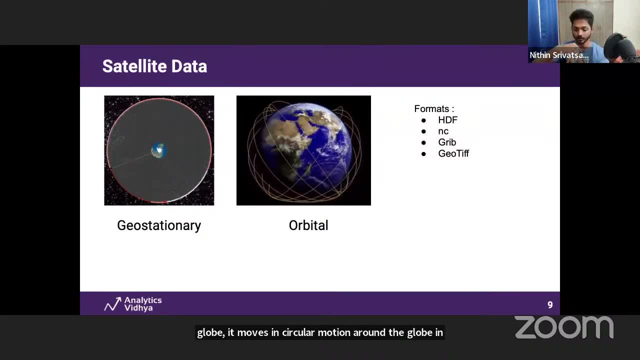 in its own orbit, covering all parts of the globe and capturing data that's relevant to it. Now, a typical weather data or a satellite data that consumes information almost accounts to 100 TB of data. Now, that's a very, very large chunk of data. 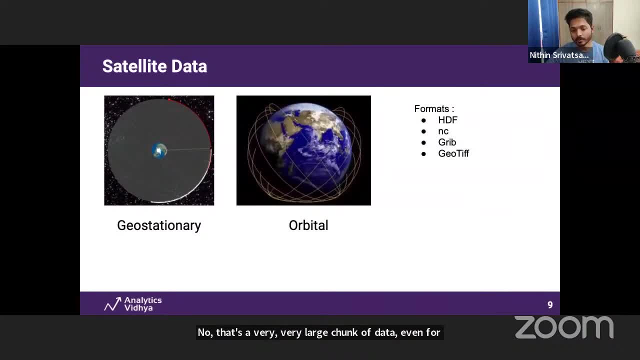 Even for us Just to process on the local systems. what these weather or satellite data providers do is they have very high resource, rich computers, supercomputers even, and they process that data and they pack a lot of data, a lot of information, into a single file. 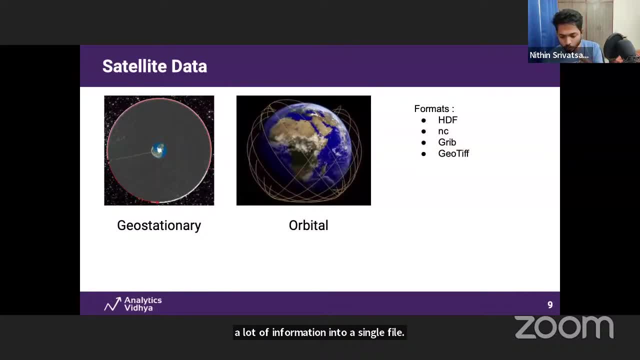 Now that file will drop down to say 2 MB, 3 MB file, but it contains a lot of information and it's packed so closely together in a space, So in a specific format because of which the file is soulless, else it would have taken. 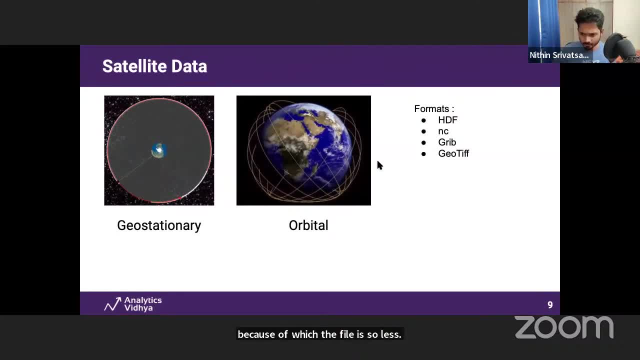 100 TB of data. that which really huge. So there are some common formats that satellites use, uh, which is HDF files, NC files, there is grip and there's also geo-tiff files. We'll be exploring uh- HDF in subsequent slides. 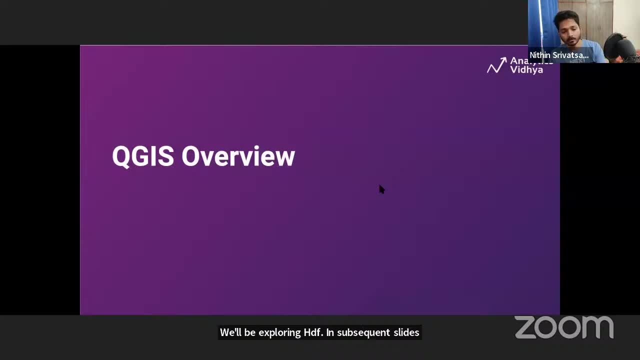 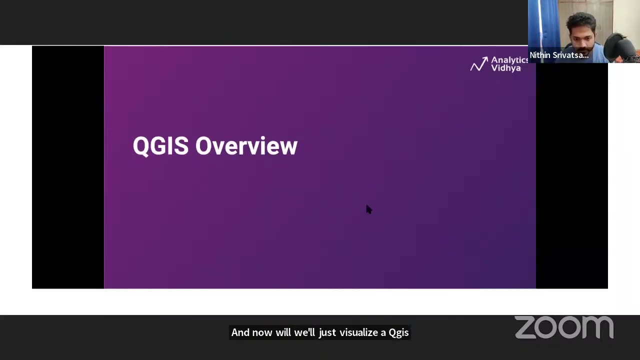 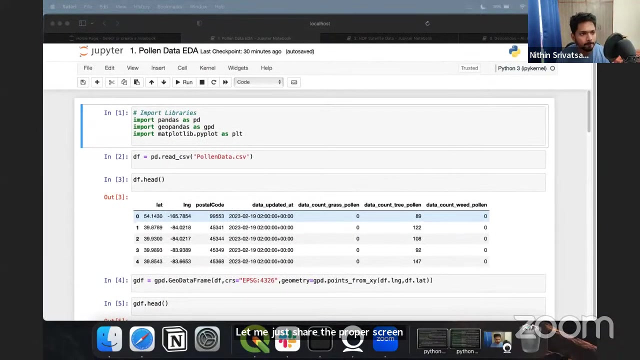 And uh, No, we'll, we'll just visualize a QGIS uh, Poland data. Now, before that, let's: uh, first let me open that just a second. let me just share the proper screen, okay, so i presume you are able to see the notebook. 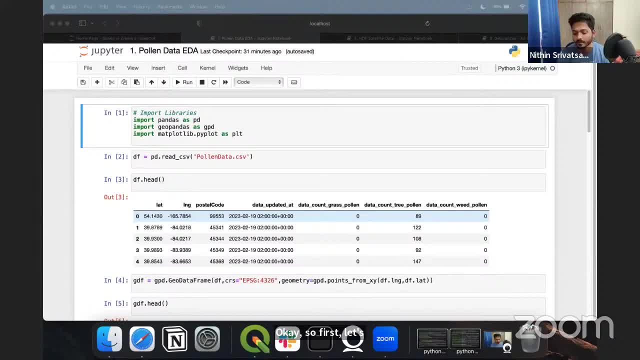 okay. so first let's see what type of file we are looking at and how that can be visualized in qgis. so let's just import our libraries and let's also import a geocache pandas library, which you will understand why we are doing that in a second. 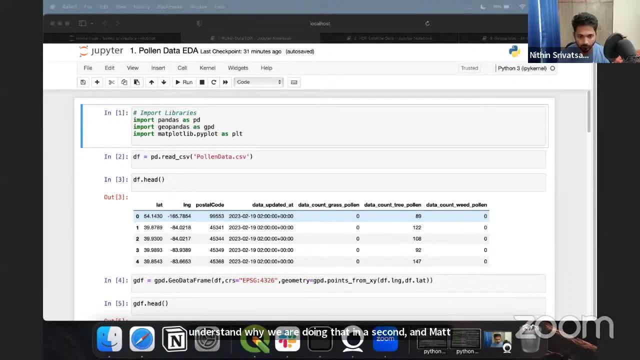 and matplotlib library for plotting. now i am assuming you already have enough experience with pandas, data frames and plotting, so that this isn't very new to you. let's just read the data set, which is colon data dot csv. so let's just look at the head of the data. 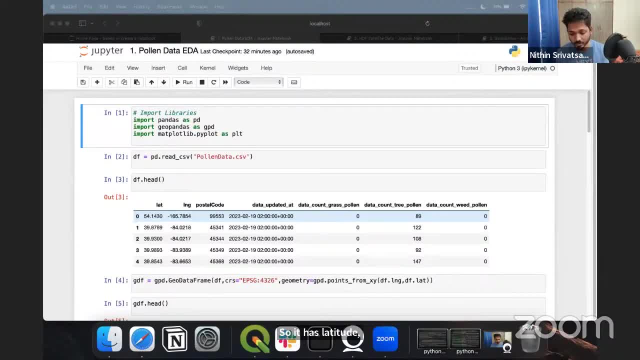 so it has latitude, longitude, so that's geospatial data. we have a postcode, we have created a timestamp. there is grass, poland, this tree pollen, and there's wheat pollen. okay, now let's just create a geo pandas data frame. now, stay with me here. uh, we i'll be explaining that in subsequent slides. 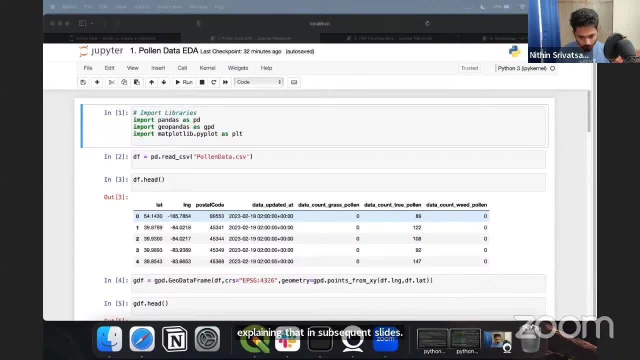 so let's create a geo data frame which uses geopanda's library and creates a geo data frame. now this might be new to you, but if you're a beginner, so i'm going to give you a bit of time in this video to show you the following data. 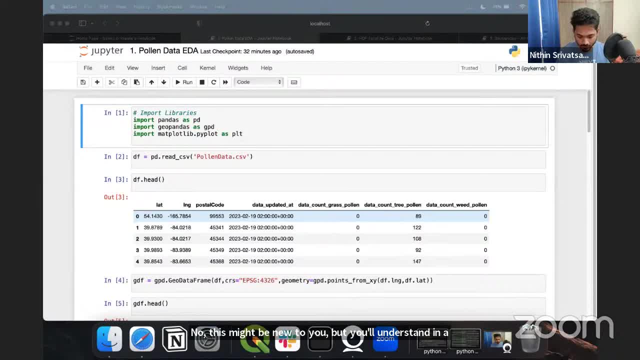 but you'll understand in a second how this is happening. We have EPSG 4,, 3,, 2, 6.. So this CRS, which stands for Coordinate Reference System, is the generally accepted standard globally for a view of a map. So in the previous slide when I told there is a general 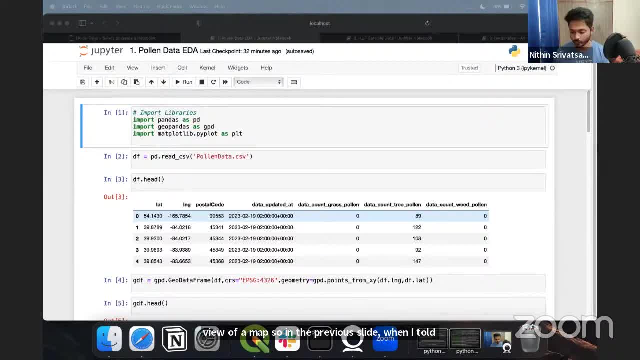 standard that's accepted, that's EPSG 4,, 3,, 2,, 6.. It's a name for the Coordinate Reference System. Okay, And next we have geometry, We have a longitude and we have a latitude, So now a GeoPanda's data frame. 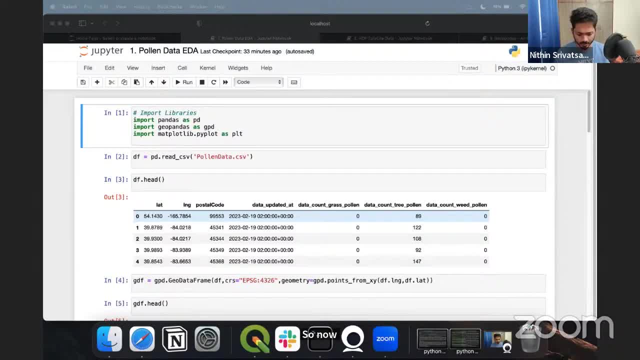 has been created. Let's just visualize how that looks like. It's pretty much Pandas data frame itself, except there is one column called geometry. This is the last column. Now, this is very important for a GeoPanda's library, because this geometry column is what tells us that the data 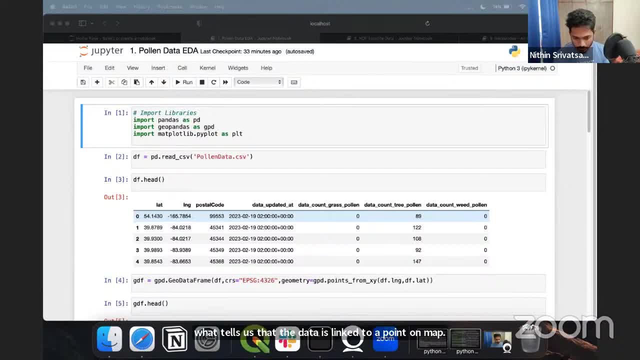 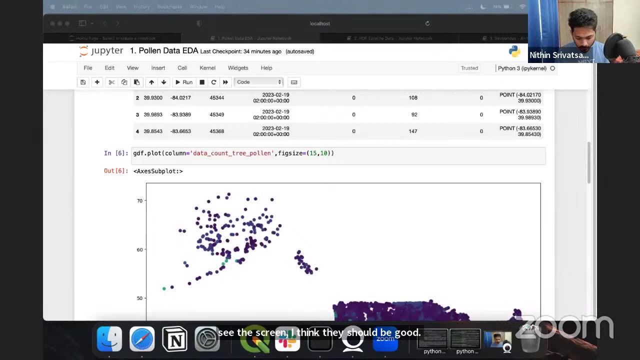 is linked to a point on map. Okay, So I'll just zoom in, just in case you're unable to see the screen. I think this should be good. Okay, Now let's just plot it. gpdplot. Let's plot the column. 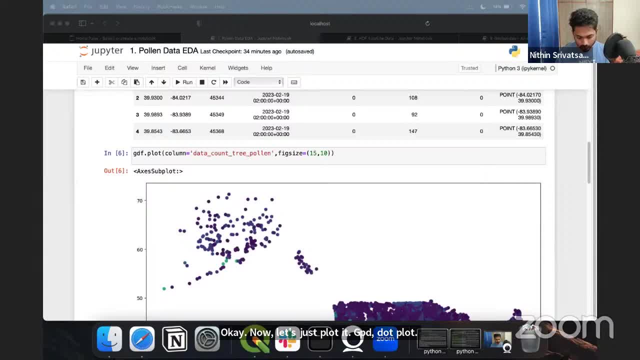 of tree pollen, because that has numbers in it And let's add a figure size, just so we can visualize that. Okay, So this is the pollen data which spans USA and Canada. So you see, geospatial data has a lat-long to it, identified by a column called geometry, and that is being plotted here. 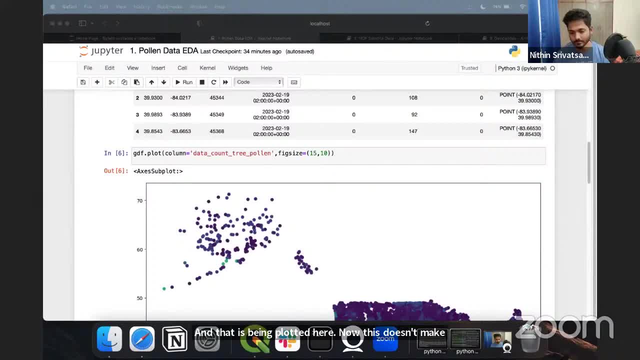 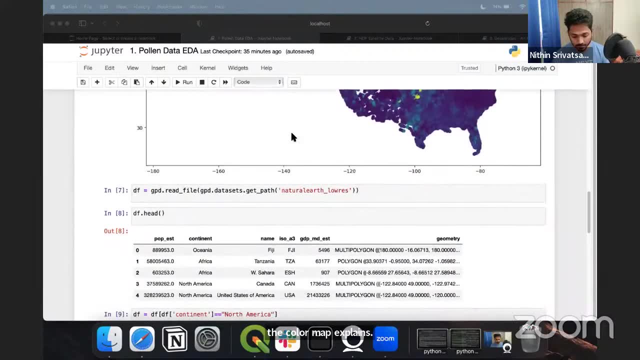 Now this doesn't make sense, right? I mean, I cannot see the boundaries, I cannot see what the color map explains, So let's add a few parameters to that as well. So to add a background map to this, we'll have to pull in another data. 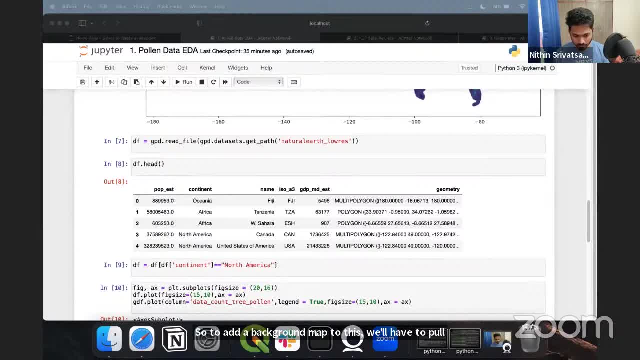 frame. So this is already available in GeoPandas: Read file similar to read CSV in Pandas, And we have a data set, Data sets, We get path from it And it's called natural earth Loris. Now let's see what this data frame actually contains. 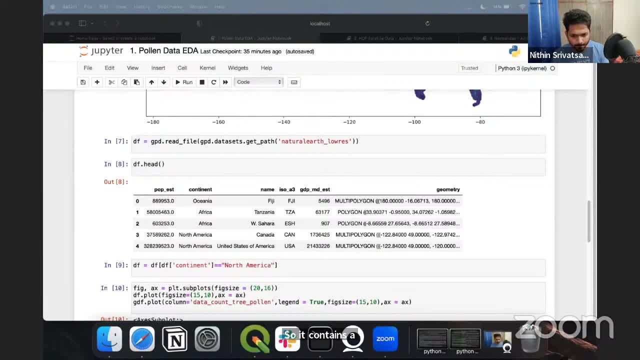 So it contains a continent here and the name for it And again the geometry, which is really important. Now you can see there's something Difference here. There's a polygon, There's a multipolygon, But our data frame had point. 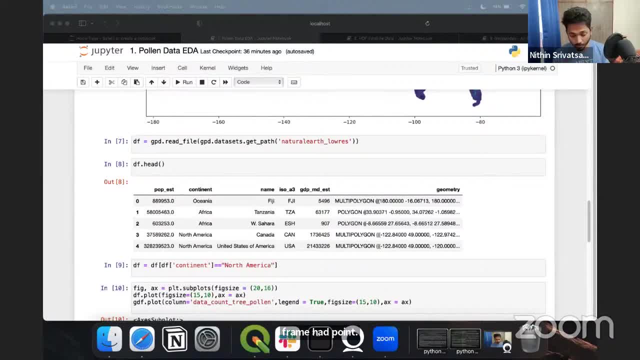 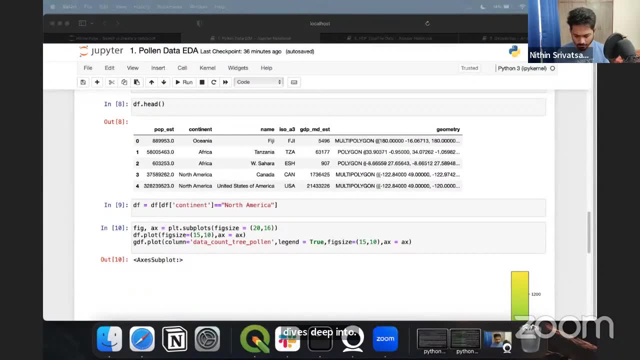 We'll be understanding that in a separate notebook which dives deep into what GeoPandas is all about. Okay, Now, once this is done, let's just filter it for our continent. So continent is equal to North America, Okay. 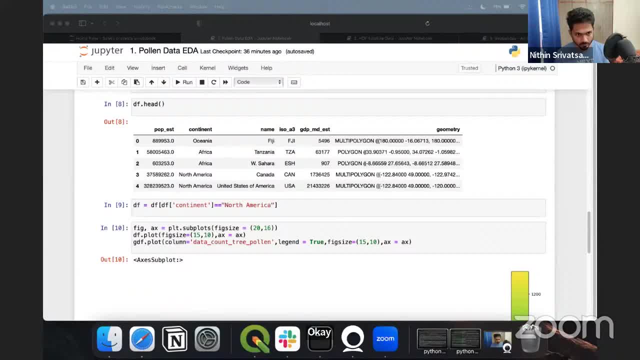 Okay, Now let's just plot it to see how it looks like. Okay, So this is map of the US, US, Canada. So now let's add this as the background for our image, so that we can see where Poland counts. 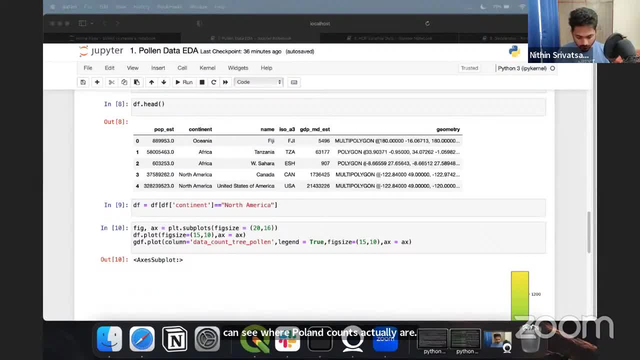 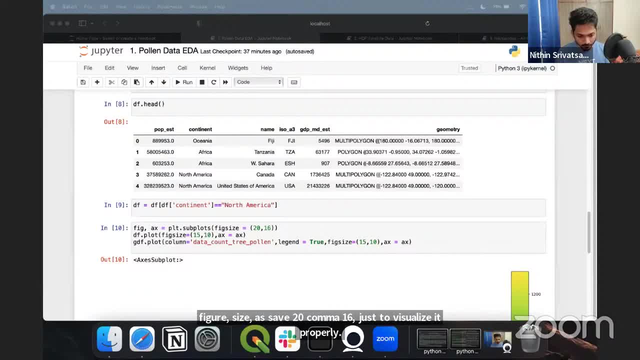 Now let's plot the world map, refer it to AX zone, And let's also plot our Geo data frame. Let's add legend equal to true, so that we understand what this scale is about, and a figure size again, and refer it to ax. so now, once we do that, 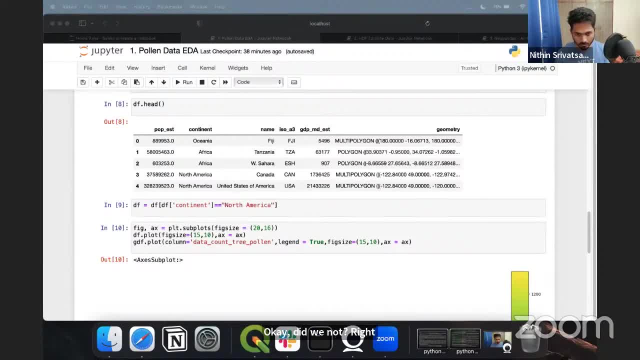 okay, did we not right? here we go rookie mistake right now. you can see the legend here and you have poland data that's mapped on the north america map. so now we get an idea of: okay, it's, it's high. uh, the counts are high here and it's pretty much low everywhere else. so this is. 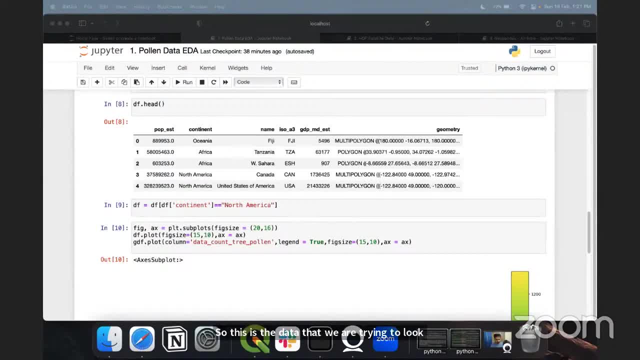 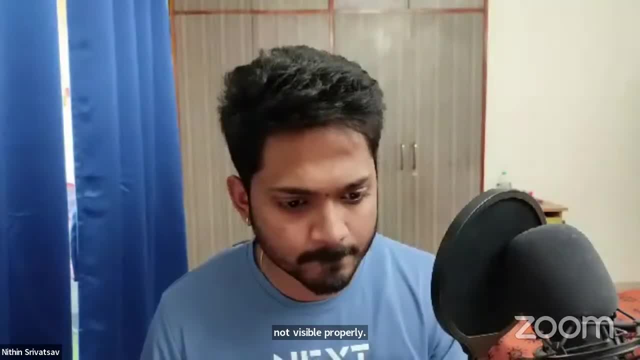 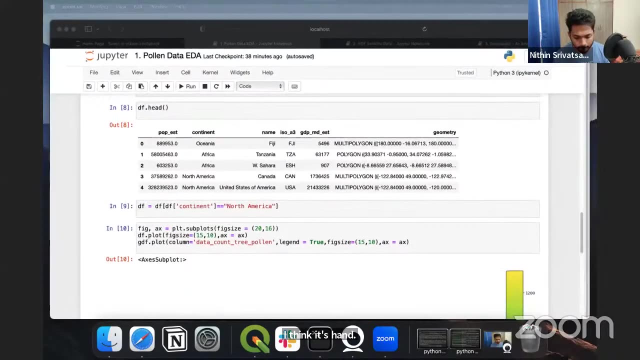 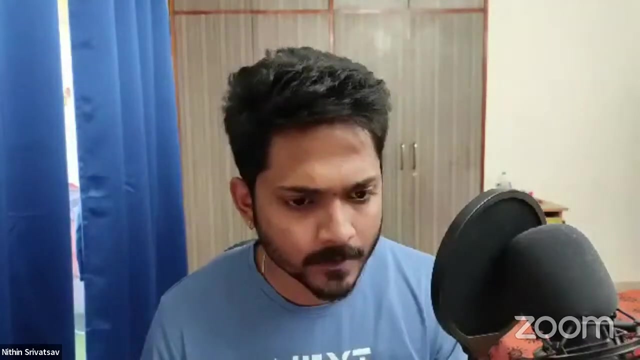 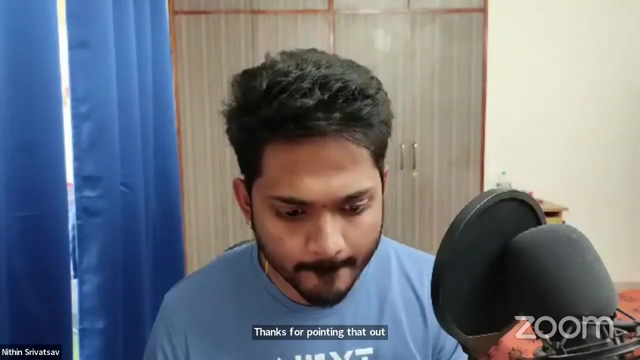 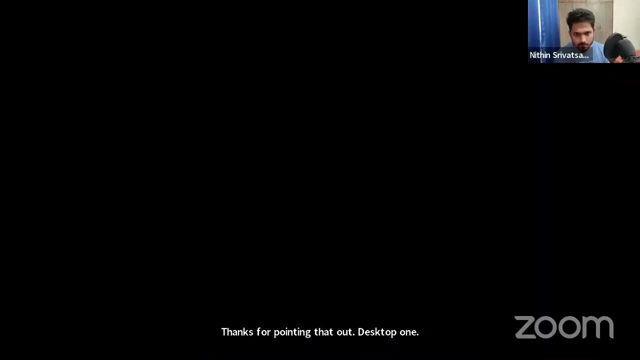 the data that we are trying to look. i'm sorry to interrupt you, but i think your screen is not visible properly. i think it's hanged, is it? let me just reshare just a second, okay. okay, Thanks for pointing that out. uh, desktop one. okay, is it visible now? 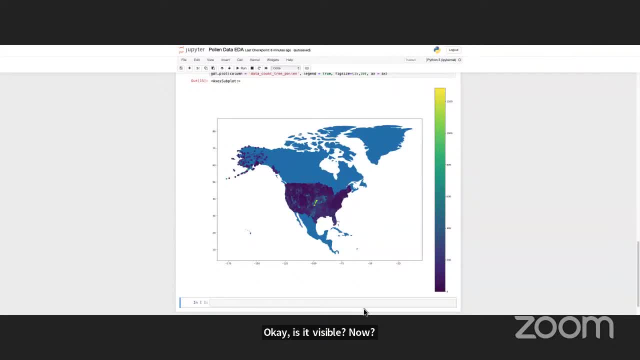 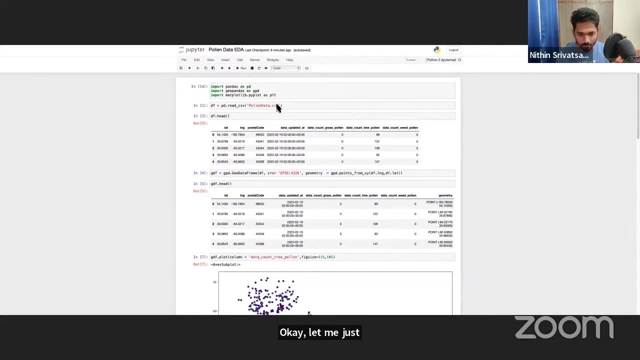 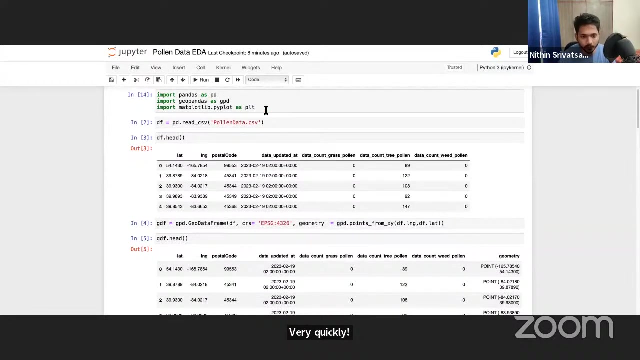 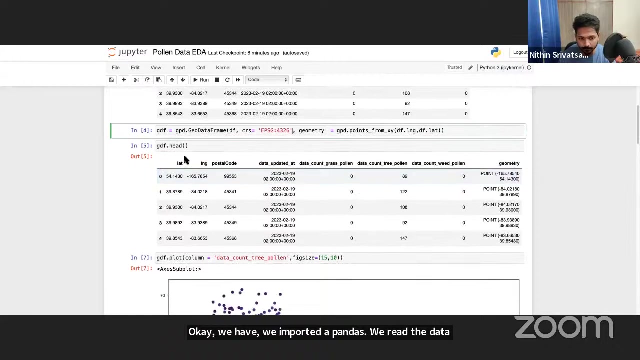 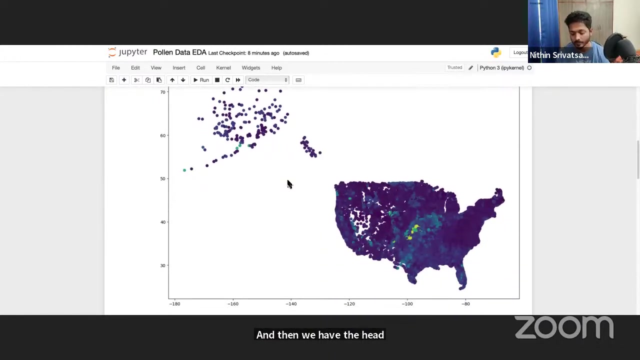 yes, yeah, okay, all right, okay, i was sharing the other screen. okay, sorry, okay, let me just uh rerun through the notebook again. uh, very quickly, okay, we have, we imported pandas, we read the data set and, uh, we created a geopandas data frame and then we have the head. uh, then we just plotted it on the map without 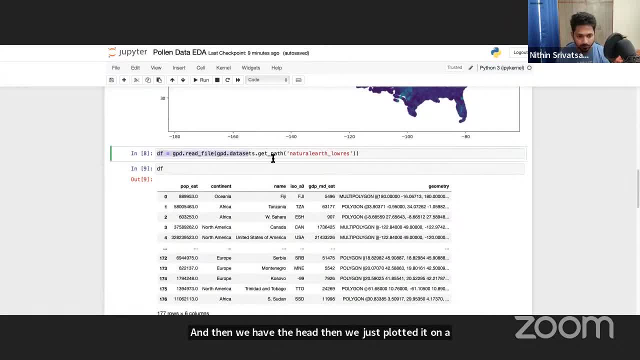 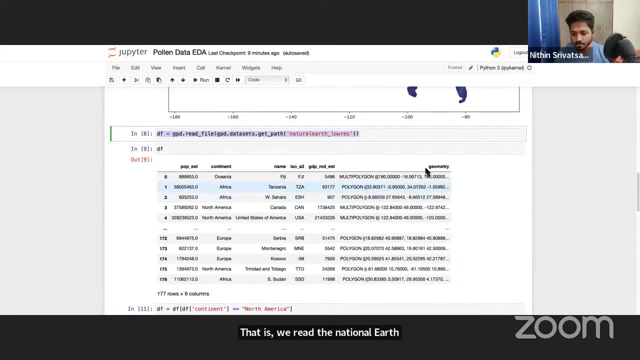 anything. and then we came forward. there is, uh, we read, the natural earth loris, which is a geopandas data set, inbuilt data set. so this is what i was mentioning. the geometry is that's what is most important for uh, geopandas data frame to understand what it is. so you have multiple 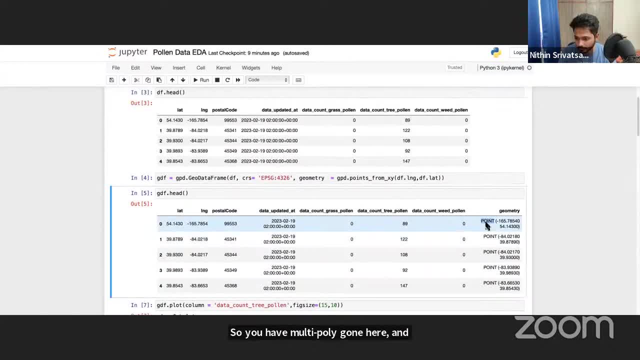 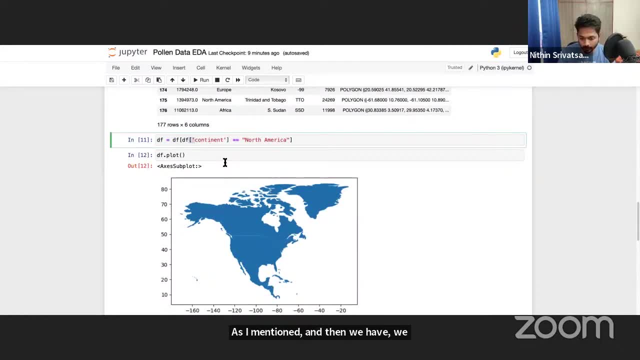 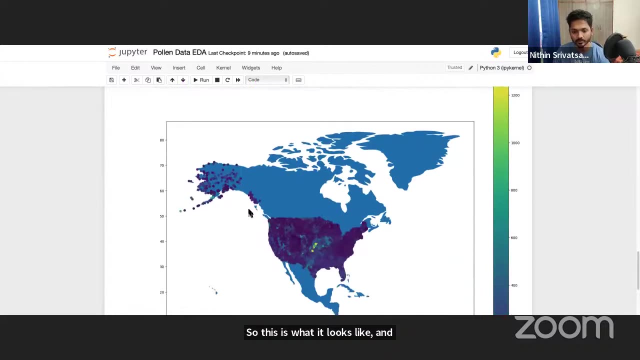 polygons here and you have poly point here now, which will be deep diving again, as i mentioned, and then we have- we took- the continent of north america, so this is what it looks like, and then we uh map those both to plot it like this: so we have poland data on top of the us. 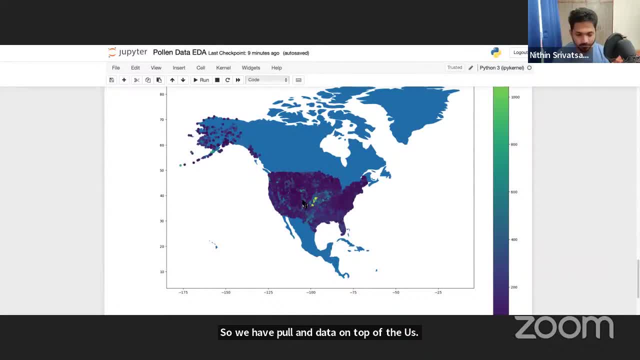 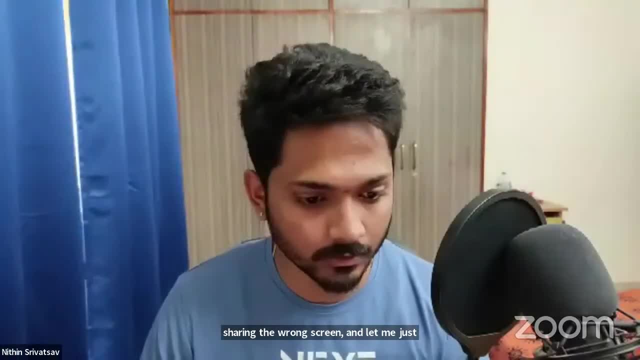 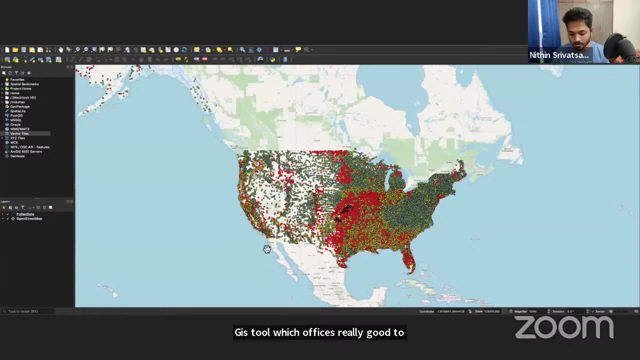 continent. so this is what we did in the notebook. please excuse me for sharing the wrong screen- and, uh, let me just share now the qgis tool, which offers a really good way to interact. now i'm sure the screen is visible. i think it is. so whatever we saw on that map is here in qgstool i. 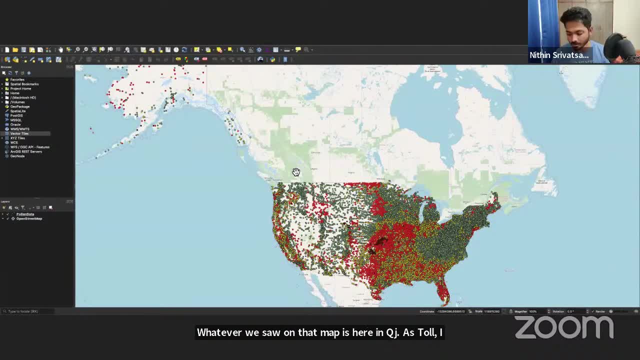 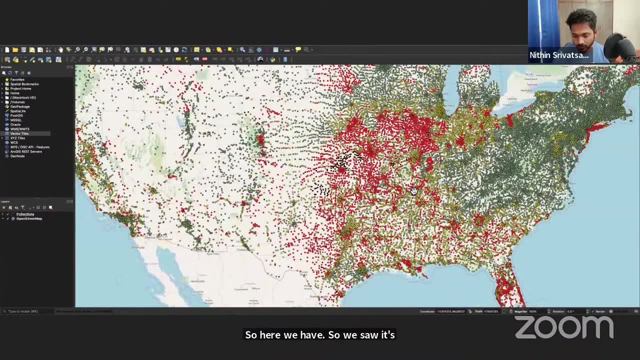 will not be deep diving into how qgis works because it's a little complex and will require a session on its own. so here we have. so we saw it. it's high here, so so you can play around with qgs like this. so there's a tool that exists. 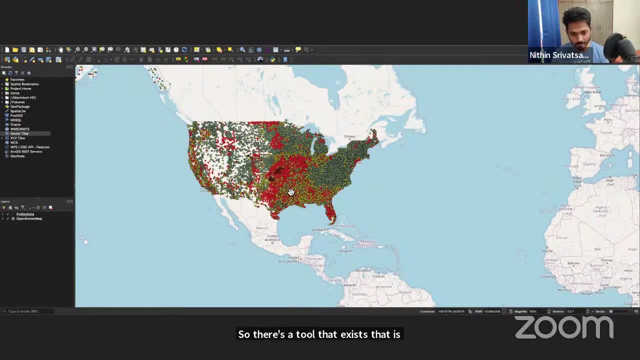 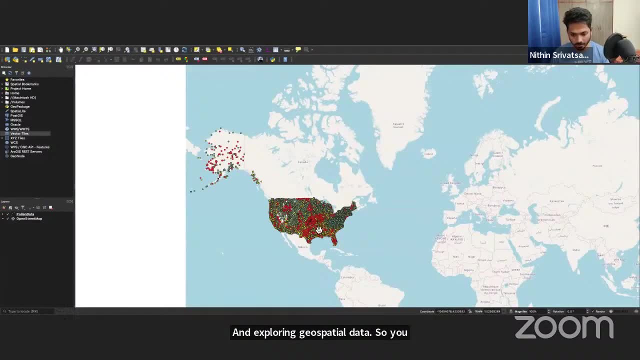 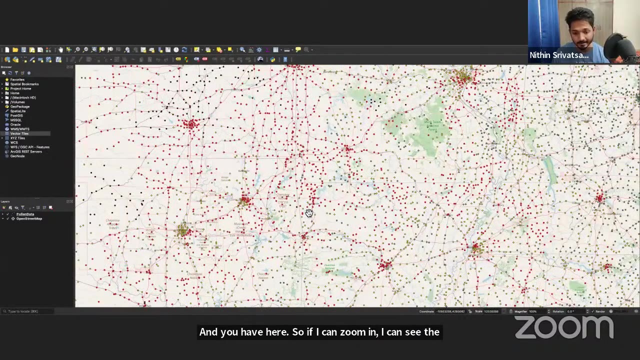 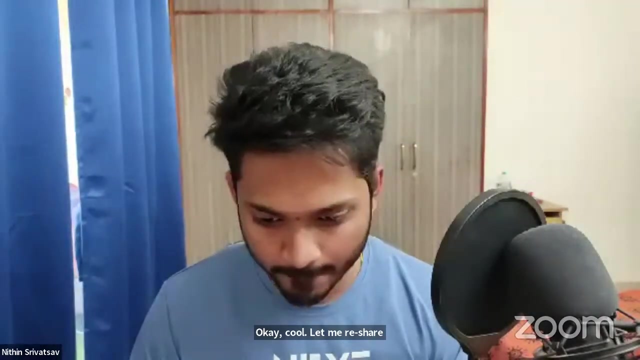 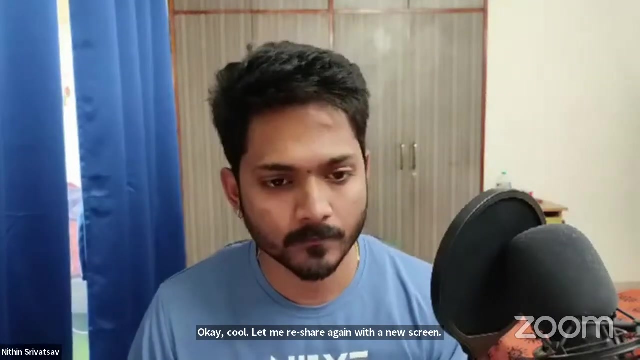 that is specifically built for visualization and, uh, exploring geospatial data. so you have data here, canada, and you have here. so if i can zoom in, i can see the individual points, the points that were present in the map. okay, cool. uh, let me re-share again with a new screen. 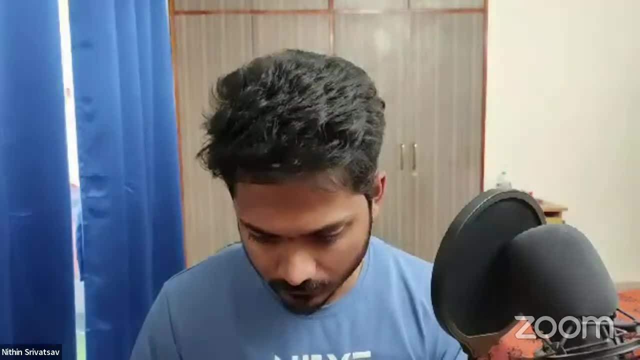 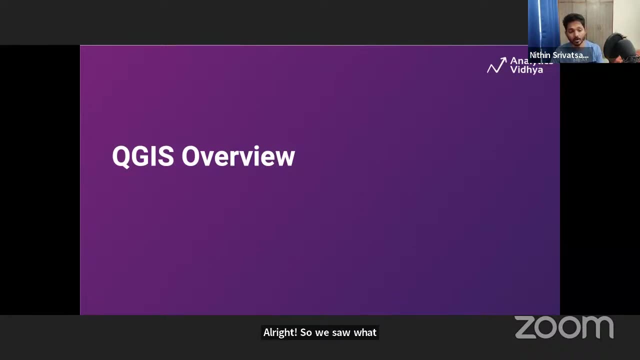 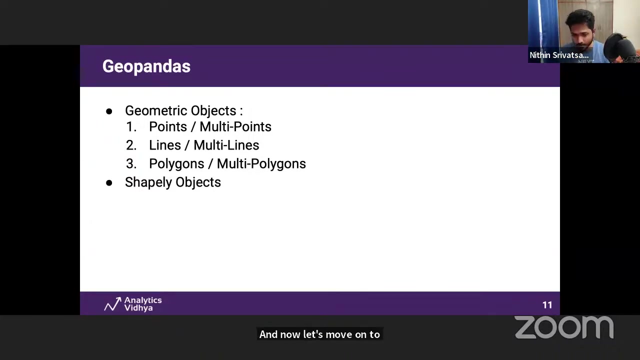 all right. so we saw what the data set was about and what qgs is, and now let's move on to geoparlers. so geop sodars is the go-to library for geospatial data. there are a lot of geometric objects in that. 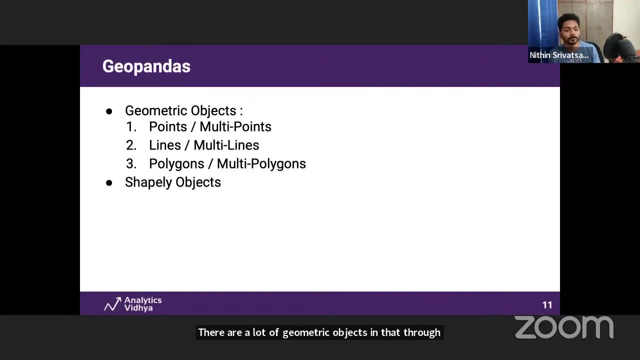 through which we can play around. and, uh, there are points, there's lines, uh, and clicking on the, And there are polygons and shapely objects as well. Okay, any questions? so far? Okay, none, Cool, Okay, so now let's deep dive into GeoPanda's library. 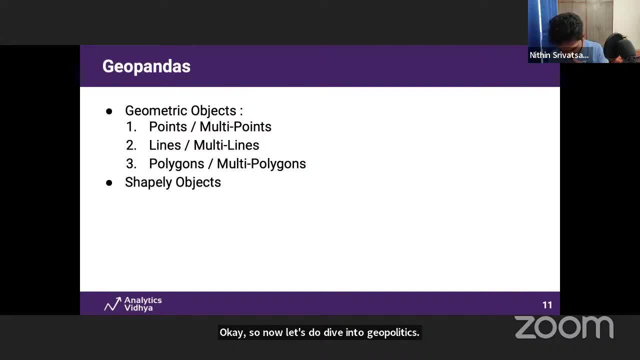 Now, actually before that, just realizing. so there are a lot of satellite data formats, right? So let's just look at one example of a HDF file on how that works And let's just explore the library and just read a data frame and see what exactly our HDF files are about. 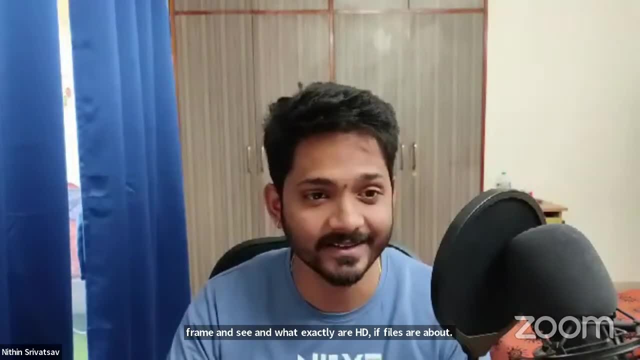 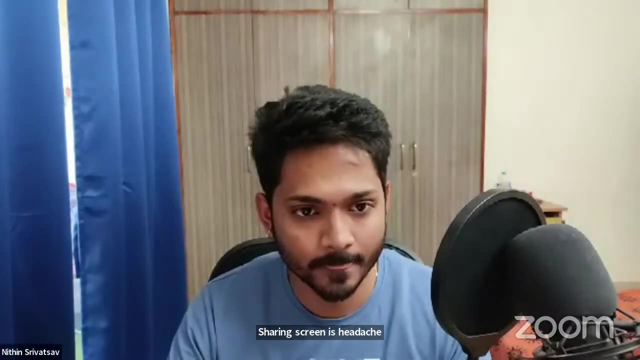 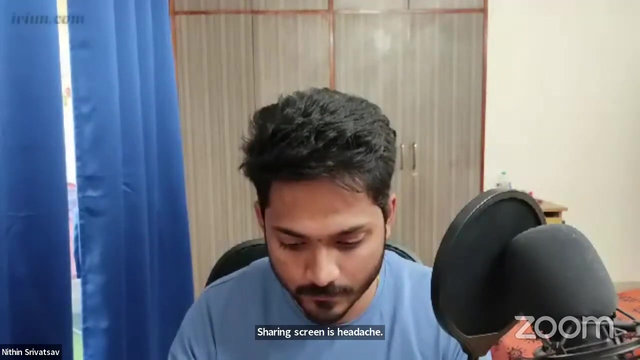 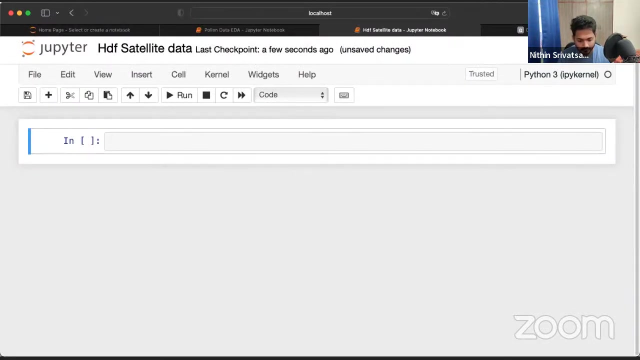 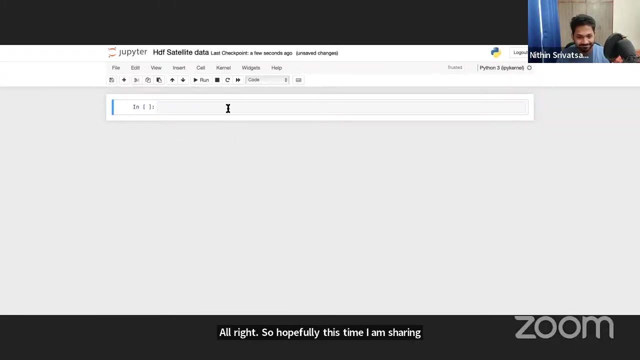 Sharing screen is a headache, All right, so hopefully this time I am sharing the app. Okay, cool, So let's just import Pandas SPD. Now, in order to access the HDF file, we'll need a specific library, which is called PyHDF. 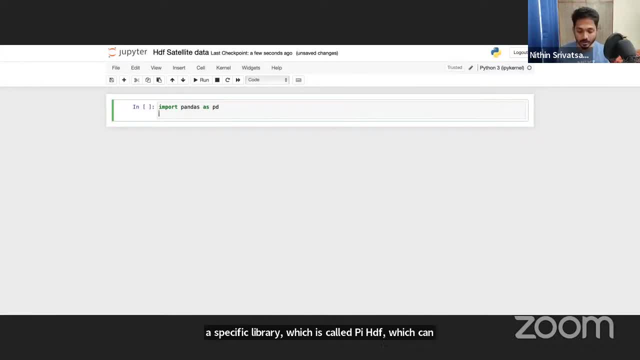 which can be installed using install PyHDF or Conda, install minus C, Conda 4, PyHDF. So let's just import that PyHDFsd, Import sd and sdc, So you needn't worry about all the terminologies. 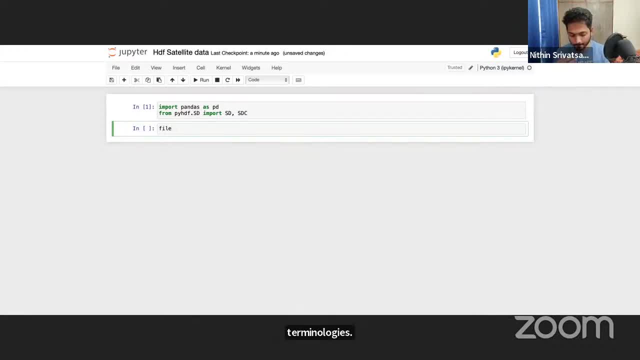 It's okay to understand that these are the libraries that are required to read specific formats. Okay St, and we have dot. We have a file which is a file from NASA, which is the MODIS file, which contains water vapor data in it. 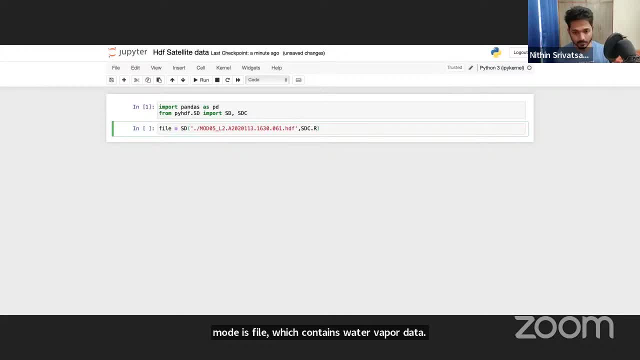 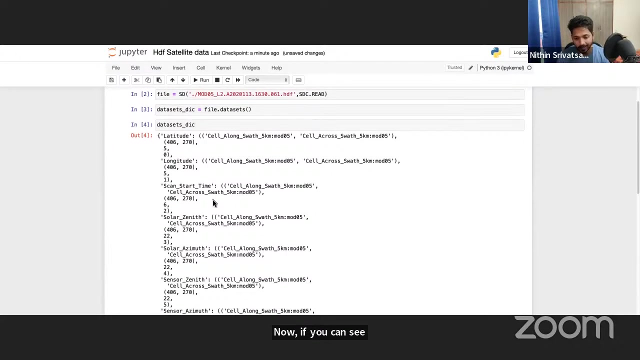 So we pass sdcread. So now we've had the file contents and we can see the parameters that are present inside that as data. And, if you can see, This HDF file contains latitude longitude, again important for geospatial data. 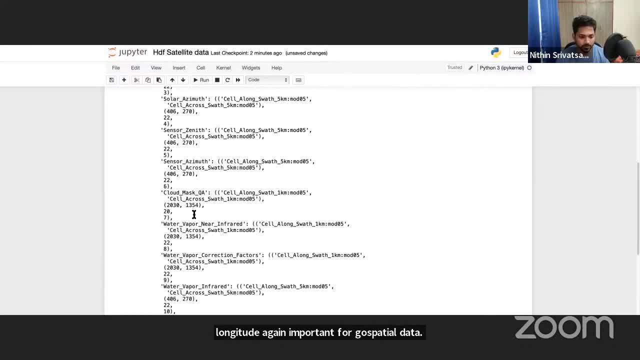 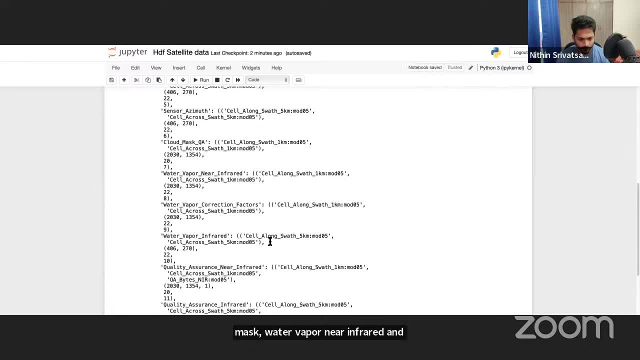 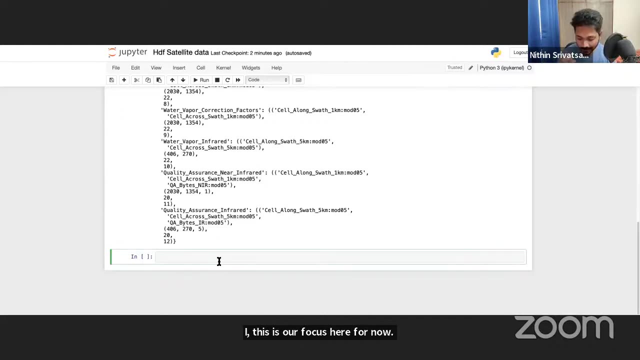 This can start start time. a couple of sensor values, cloud mask, water vapor, near infrared and stuff. uh, i i. this is our focus here for now. uh, so right, let's, let's select these columns, the columns that we need. so we need the latitude, we need the longitude and we need the water vapor data. so 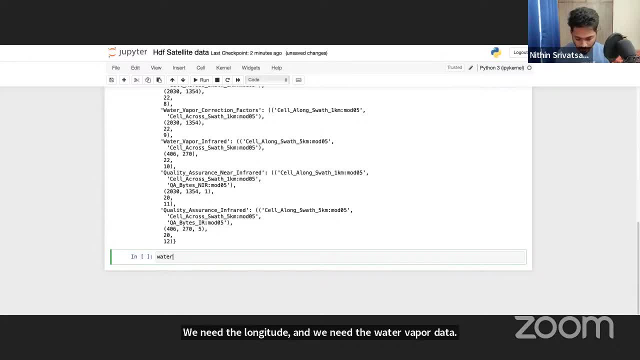 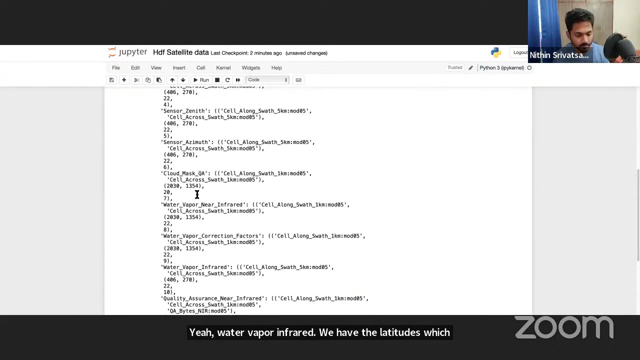 let's select that. uh, i'll just type in quickly: so we need water vapor. we select it from the file file dot select. yeah, water vapor infrared. we have the latitudes which are in the latitude column, so again. so these are the data dictionary, these are the columns that are present. 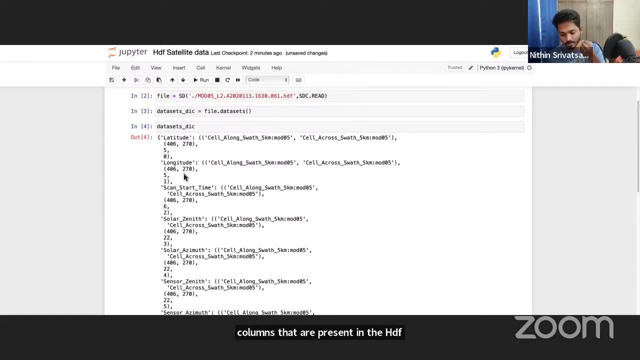 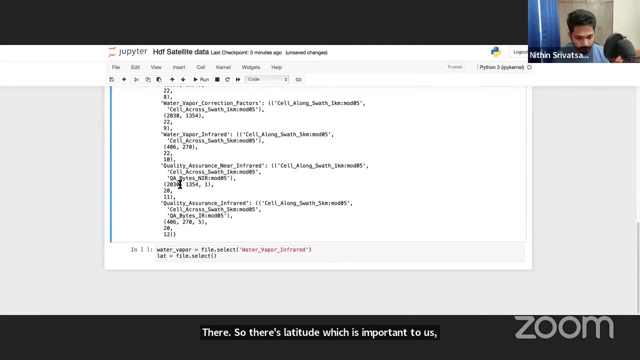 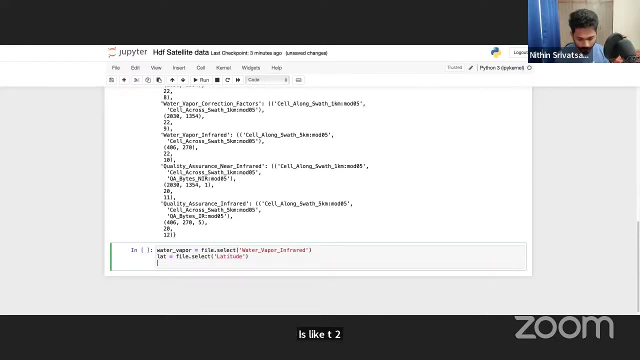 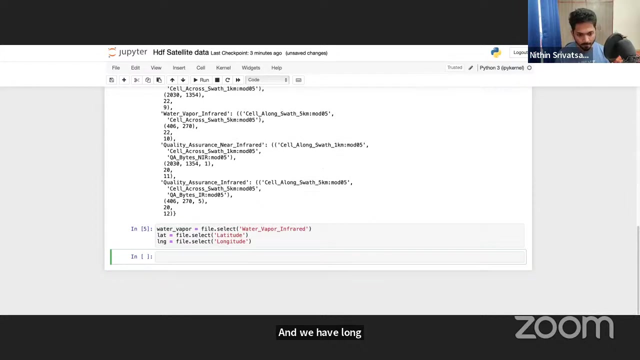 in the hdf file and we'll be taking these from the hdl file and creating a pandas data frame there. so there's latitude, which is important to us, and longitude, so let's take that. there's latitude and we have long, which is okay. now here is where things get interesting. 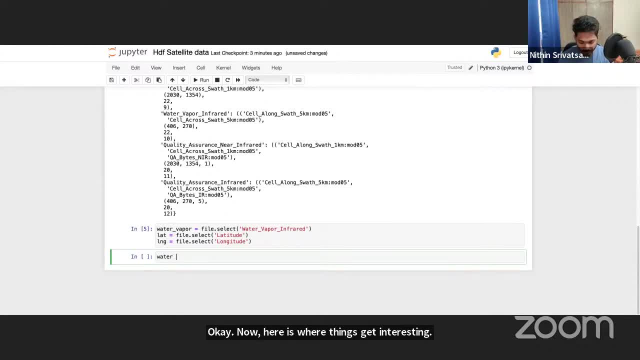 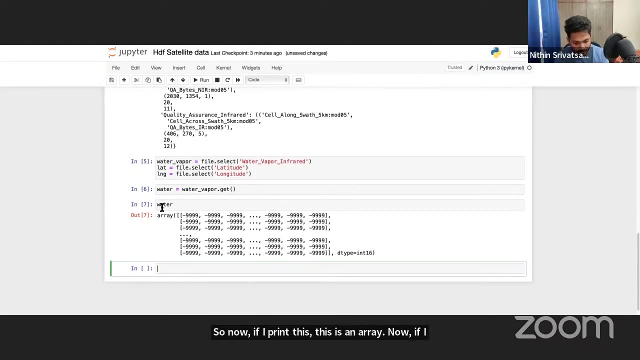 let's just first take uh, the data from the selected fields, and you'll understand where things get interesting. so now, if i print this, this is an array. now, if i just convert this into a data frame, you'll see how it is mapped to the entire world and the format of uh hd. so last data frame: 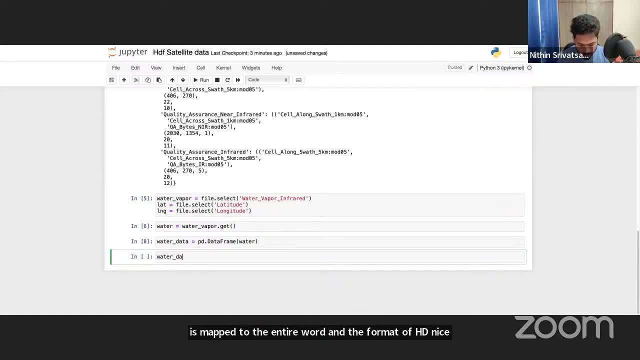 now, alright, let's say w way i'm like, and then this is that which i have, exactly which i want. but i did not want to copy because when it's uer that becomes crap. let's see if i can do a, but i will complete, correct all the data. 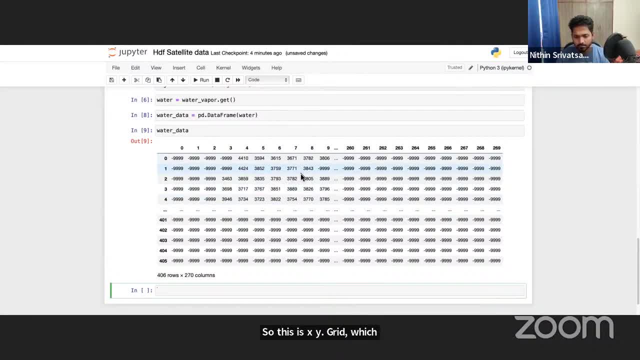 and now if i see water, now if i see water data. so this is a x comma y grid which contains only values at a specific place, but rest, every of that is minus 999, meaning invalid value. now, this explains us that the data that we got from the 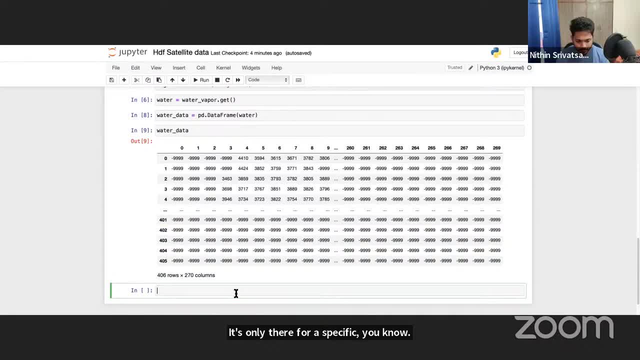 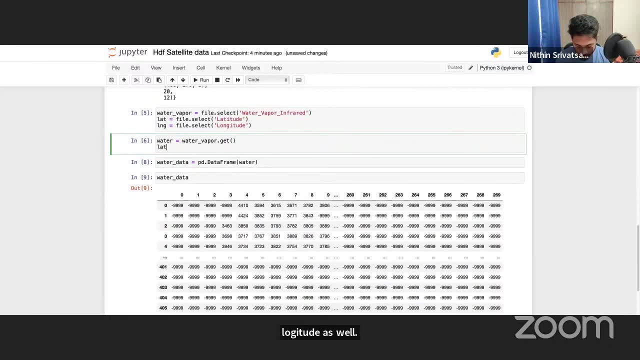 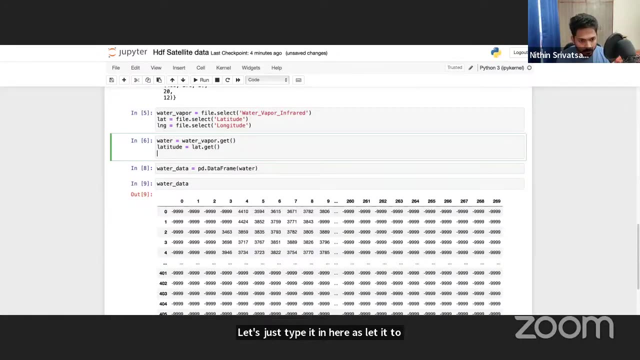 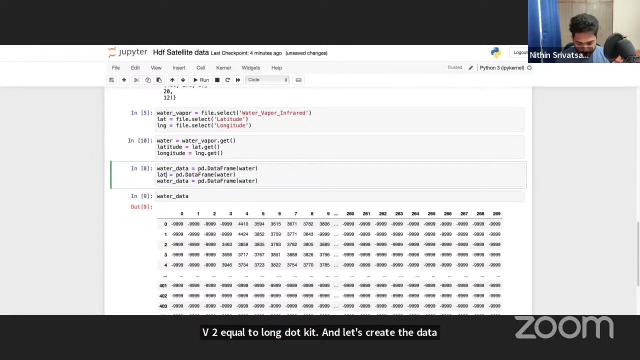 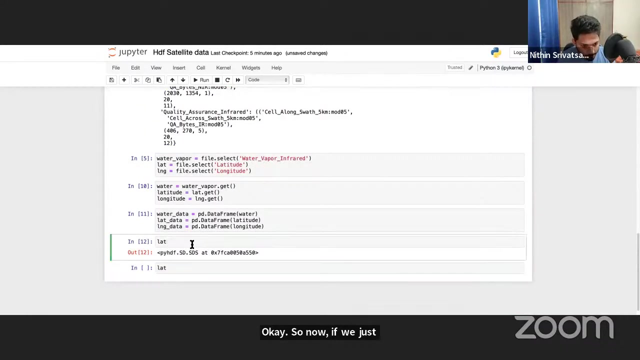 region. So what we do is now: let's just take the latitude and longitude as well. Let's just type it in here: is latitude equal to long, dot get, and let's create the data frames respectively: Okay, so now, if we just visualize the lat long, 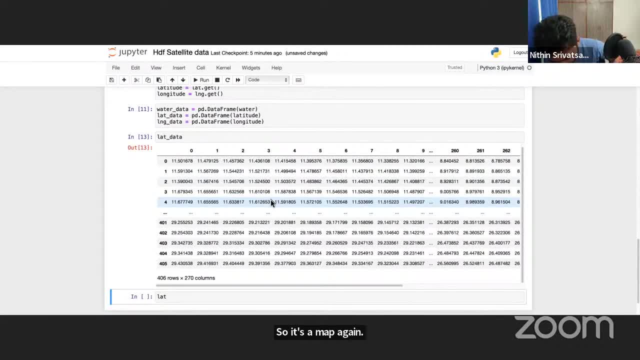 So it's a map again. so what's happening in the backend, in a hdf file is, uh say, for example: so there's one layer now this contains all the latitudes, and on the, all the latitudes of the world, and then there is longitude file. so there are two files now: latitude, which contains all the latitudes of. 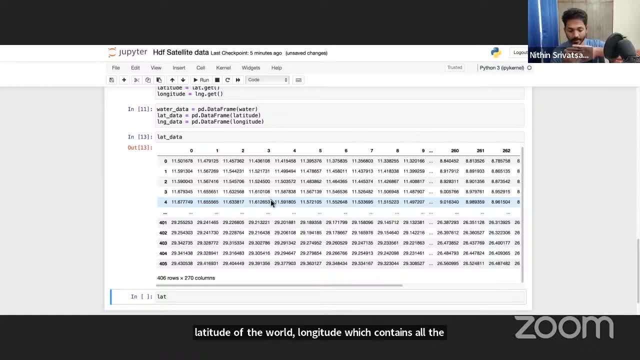 the world longitude, which contains all the values of the world, and then we have water vapor data, which we took. that contains for all the individual mappings. now, when we merge all these three together, all these three files merged together, is how hdf is stored in the backend. so it's not 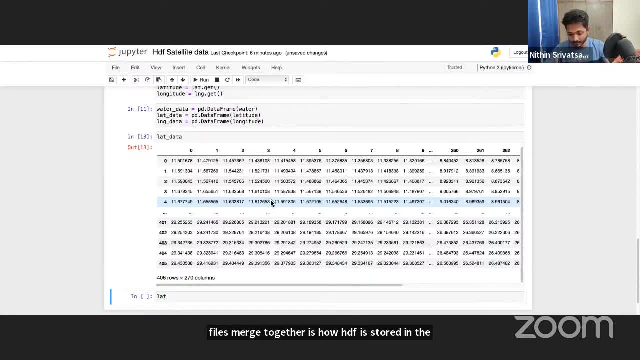 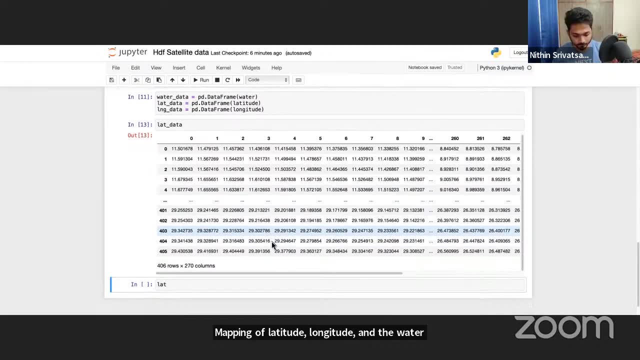 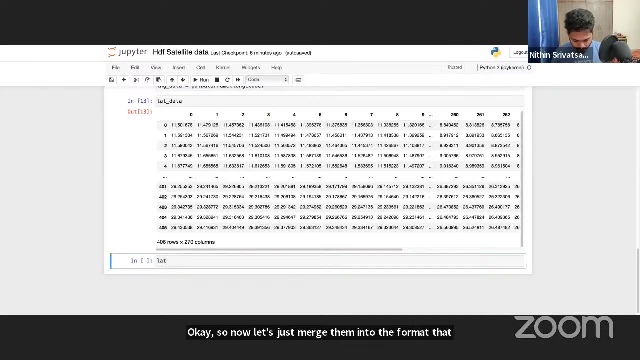 like your traditional lat long and then water vapor, but rather it's a 3d mapping of latitude, longitude and the water vapor data. okay, so now let's just merge them into the format that we want. uh, it's a pretty long code, so i'll just copy paste it here, instead of wasting time typing. 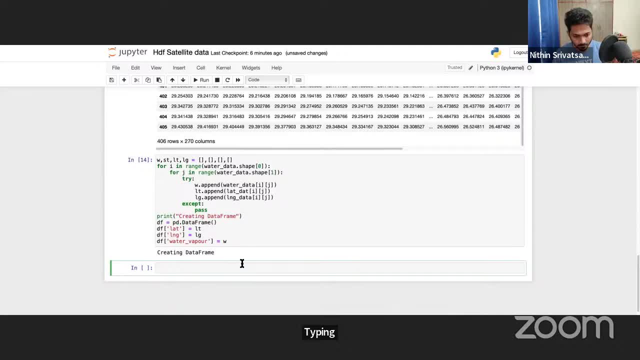 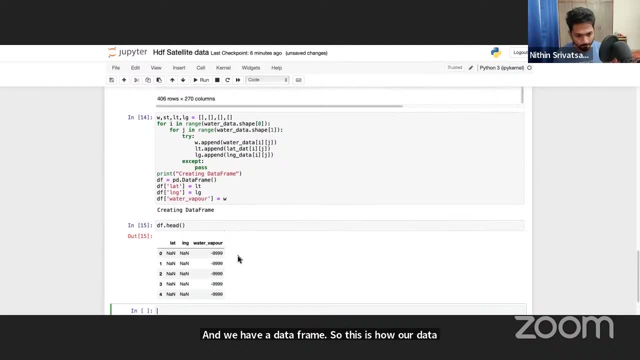 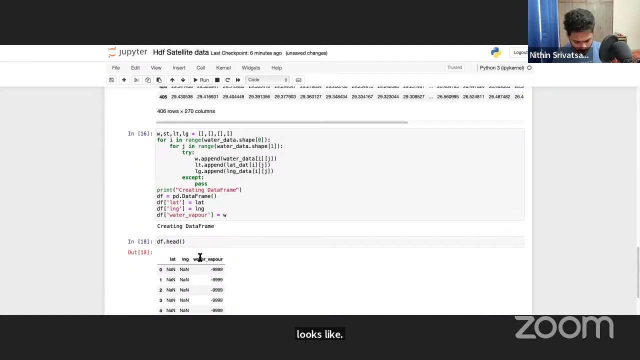 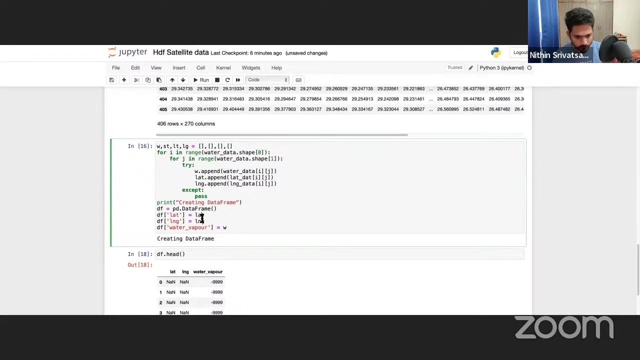 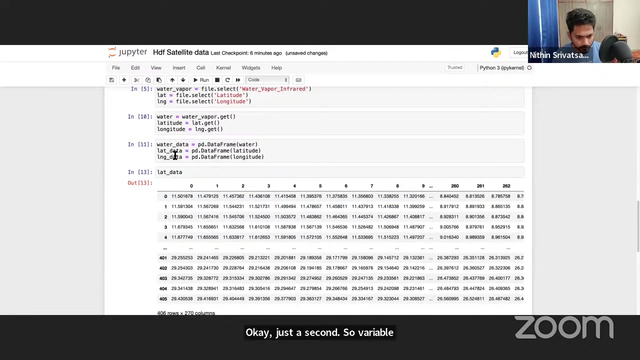 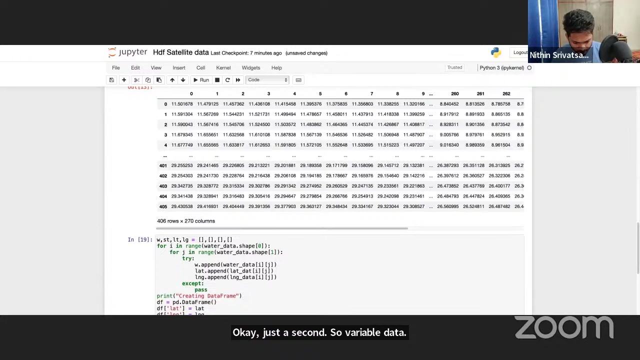 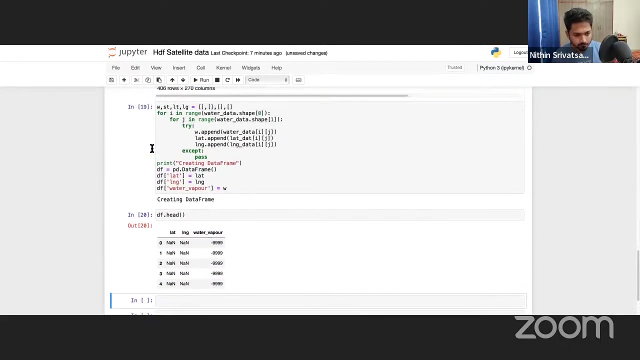 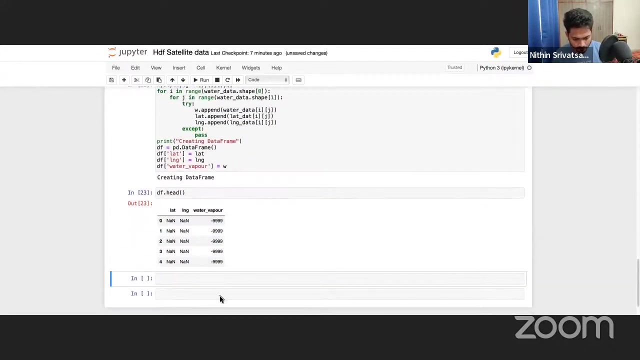 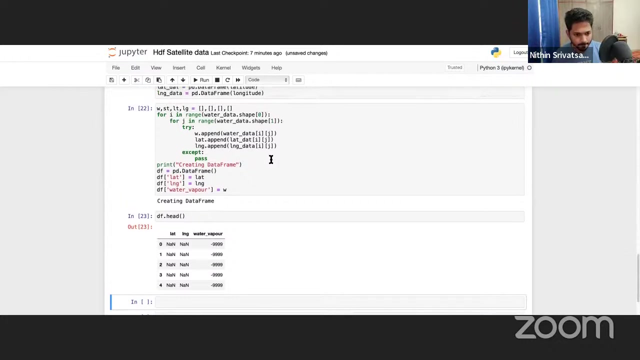 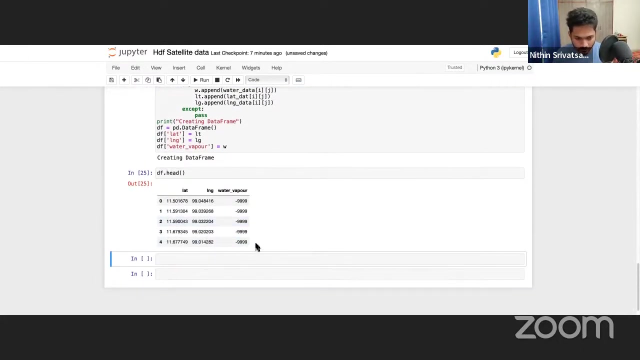 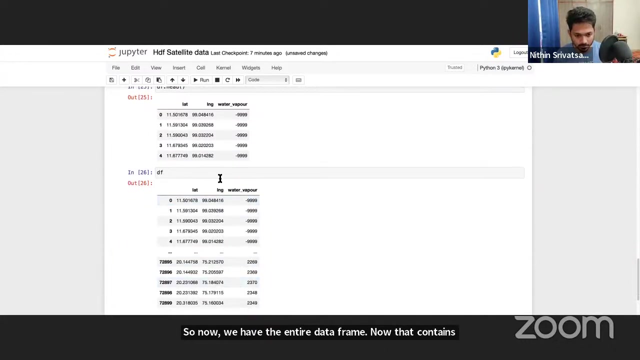 and we have a data frame. so this is how our data frame looks like. okay, just a second. some variable data. okay, here we go. some variable change issue, right? so now we have the entire data frame. now that contains minus 999 values, so let's just remove the values that are not. 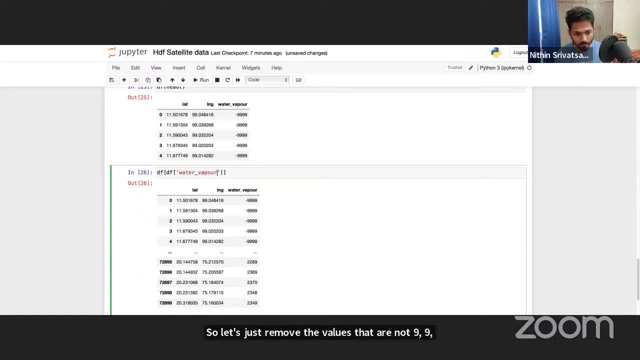 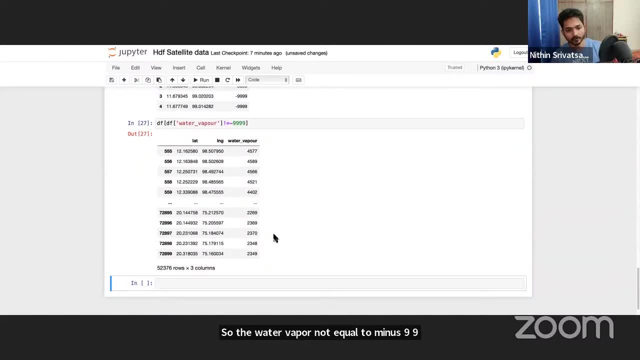 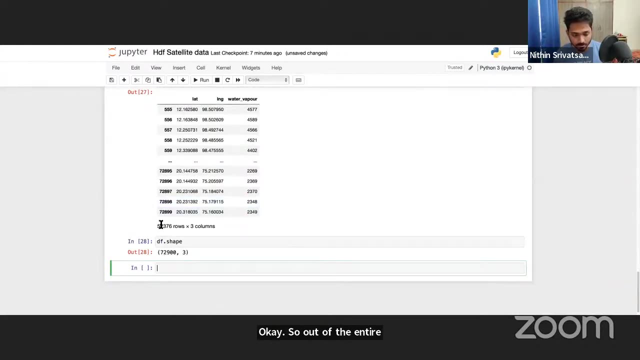 999, so the water vapor not equal to minus 9999. okay, so out of the one-Art Native, ok, oh, too heavy. uh, 72 000 locations, only 52 000 locations had actual valid lat long value or water vapor value, and let's just save it to a csv: water vapor dot csv. so this is how we took the data from the Maeve file distribution. okay, so after we merge the entire system. okay, so out of the entire uh 72 000 locations, only 52 000 locations had actual valid lat long value. that's doing something positive. two rows at one, Например Next. so now we have data, will that comes out? 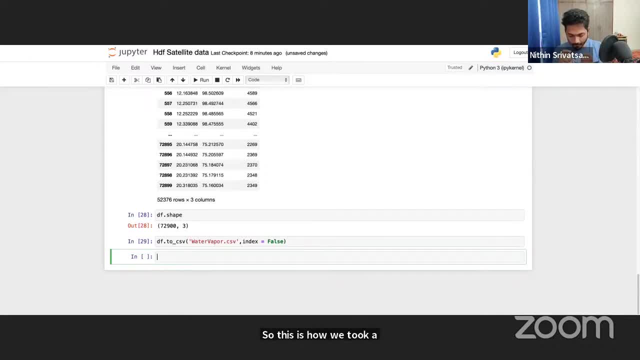 satellite data to call the parameters that we need and then convert it into a data frame that's understandable to us. so this, this is an example of hdf. there are other libraries and other files that are, you know, netcdf, or there are grip files, geotiff files, and each has a python. 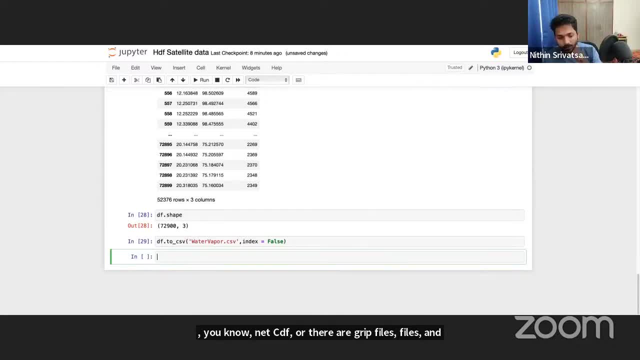 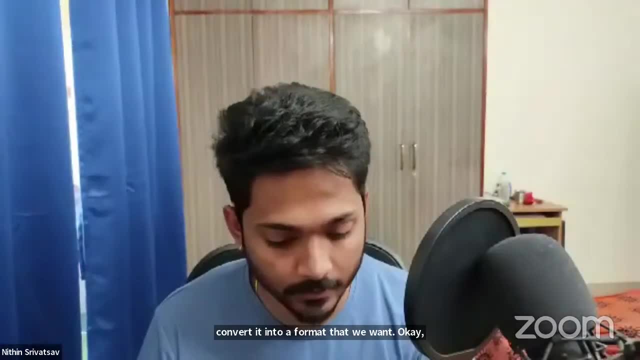 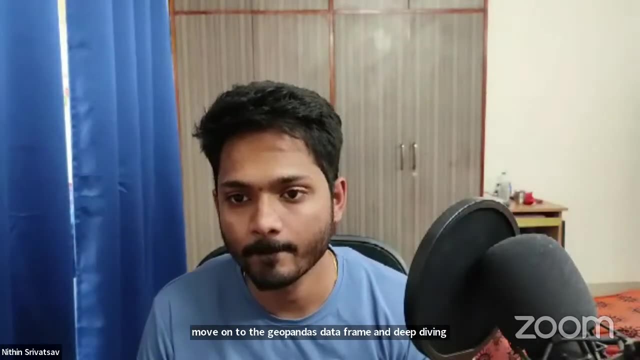 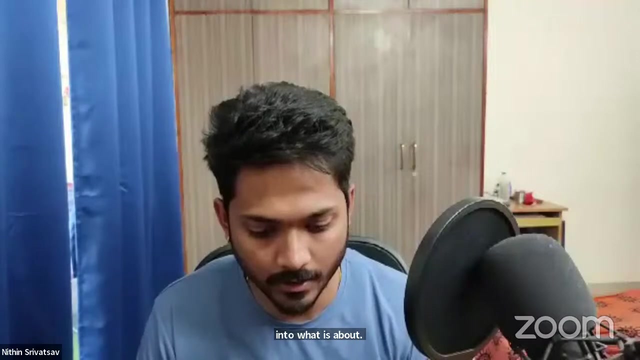 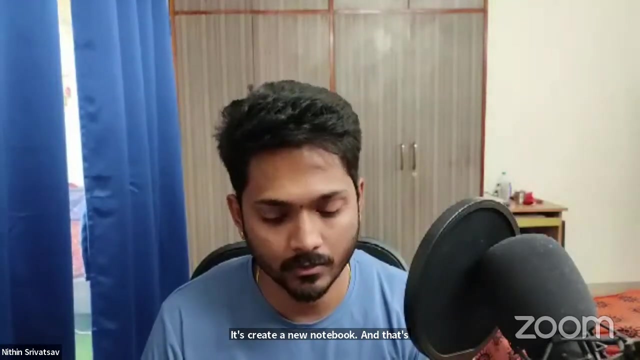 library which we can use to take data and convert it into a format that we want. okay, now let's move on to the geopandas data frame and deep diving into what geopandas is about. let's create a new notebook and that's geopandas intro. okay, sharing the screen again. 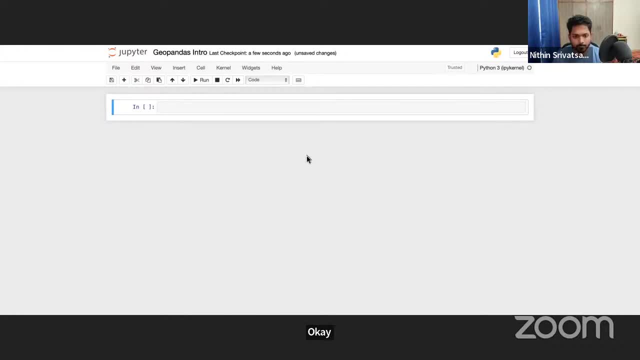 okay, right. sarang is asking: you know there's one hdf file, and what if we have data for multiple years so you'll have to process the file individually? now there are advanced methods on how you can do this in parallel. you know there are glue jobs in aws where it runs through the entire hdf files and 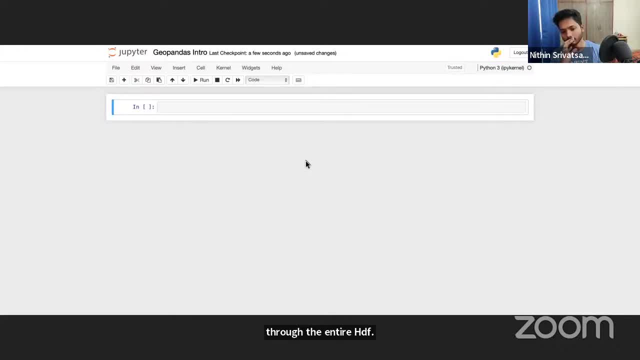 then converts it into a single file. so this is a single data frame. so but to in order to process, you will have to do it one file and one by one. okay, i'll just you know answer some of the questions here. so i use tablou. can we use it? 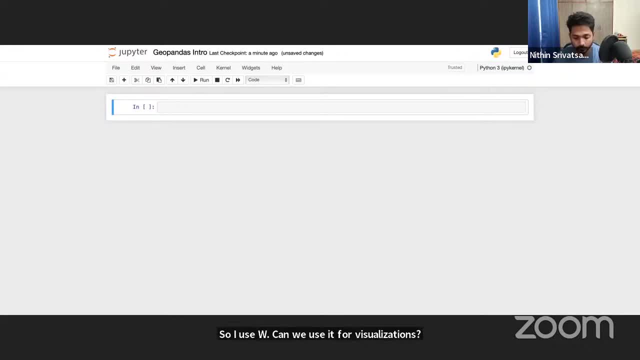 for visualizations? yes, we can uh. again, i'm not really much well versed with tablo but there is an option to visualize qgis. i mean a, j, special data in tableau and uh. abdul is asking: where can we get geospatial data set right? so geospatial data sets is anywhere. 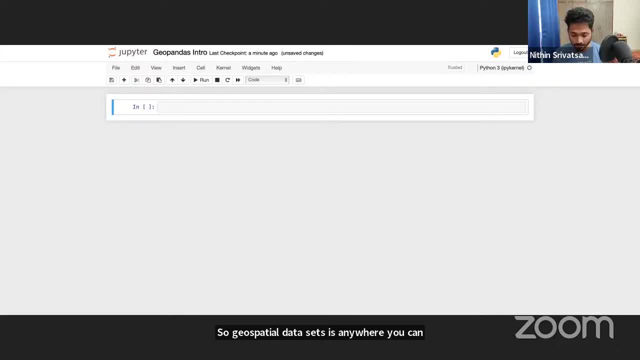 you can find it in ambi and any weather data provider. so everything is there in ambi, actually, and there are some kaggle open source data sets available for- uh, you know, uber data sets or swiggy orders, zomato orders, so anything that has latitude and longitude to it that can be considered as. 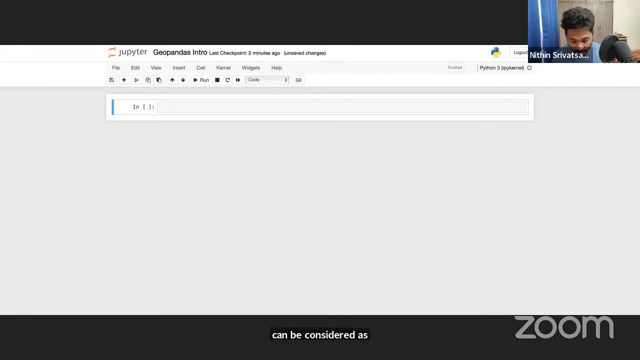 geospatial data. yes, i can recommend a textbook. i have a couple of links which i will be sharing at the end of this presentation. i will also add it to my github profile that you can check in. all right, let's uh move into geopandas intro. so what this? 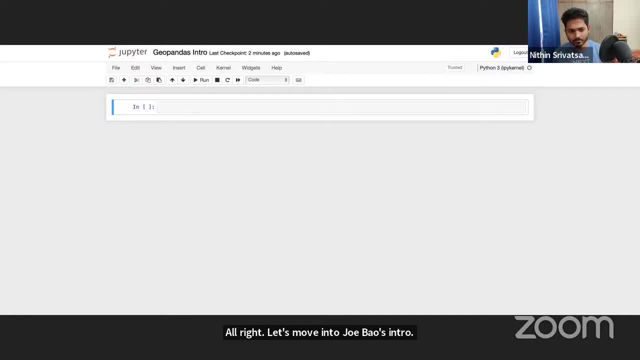 says session is being aimed at is not deep diving into geospatial data or, you know, getting into depth and messing with our minds, but rather an overview or a kind of information for you like. all right, there is geospatial data and there is geospatial data science. if i ever come across any sort of 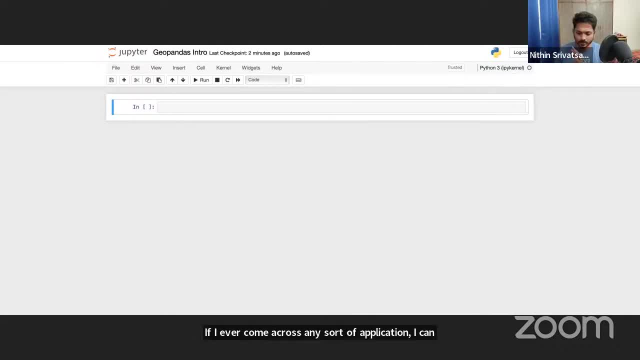 application. i can utilize this and you know, okay, these are the libraries that i need. so this is the sort of information that i'm trying to convey in this session. if you want, we can deep dive into geospatial data science in subsequent sessions, or even deep dive into qgis, which is an excellent tool. 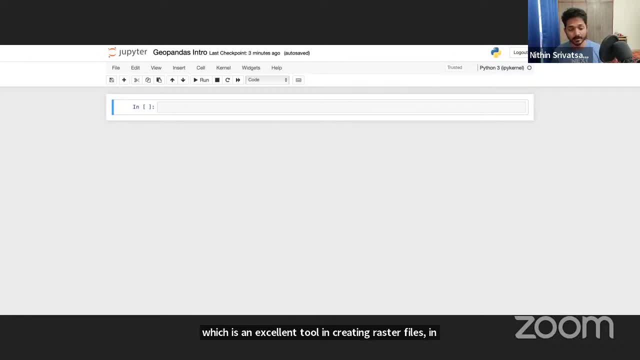 in creating raster files, in creating tiff files and more to do with satellite data and pure raw geospatial data. that's where qgis is used. so let me know in chat and comments on if you want that session or not. okay, let's just dive into now the 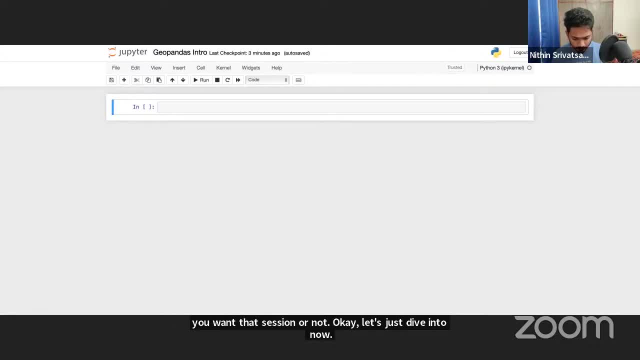 geopandas. so first let's import our necessary libraries, or you know? let me just copy paste. you know, i think we're wasting too much time. we can discuss better things. okay, right, so we imported pandas, which is a well-versed library. there's geopandas, there's shapely geometry. 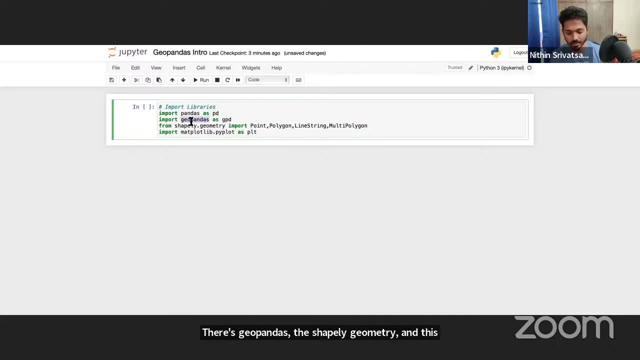 and this maplib, now geopandas, is something that you just came in touch with and, shapely again, is kind of a base layer on top of which geopandas works. so there is shapely geometry. so we'll understand what a point is, what a polygon is, what a line string is and what a multi polygon is. 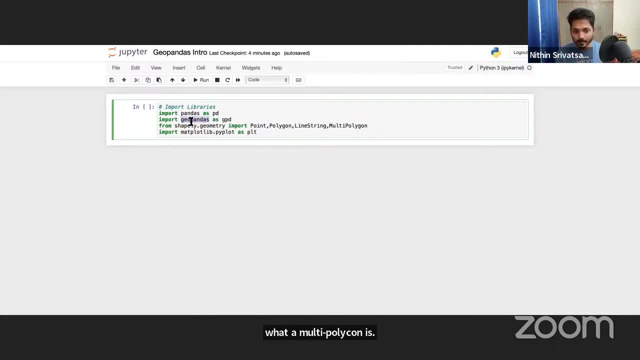 so these make up the back end of geopandas. so we imported pandas, which is a well-versed library, pandas and your filterings and functions that you can use. so we'll be exploring that one by one. so you know, in pandas there are two types of data types, right? one is the pandas data frame. 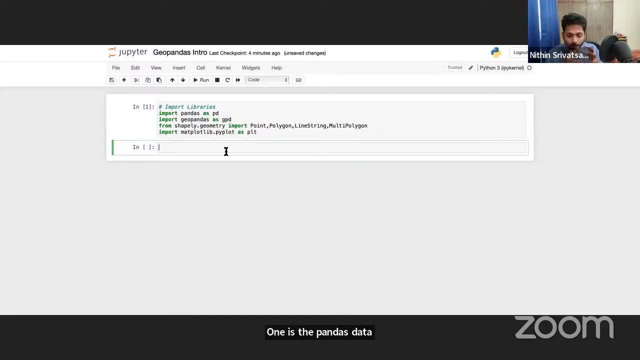 and the other one is panda series. so panda series make up the pandas data frame. similarly, in geo pandas there is geo data frame and geo data series. so same convention, same working, just it's different. works with pandas, works with geo frame. so now let's explore what point is. 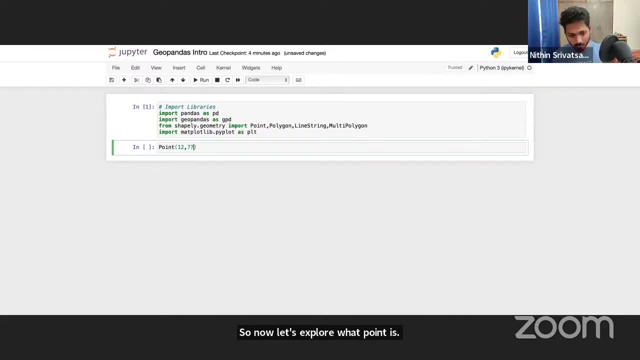 so point is a single latitude and longitude that you can plot on a map. now, if i execute the cell, it's a single point, 12 comma 77. now you cannot see where it's located because we still we haven't added the coordinate reference system or the map on top of which we can paste this. but so point is: 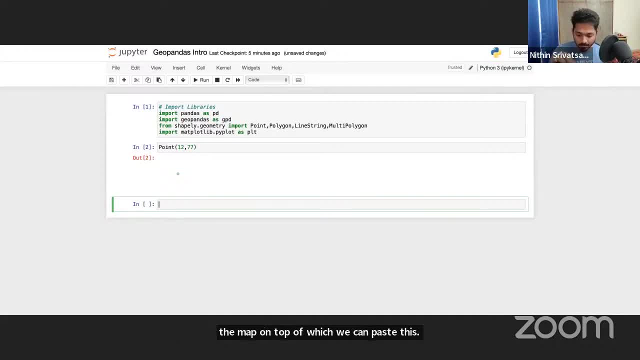 a single latitude and longitude that you can identify on a map. now, line string is a collection of points that you can draw a line on in the map. okay, so let's just create a line string which contains an array of values, so 0 comma 0, and then let's say we have 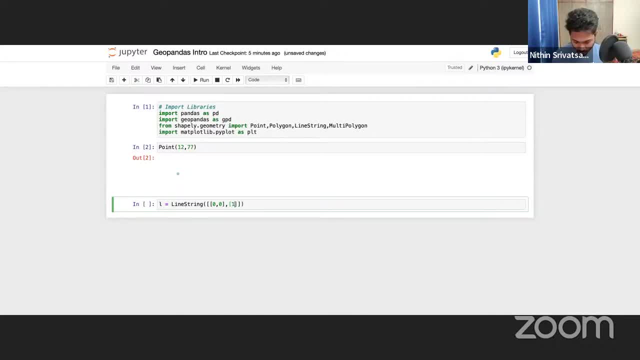 1 comma 0. and then let's say we have now, if i just plot this, you see it's a line from 0 comma 0 to 1 comma 0. now if we just do 1 comma 1, so you see how it moved. now, if i do, 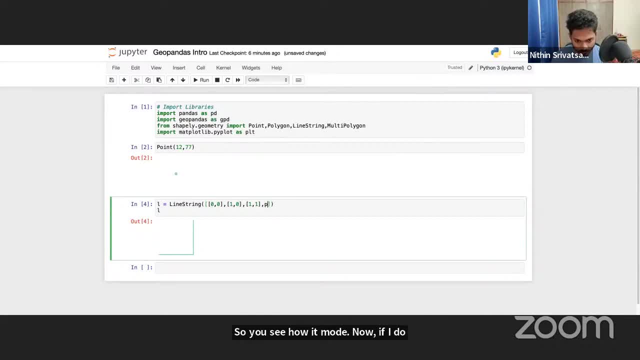 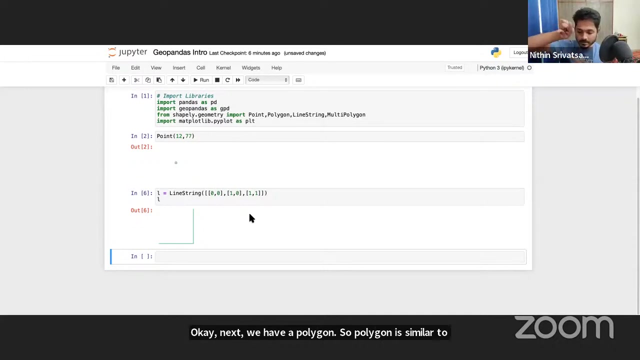 0 comma 1. so you see how those three matched right. so it's creating a line in the plane. okay. next we have a polygon. so polygon is similar to a line string, but it completes a map or it completes an area. so if we just take a couple of coordinates, 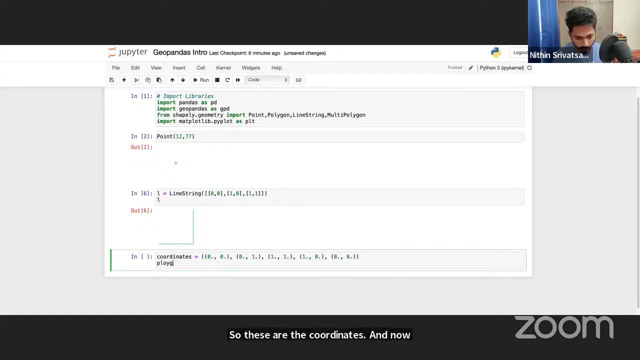 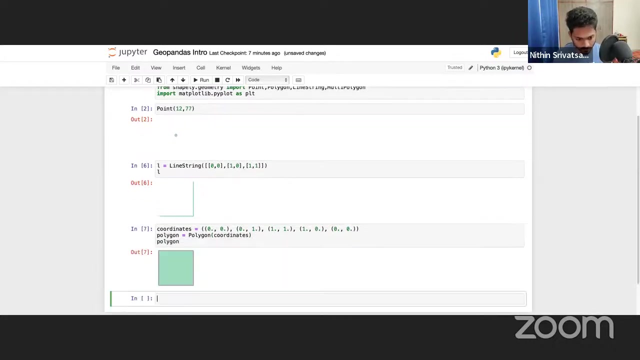 so these are the coordinates. and now if i create a polygon on top of it and let's just display that, so you see it has completed a square. now what if we were to check how it would look like if we just take a polygon on top of it? 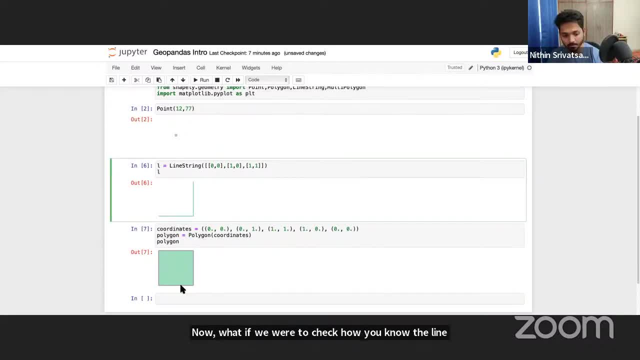 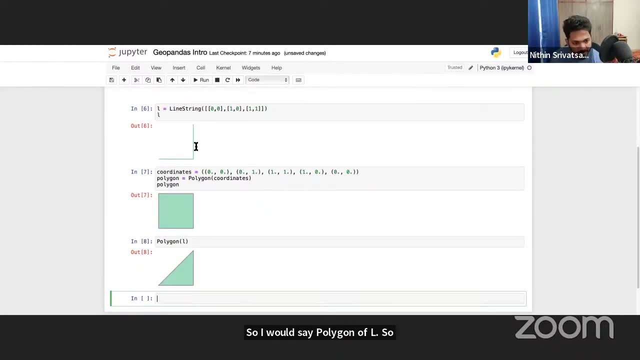 and let's just display that. so you see it has completed a square. now what if we were to check how you know the line string that we defined here as a polygon? so i would say polygon of l, so instead of these three lines, it has covered it. so this is how the back end of polygon works. 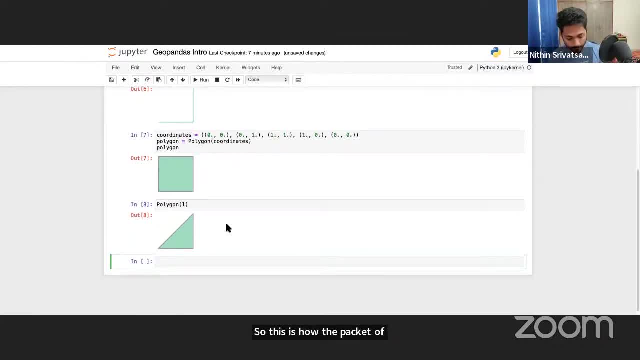 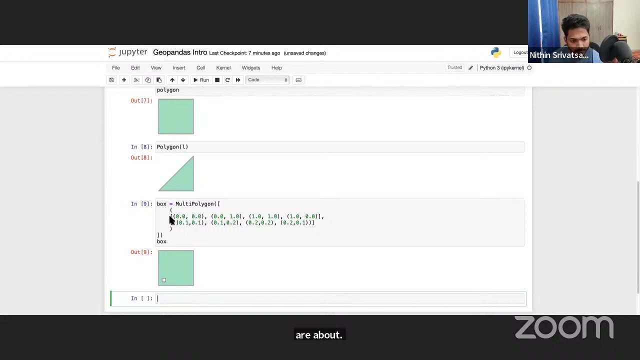 now, next again, we have multi polygons, which you know define a collection of polygons. so these are some references. so this contains the outer box, and once i printed you'll understand what these are about, right? so the outer box is mentioned here, the references, and then the second line contains 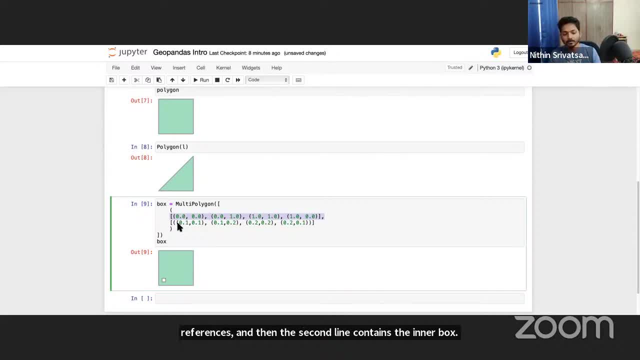 the inner box. now, how is this relative to us, or useful to us when we are dealing with geospatial data is consider, uh, you know, a polygon. polygon meaning lots of lines converged, of india, so we have the india polygon, and then, in this polygon, i want polygon of 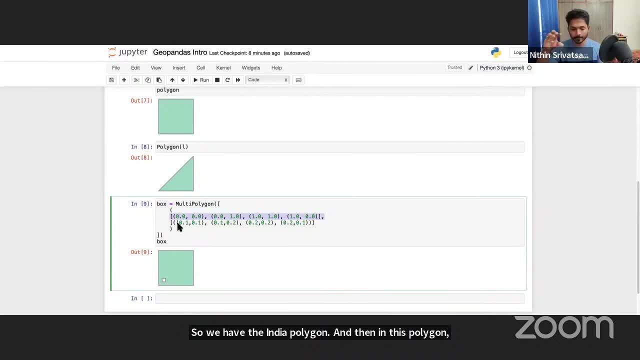 karnataka or new delhi, so i can use these polygons and filter it from them. and that contains your outer polygon, which is your india, and the uh inside polygon is your Antarctica. so there are some data sets that are inbuiltly available to you. uh, you can enjoy integration positions. yeah, we just need to copperize this polygon using contact fit and we can softerize the podía column, which means converged of india, so we have the india polygon. and then in this polygon, i want polygon of karnataka or, you know, new di, unconditional, so i can use these polygons and filter it from them. and that contains your outer polygon, which is your india, and the inside polygon is your map. �zikek, boric by米. you can look at thisriver itself. so it's always important because if it's broke down, intoolic compendia, denotification, lost, uncertainty, descendumber. we want spec wheel char, if you. 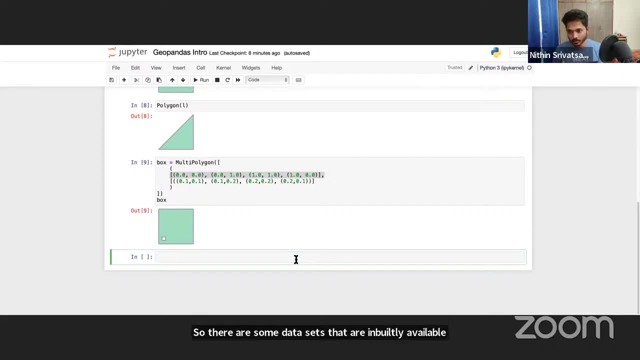 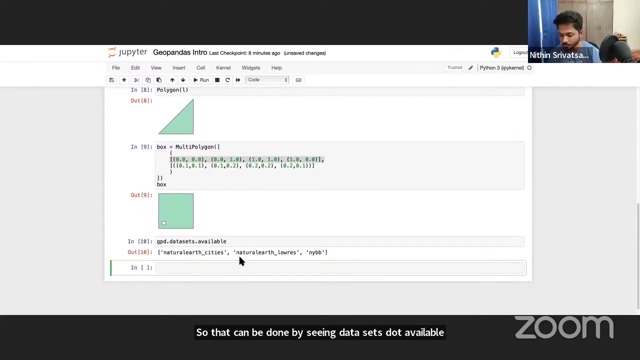 available in GeoPandas which we can use, which we can play around with and try to get hands on how GeoPandas works. So that can be done by seeing datasetsavailable. We'll explore this one by one so you understand what these are and how they work on the backend. 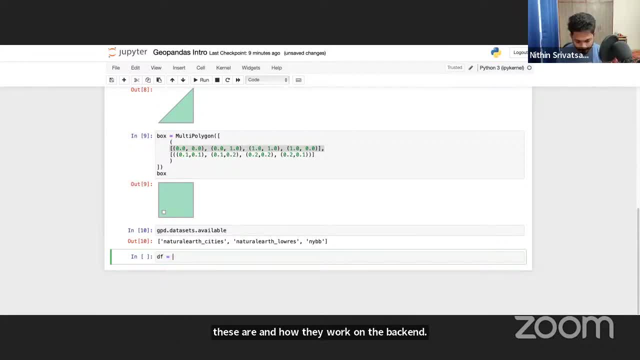 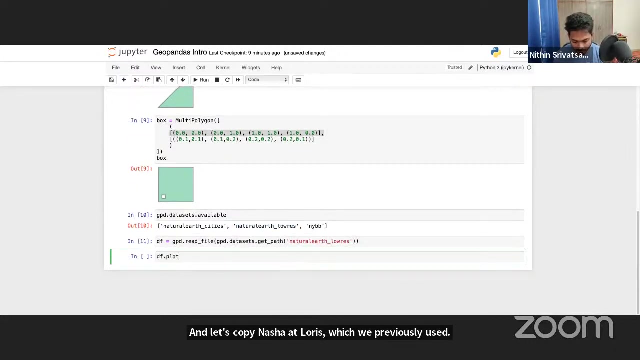 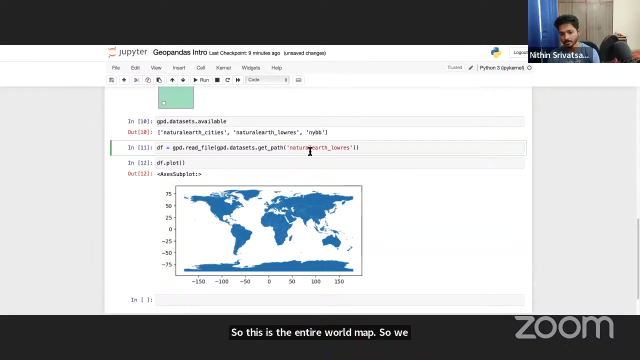 Let's just read the file. So getPath gives the path in which the library is present, and let's copy naturalEarthLores, which we previously used. And now, if I just plot it now, let's not use any resolution. So this is the entire world map which is present in naturalEarthLores. 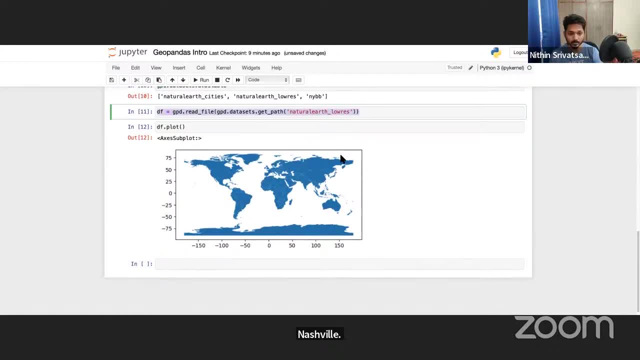 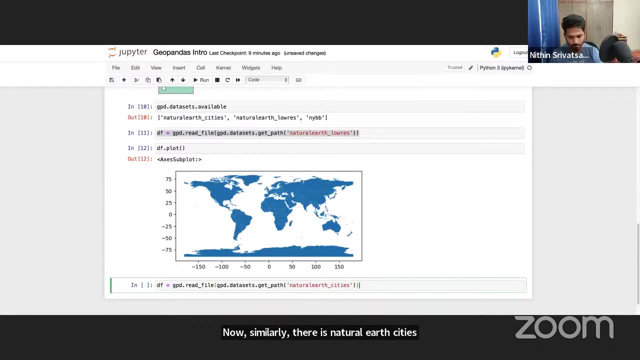 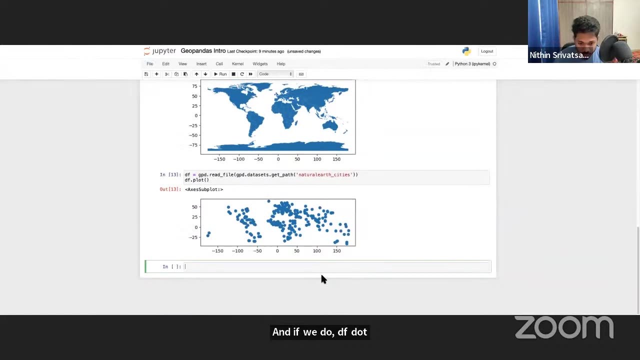 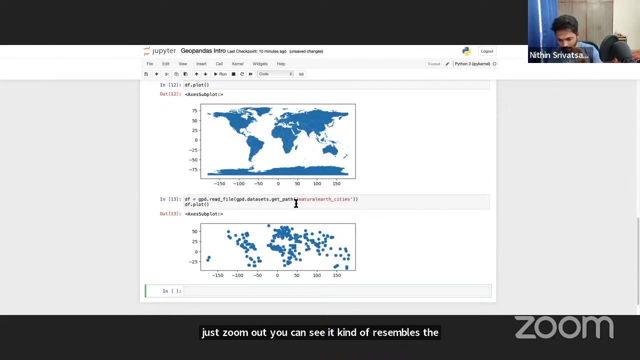 Now, similarly there is a naturalEarthLores If we plot cities and if we do dfplot. So now this maybe if I just zoom out you can see it kind of resembles the world map, not exactly, but kind of resembles it. 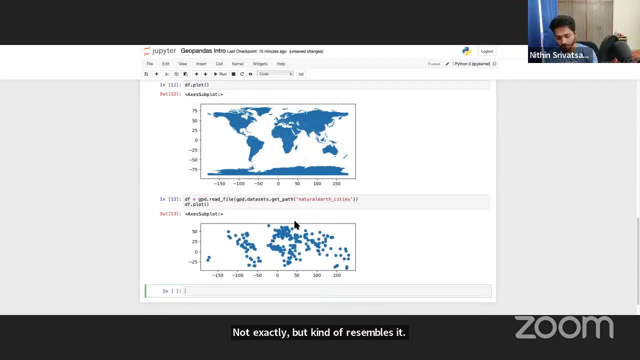 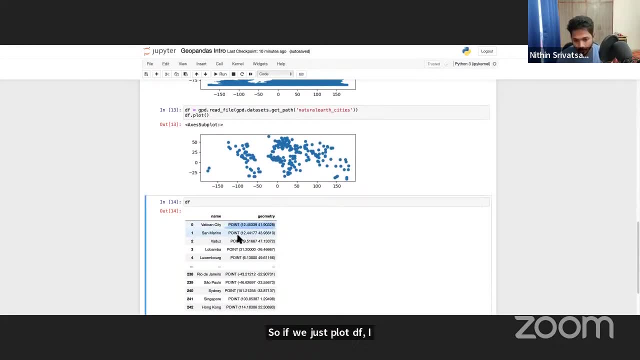 So this dataset contains all the major cities that are present in the world. So if we just plot df, I mean look at DFA. so these are single points which we discussed: a point on the map and there are city names, you know, Luxembourg, London, Singapore, Hong Kong, each having a point on the map. and finally, 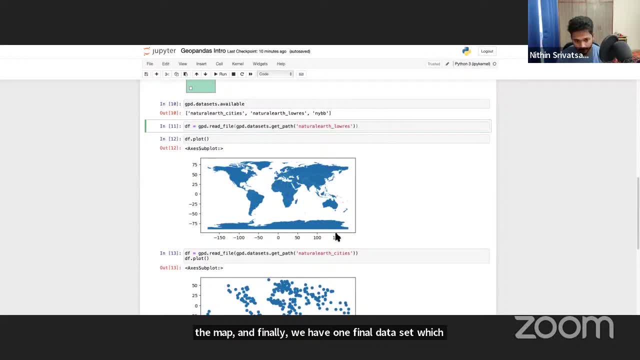 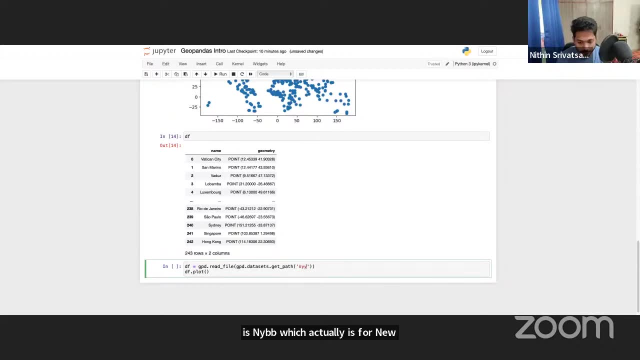 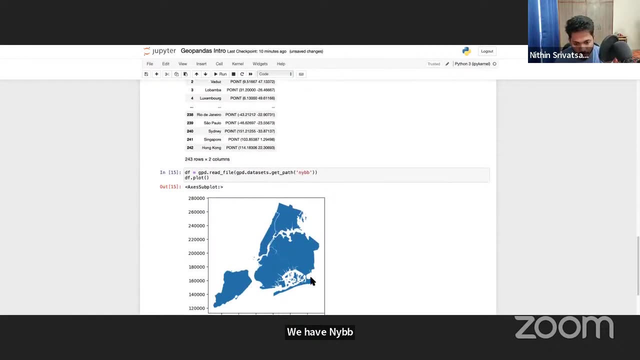 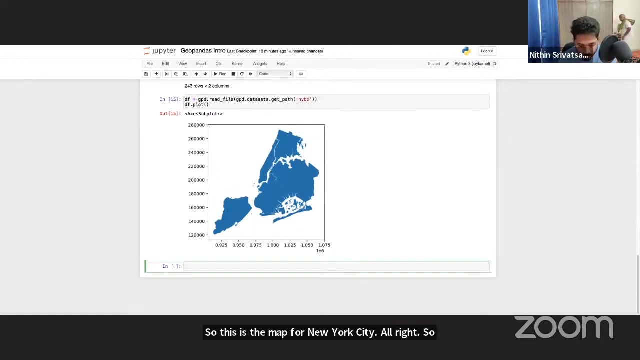 we have one final data set, which is NYBB, which actually is for New York cities. we have NYBB, so this is the map for New York City. all right, so these are the available data sets here. now, if we go back to our Pandas, EDA. 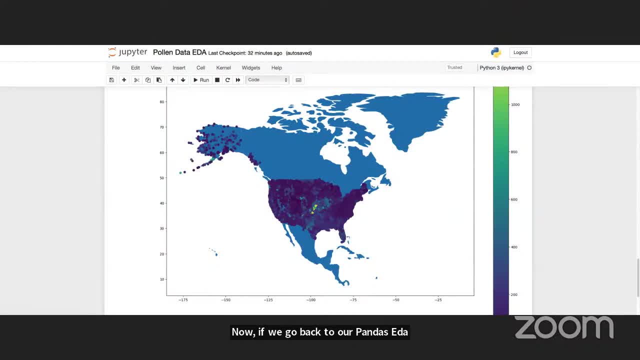 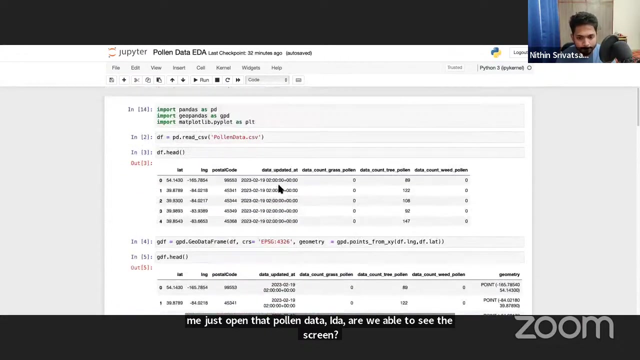 just a second, guys. let me go back to our Pandas EDA. let me go back to our Pandas EDA. let me just open that Poland data EDA. now are we able to see the screen? yes, you can, okay, cool, okay. so now, if we deep dive into code now, you'll understand what's happening in the backend. 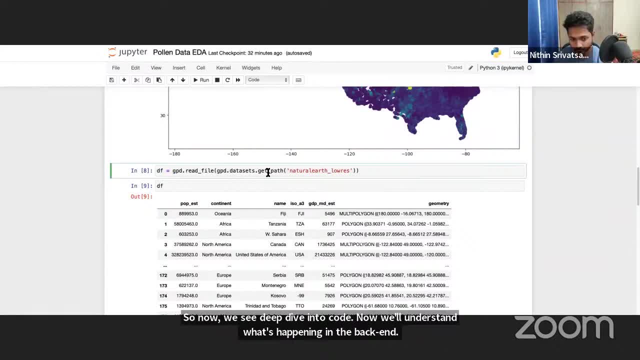 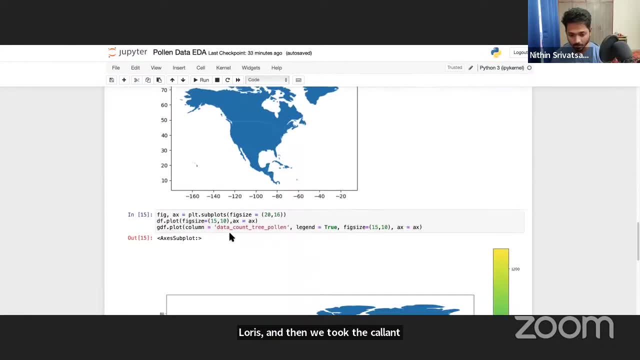 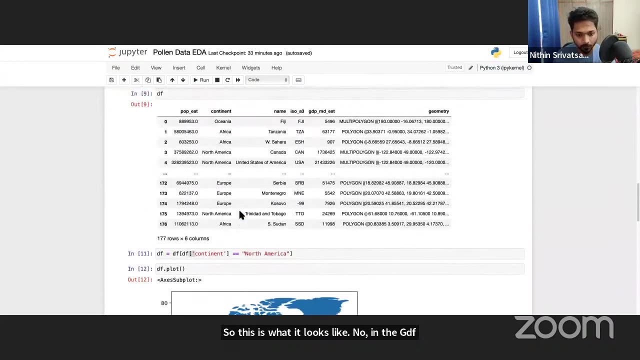 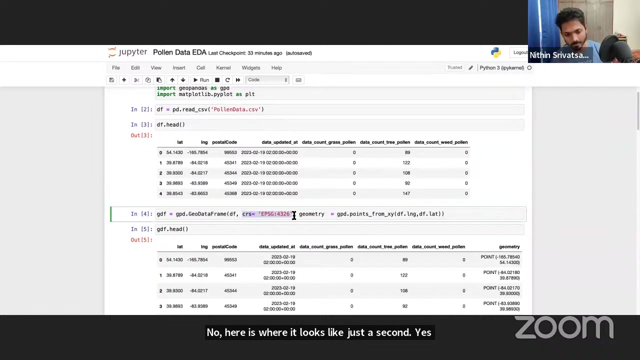 so we took the GeoPandas data, which is the natural earth lores, and then we took the continent North America. so this is what it looks like now in the GDF plot we plotted the tree count. now here is where it looks like. just a second, yes. so this is what I wanted to explain. is CRS. so again, coordinate. 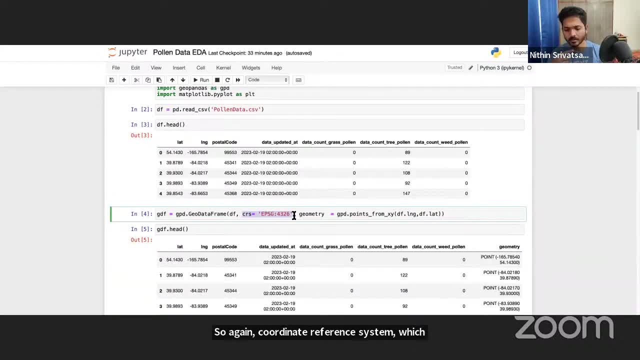 reference system which is accepted standard. now there are multiple coordinate references system which will be you can. there are a lot of CRS which you can look up and so, as I told, this is the accepted one, but there are others which have you know, clipped, uh, Antarctica and Arctic, and there's a actual relative distance map and everything which 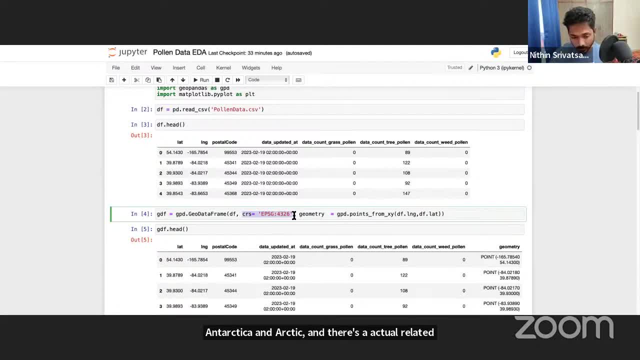 my teammate Parikshit will be talking in the next session which deep dives into what the basically deep diving to a lot of visualizations on GeoPandas data frame. we'll be looking at chloropleth maps and stuff, so make sure you register to that as well. it's a pretty interesting. 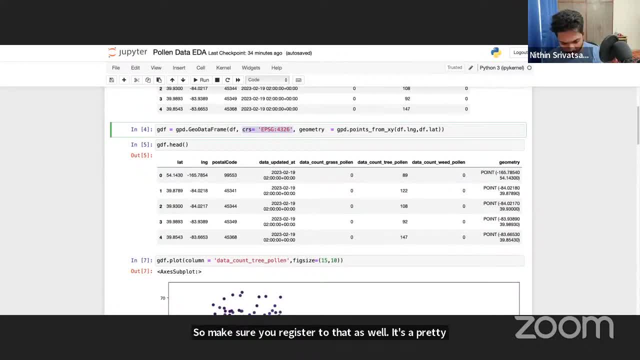 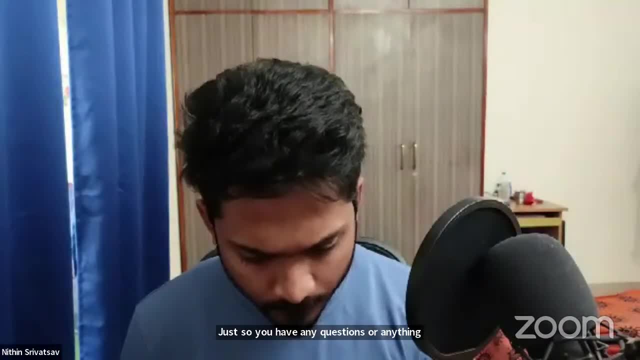 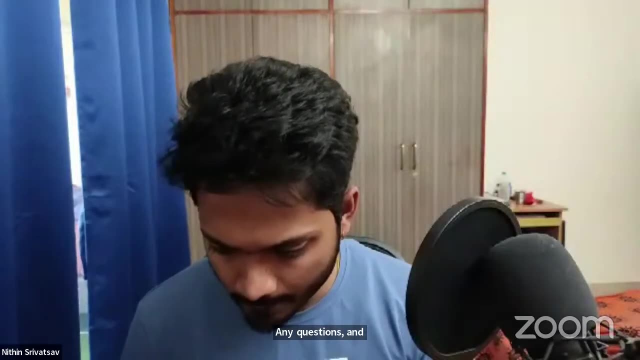 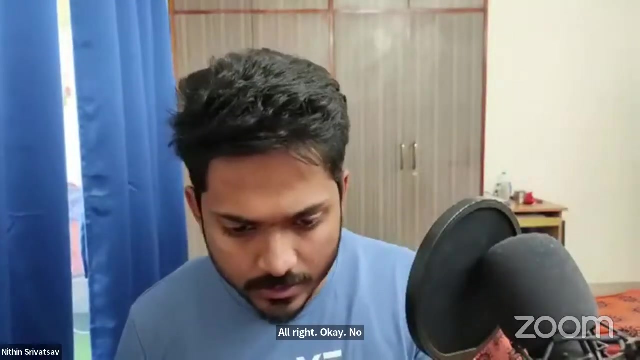 session. okay, I think I'm going to stop here and I'll see you in the next session. bye-bye, bye-bye, bye-bye, thank you. thank you, interesting right. uh, yeah, I don't look at it, so I just, I don't question, leave that. 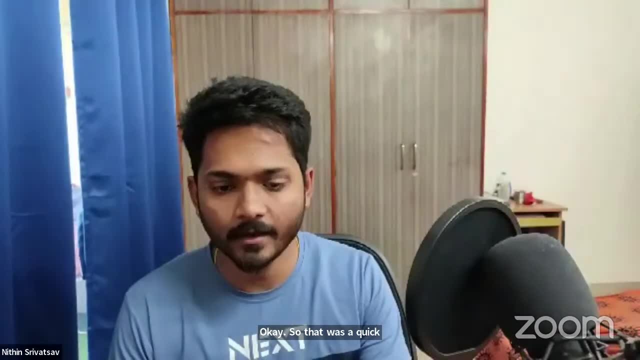 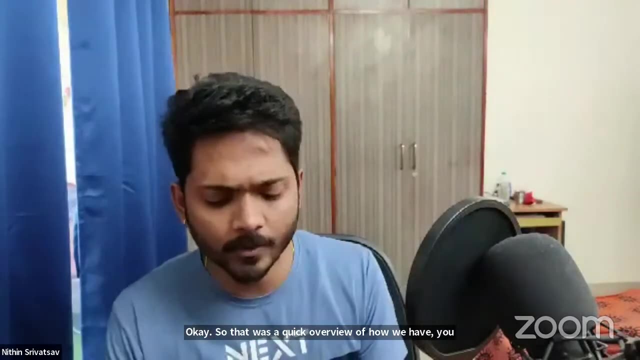 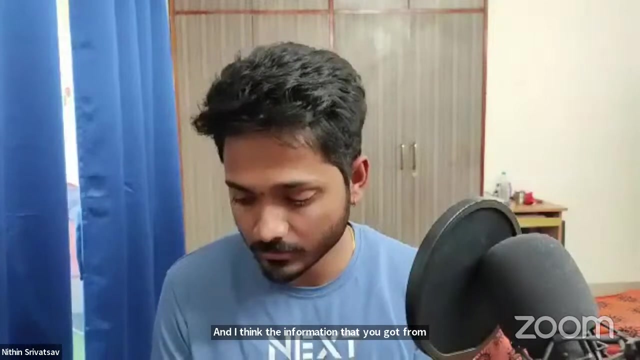 transfer you okay. so so how? we have Geopandas, which is the go-to library for us, and then a couple of satellite formats that are present, And I think the information that you got from this presentation should be enough for you to just get started with geospatial data science. 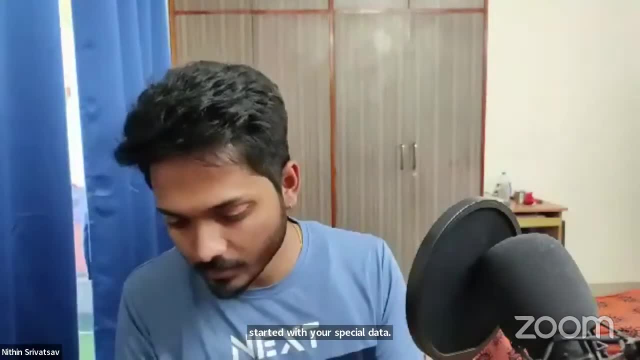 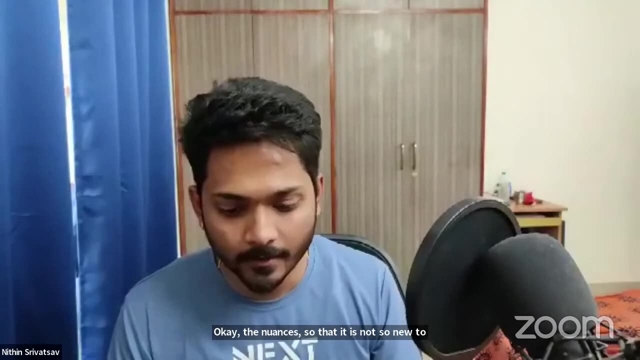 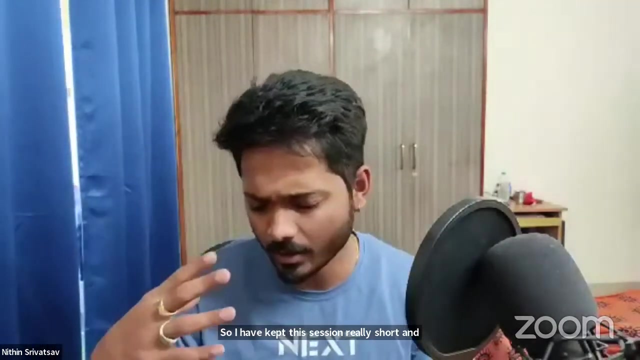 And also, once you dive into it, you can understand the nuances so that it's not so new to you and stuff. All right. so I have kept this session really short and light-weighted, so not attached to deep dive. There are a lot of other things that we can do with Geopandas data frame. 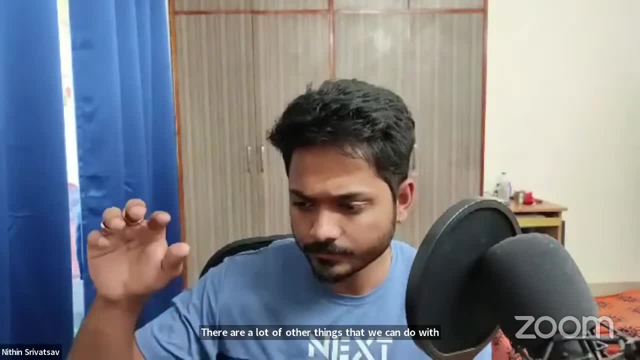 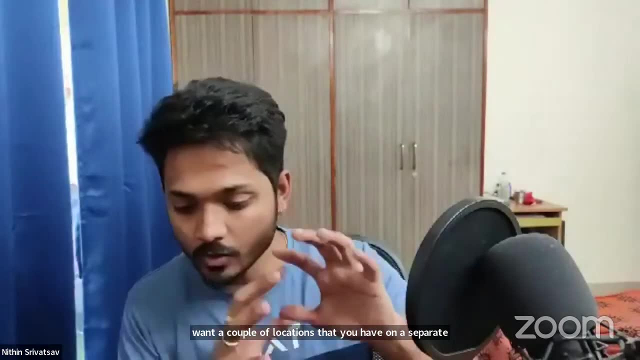 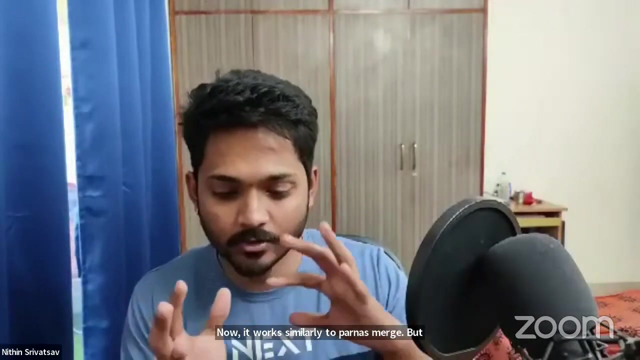 You know there is spatial join, meaning you know you want a couple of locations that you have on a separate data set and you want all those locations from another data set. Now it works similarly to Pandas merge, but Pandas merge is more on your numbers. 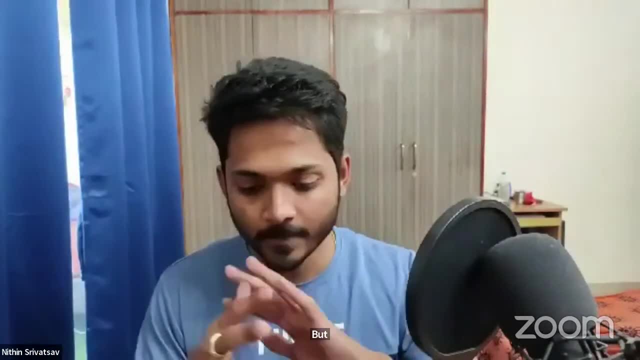 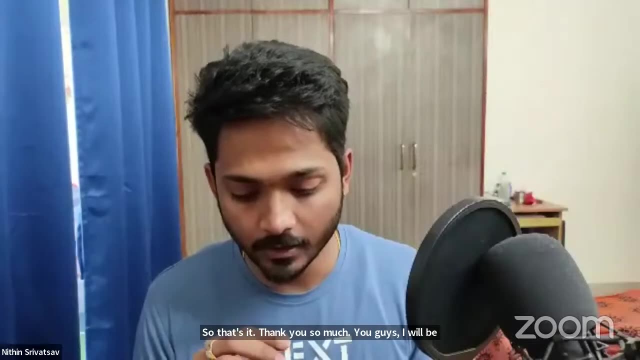 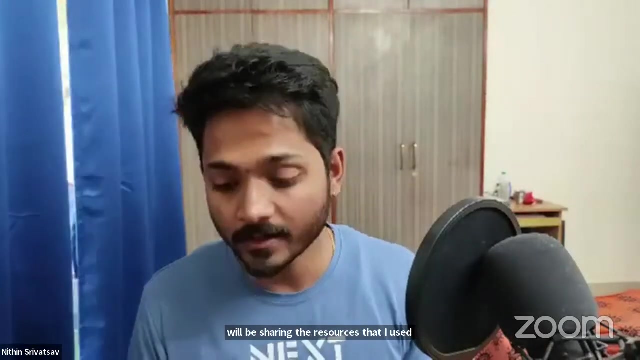 but S-join is more on a spatial level. So that's it. Thank you so much, guys. I will be sharing a couple of I'll be- I think the team actually will be sharing the resources that I used here and also a GitHub link where all your resources 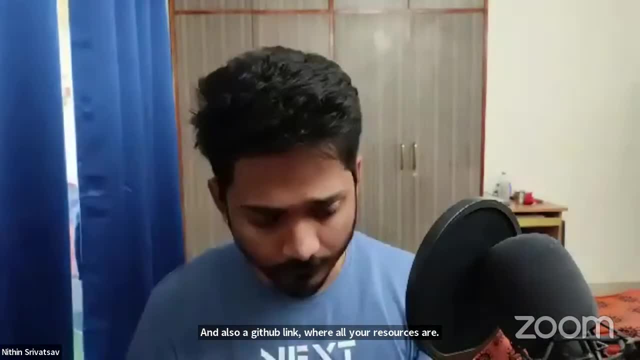 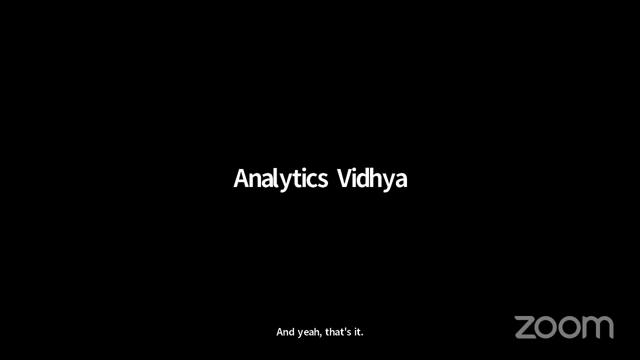 or the notebooks that we presented here will be available to you. And yeah, that's it. Thank you so much. Yeah, before we proceed to answer your question, I would like to request the attendees to please fill the form of the feedback, as it helps us to conduct more such sessions. 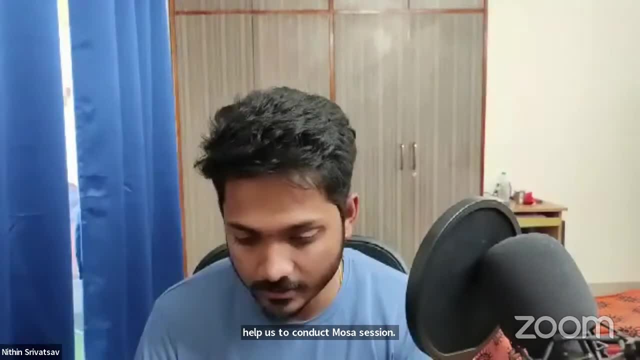 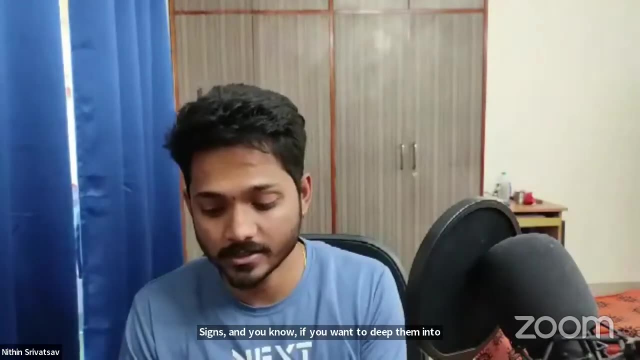 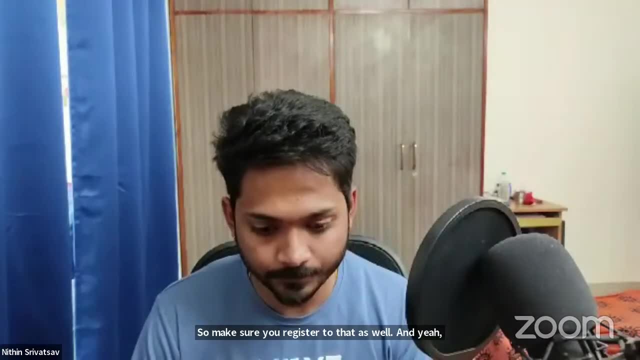 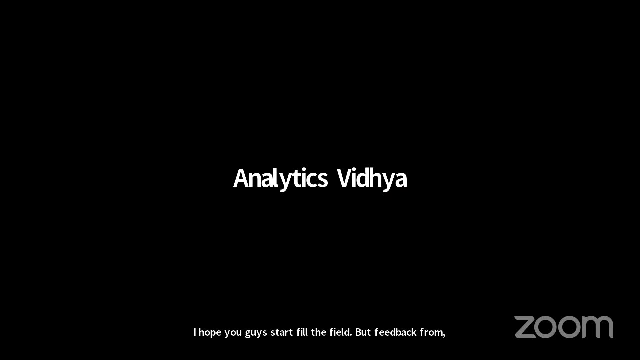 Thank you, Thank you, Thank you And, yeah, let us know how we can be of help. I hope you guys have filled the feedback form. If not, I request you to please do it And if you wish to conduct a webinar or facing any difficulty in registering, 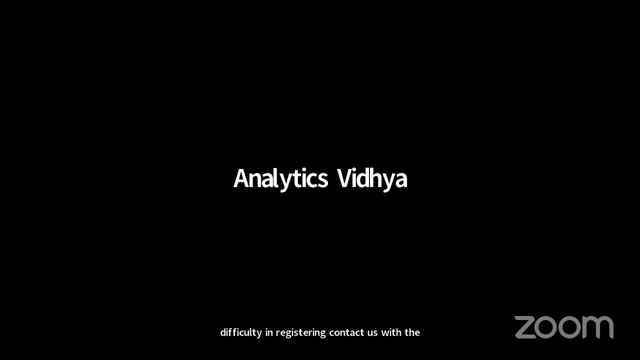 contact us with the email provided in the chat section. The recording of this session will be available within two days on our YouTube session or YouTube channel And we will be back with another session of the data at 3 pm today. The link is in the chat section. 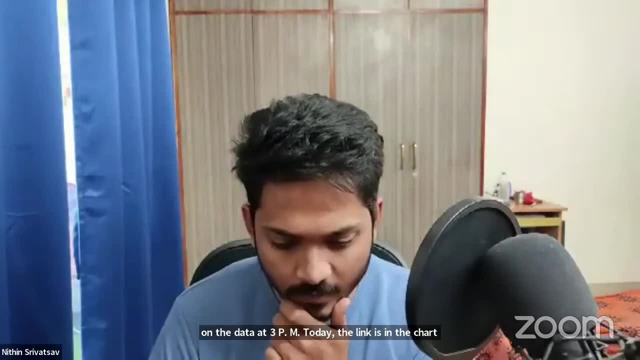 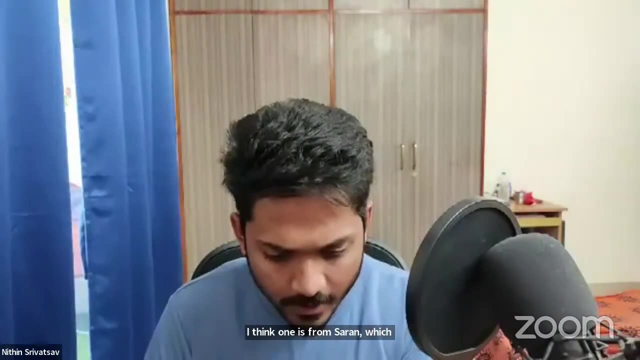 Till then, have a good time, Keep learning, Keep learning. Yes, Okay, I think we have a couple of questions that are left unanswered. I think one is from Sarang, which is: from which satellite do we get this data and how? 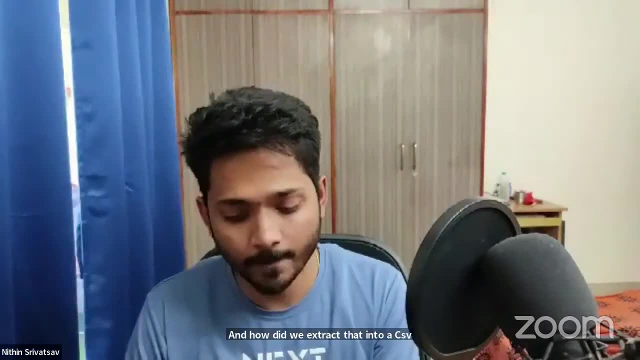 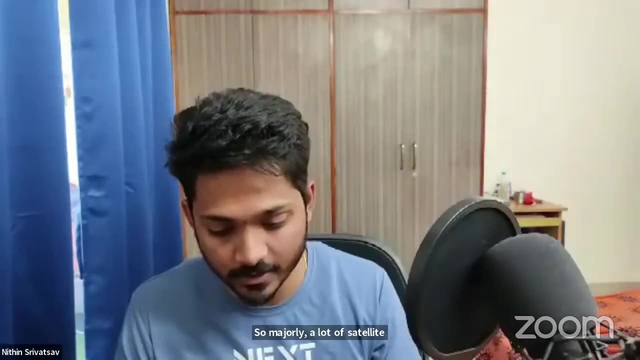 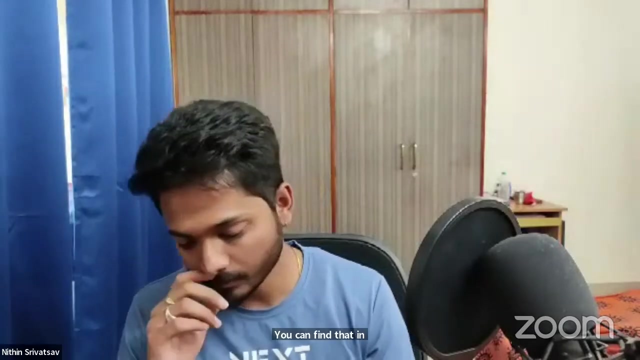 did we extract that into a CSV Right? So majorly a lot of satellite data that has HDF files and HDF is basically from NASA. You can find that in earthdatanasacom: A lot of parameters. So there's weather, there is cloud cover, there is water vapor, there's soil. 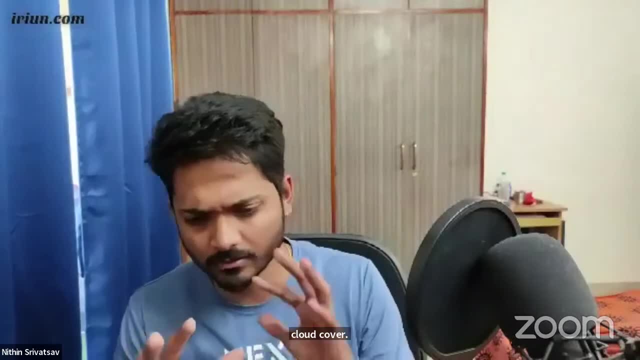 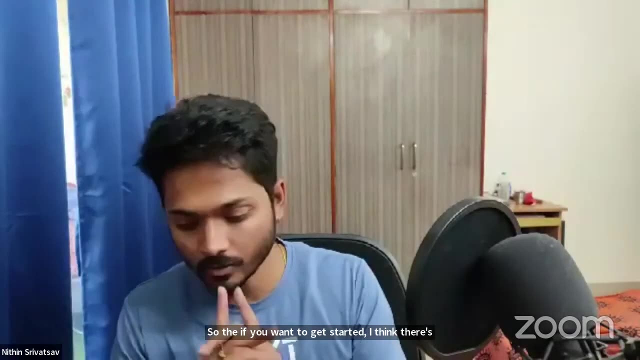 and a lot many things that you can play around with. So if you want to get started, I think there's probably a registration page on NASA which you can, you know, log into and then you'll have free access to the data sets. 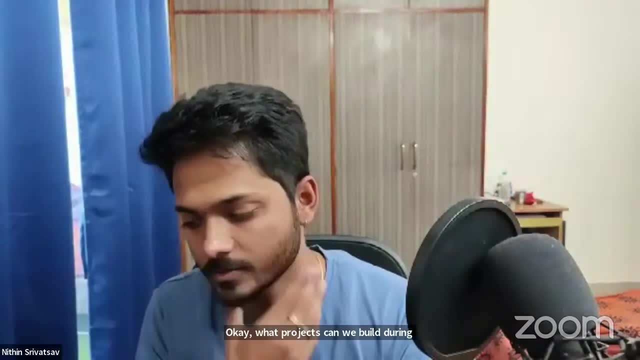 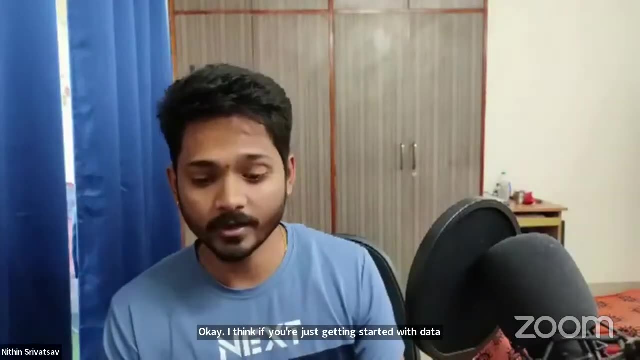 Okay, What projects can we build? What projects can we build during learning geospatial data? Okay, I think if we're just getting started with data science, you know Uber data set is a really good way to start. So you can take the lat long. 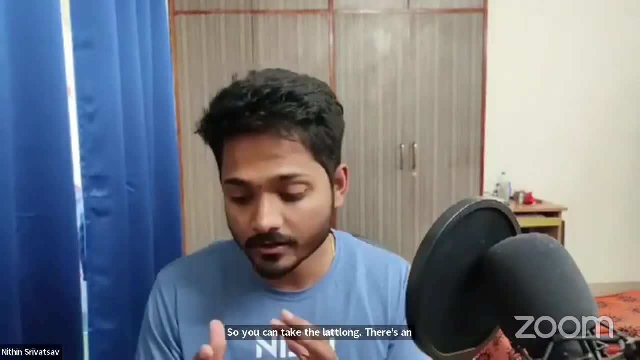 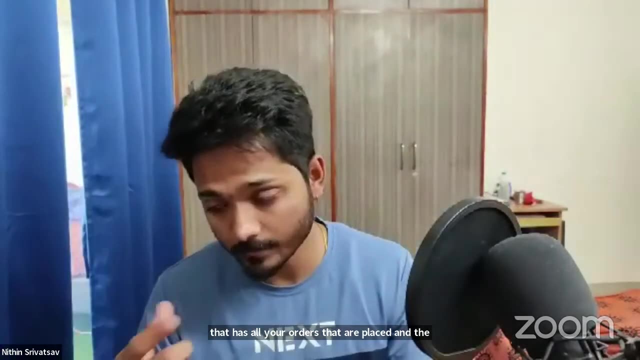 There's an entire data set that has all your orders that are placed and the locations from where a request was made and request was served. request was not served also, So I think that is a pretty useful data set that you can get started with. 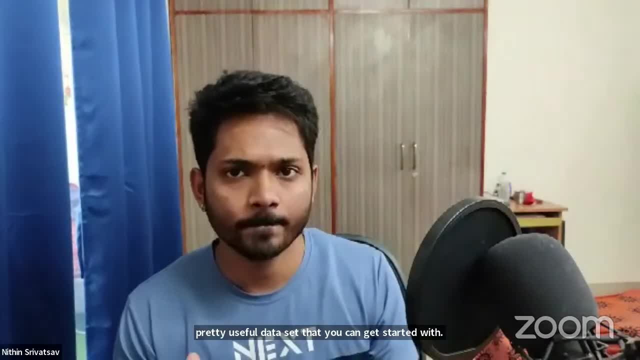 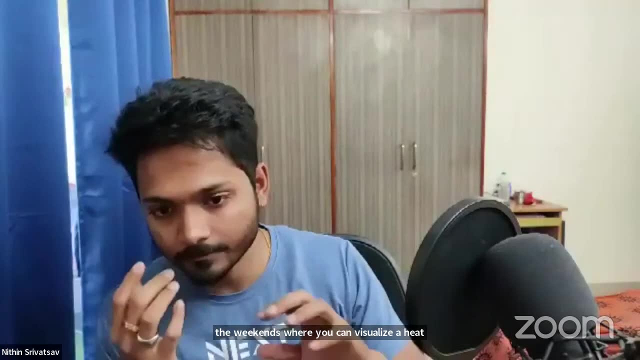 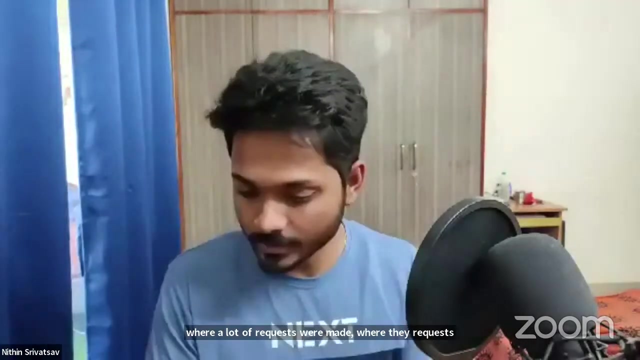 So you know a lot of You can do. say, you know in the weekends where you can visualize a heat map on where a lot of requests were made, where the requests failed, where were there a lot of requests but we couldn't, you know, serve them because the costs were not available. 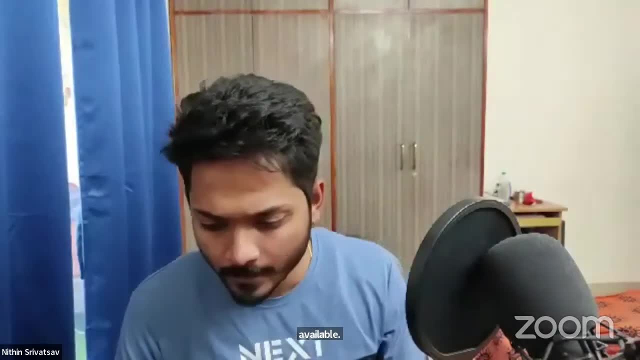 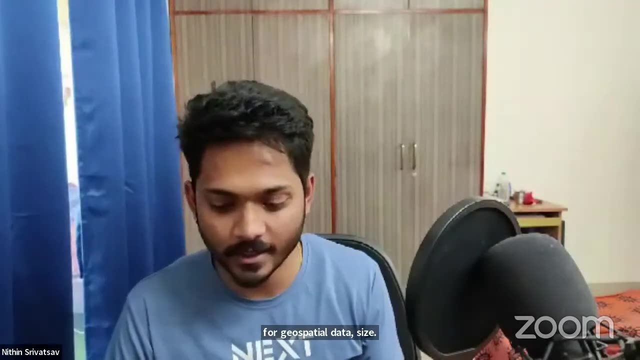 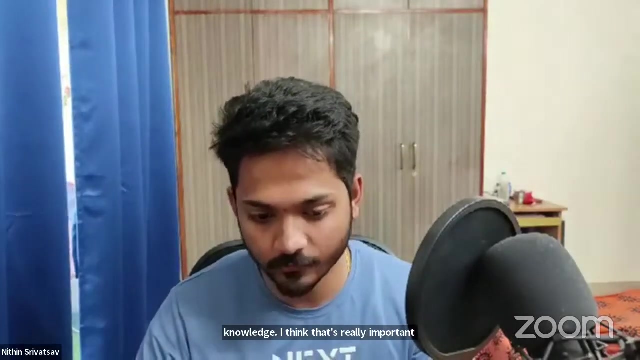 So all these sorts of EDA, Okay, A full roadmap for geospatial data science. I think That starts with first understanding the domain knowledge. I think that's really important. So if you want, like from a starting, you know base A to Z kind of thing starting, 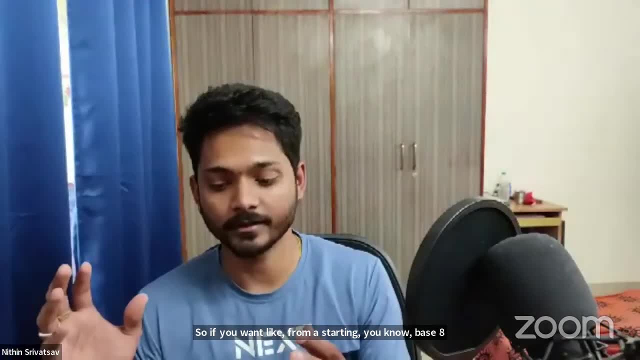 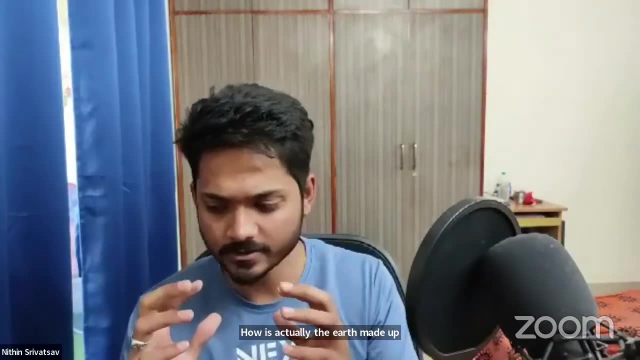 from zero. I think you would first need to start with the latitudes and longitudes. How is actually the earth made up of? what are the coordinate reference system? How can we identify location? All of this which has Actually been discussed in the seminar. 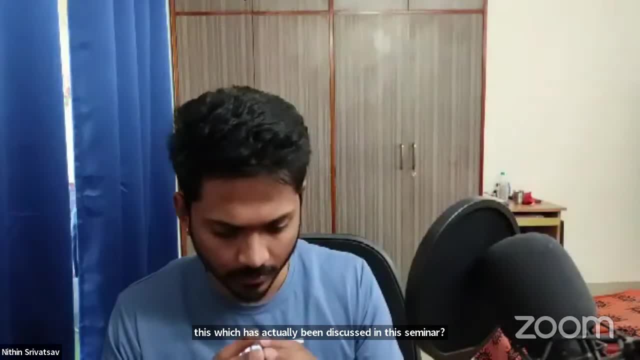 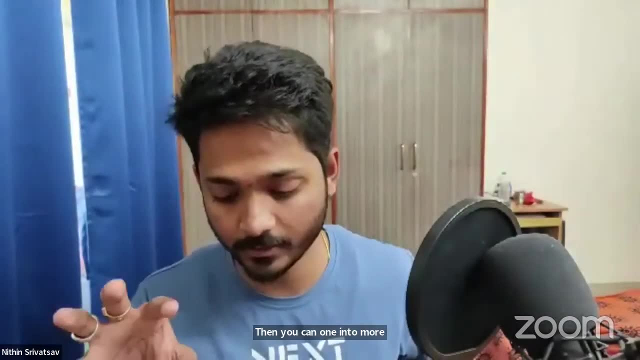 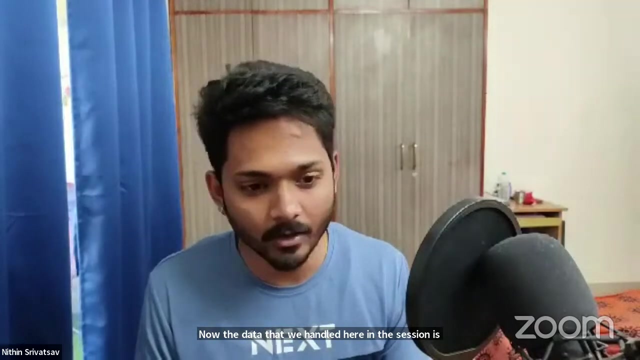 Once you have that basic basics of domain knowledge built into you, then you can move on into more advanced things like playing with data frames. Now, their data that we handled here in this session is pretty lightweight: It's not even an MB or two MB. but when you start deep diving to big data sets like say, 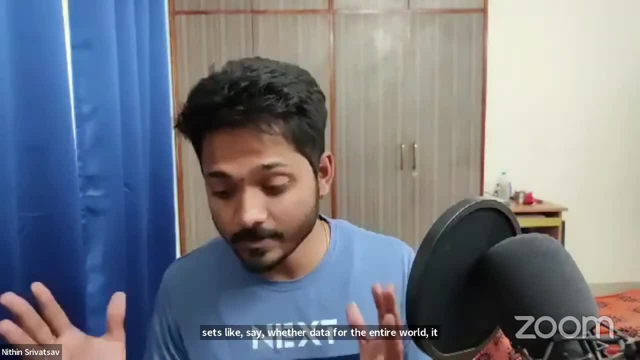 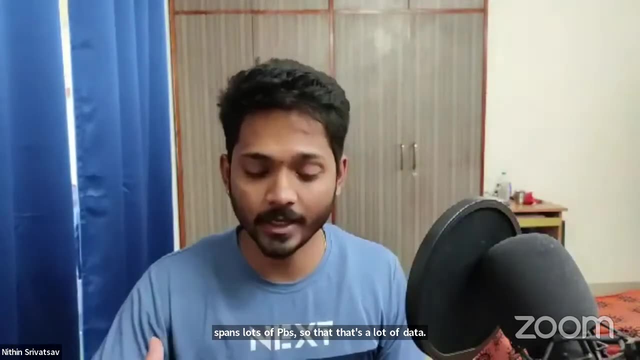 weather data for the entire world. it spans lots of PB, So that's a lot of data And I think, uh, the tool that's being used to will come into play and where you can deep dive into the tool, say GeoPandas. 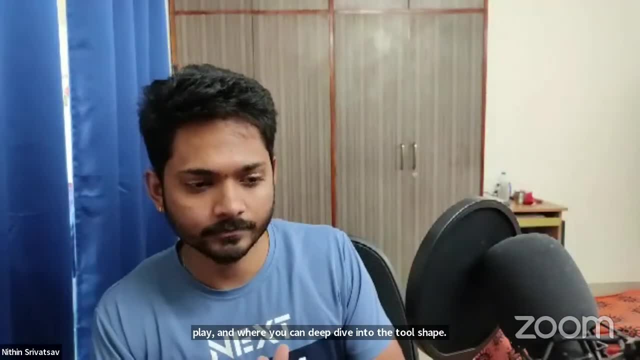 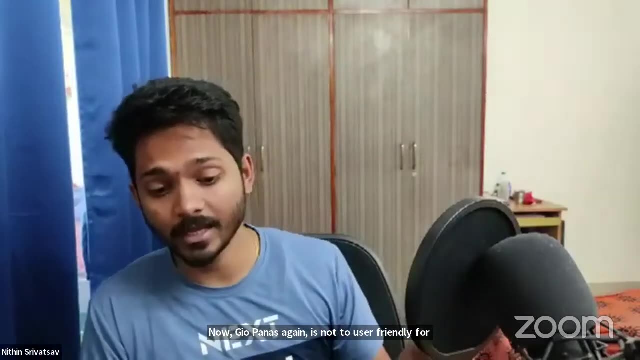 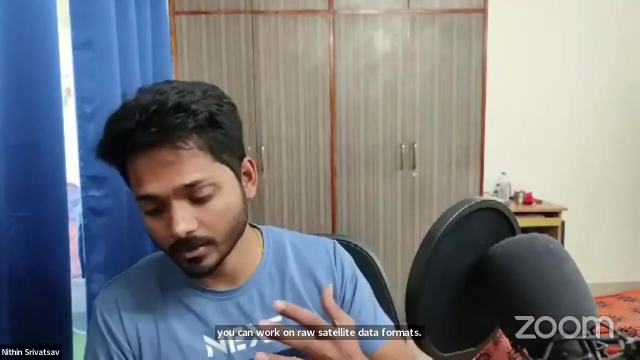 Now GeoPandas again is, uh, not very user-friendly for handling very large data sets. There are separate data sets available, like X-ray, which you can work on raw satellite data formats. I think those would be helpful in a production environment. 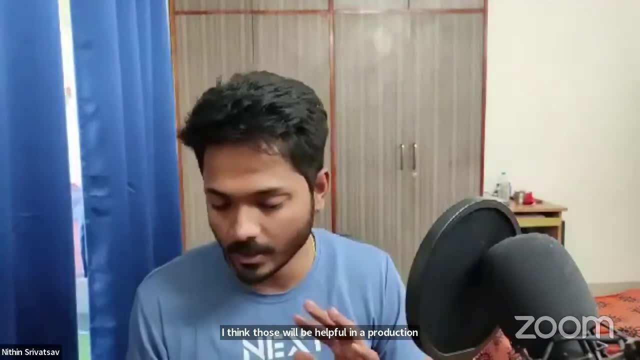 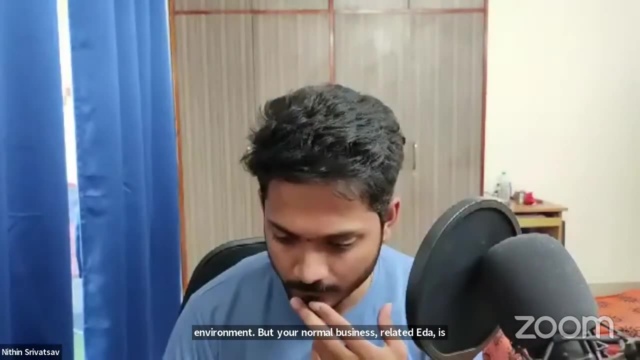 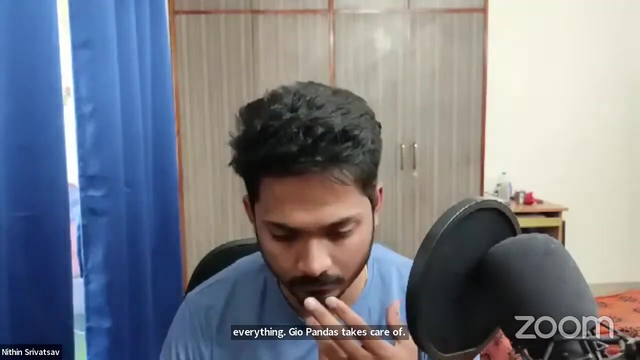 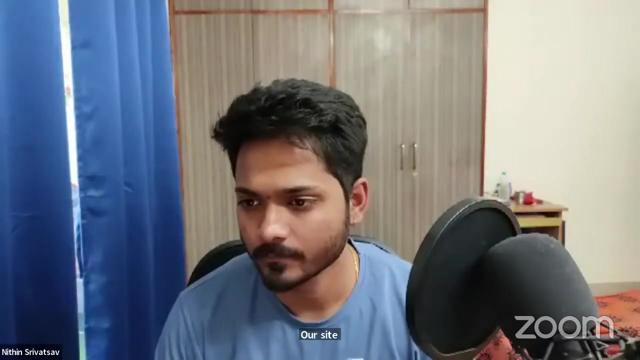 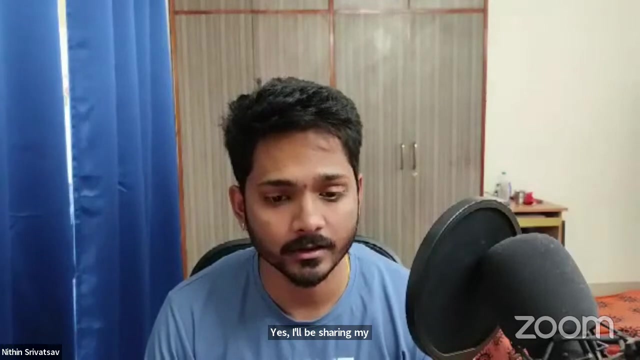 But, But your normal business-related EDAs, everything GeoPandas takes care of All right, Uh, yes, I'll be sharing my quote on the GitHub. Uh, I think. uh, it's. it'll be available in the resource section. uh, along with the. 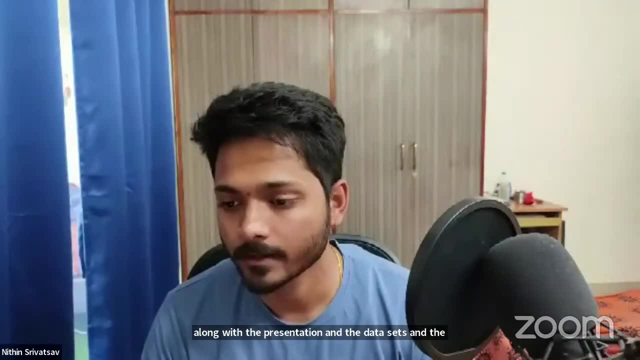 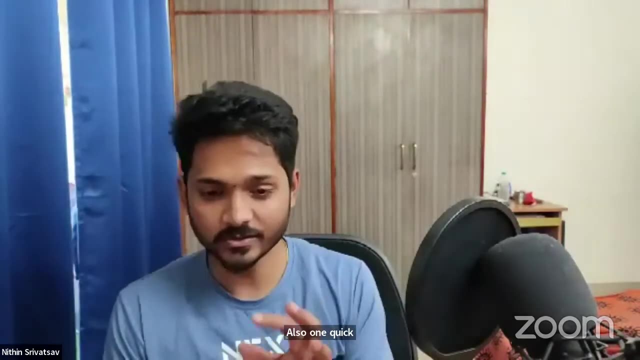 presentation and the data sets and the GitHub link. Also, uh, one quick, uh shout out, shout. not shout out actually, but uh information. So since we understand- uh, I mean Ambi and my teammates and I- since we understand the 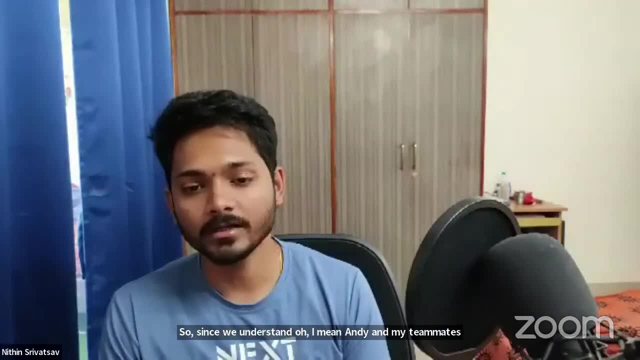 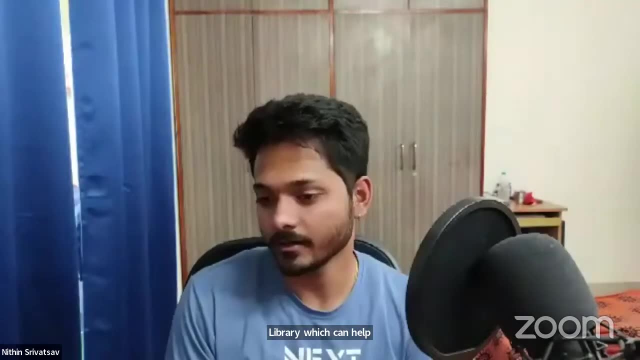 importance of geospatial data. what we are doing is we are creating an open source library which can help you soak You. you saw how we plotted right And in the next session that my teammate takes, you'll be looking at even more plotting and 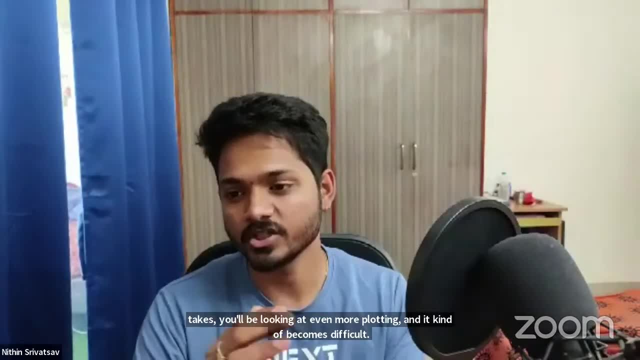 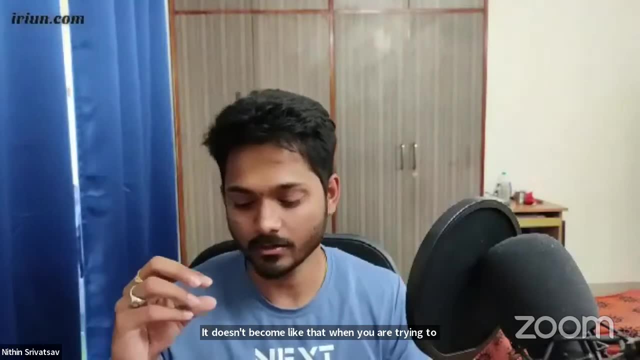 it kind of becomes difficult. It's not straight forward like GDF dot plot. It doesn't become like that when you are trying to- uh, you know, make a lot of changes, uh, or, or, visualize it in a more deeper way. 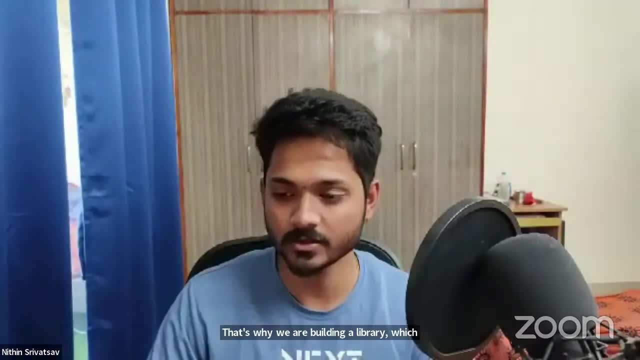 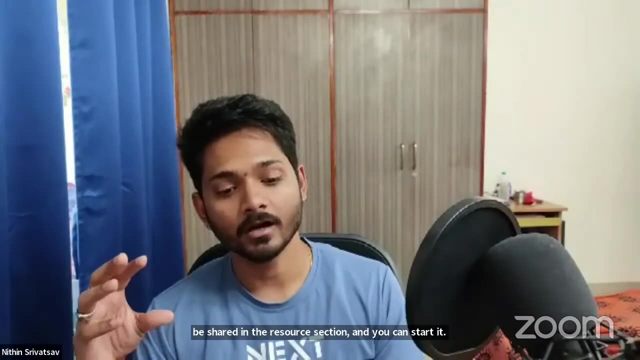 That's. that's why we are building a library, which again will be shared in the resource section and you can start it and we are planning there's a huge roadmap built around open sourcing things And, uh, especially with respect to geospatial data science. 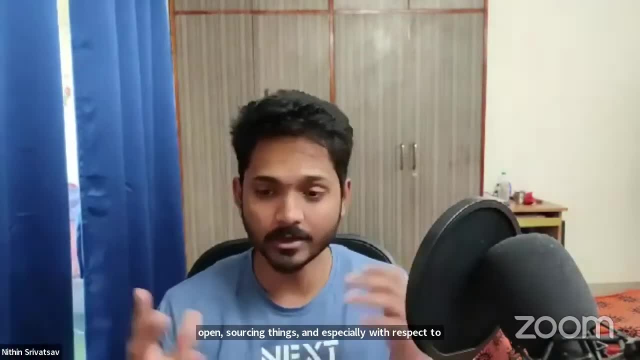 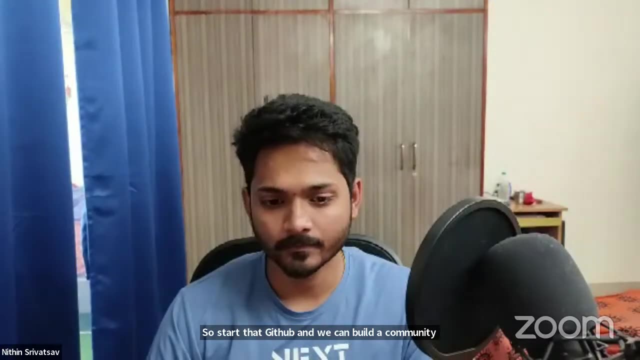 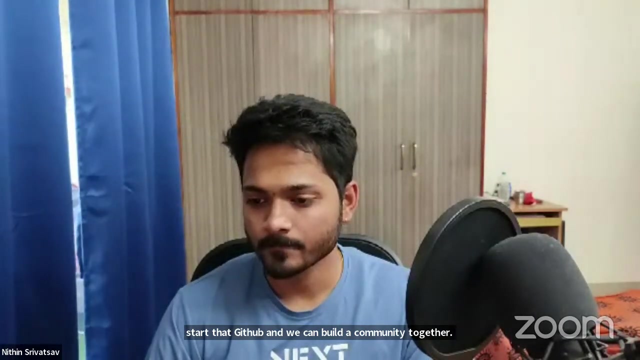 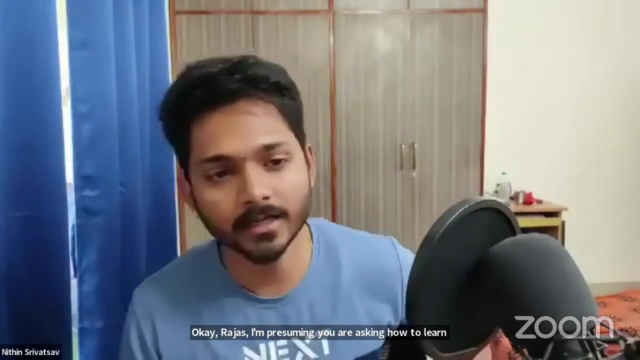 So start that GitHub and, uh, we can build a community together. Okay, Uh, Rogers, I am presuming you're asking how to learn QGIS. Uh, I can actually pray. uh, just Give a very small intro on how it works. 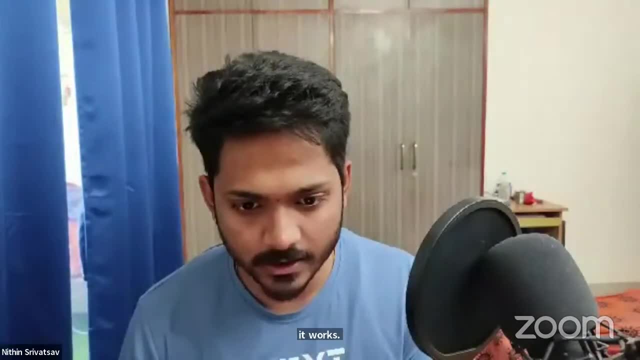 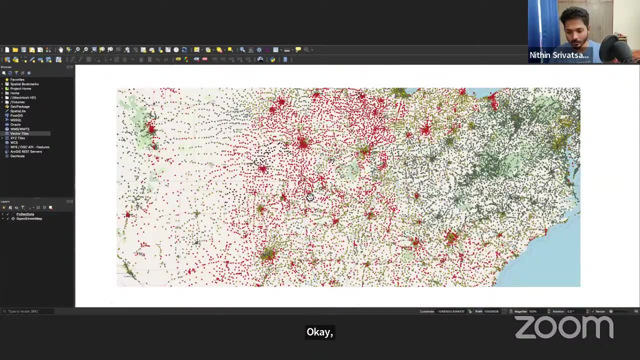 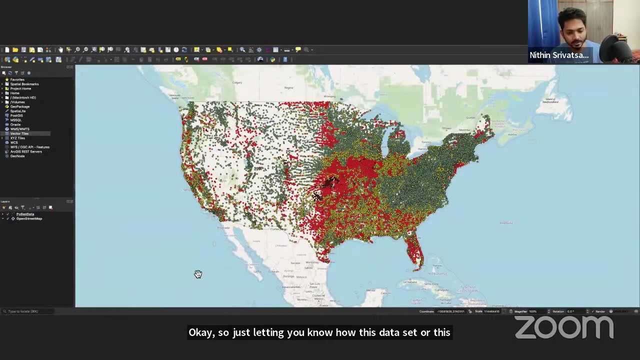 I won't deep dive much, but, uh, let me just see if the QGIS is present. Okay, So just letting you know how this data set out of this map came into picture is uh, so we need to create a layer first. 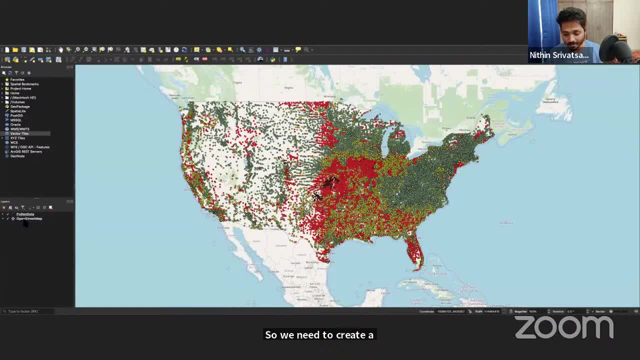 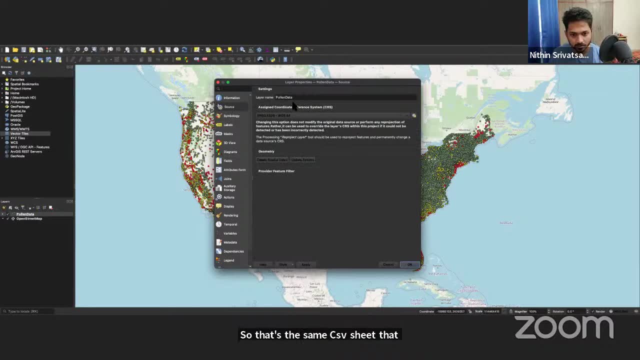 Okay, I I'll keep it very light here. Uh, so we did an ED on the Poland data, right? So that's the same CH Sweet She that's linked here. If you go to the source, it's the Poland data which the CSP sheet that we read and we have. 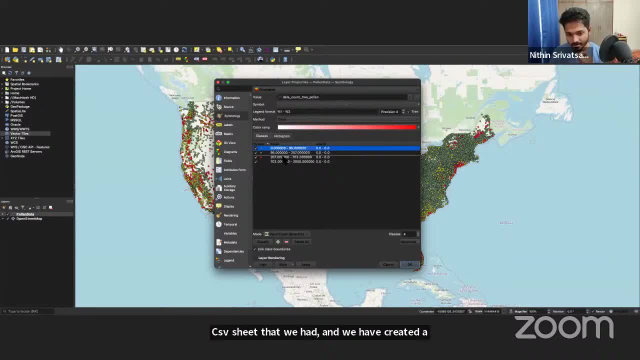 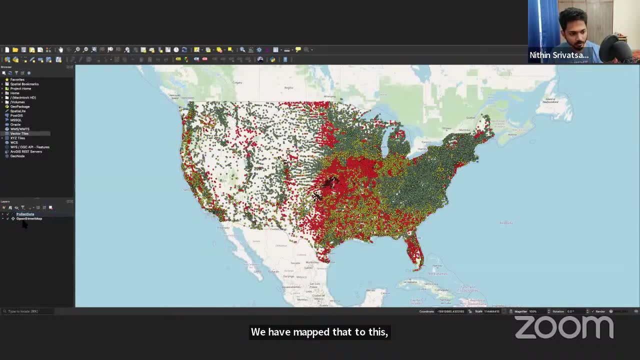 created a symbology or classes. So these are the risk levels of the Poland data set. We have mapped that to this and this is an open street map that's freely available on QGIS which you can use, So we pull in that layer. 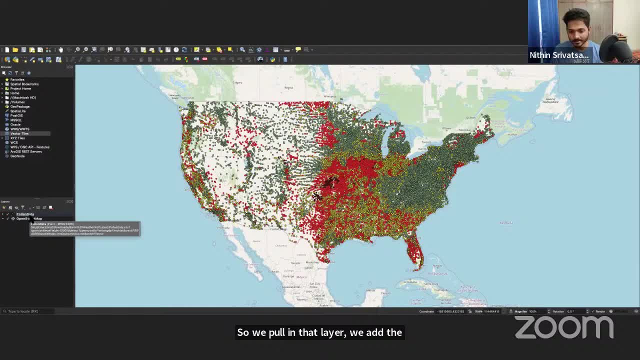 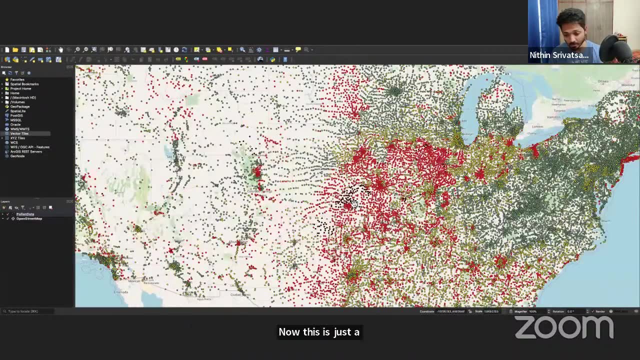 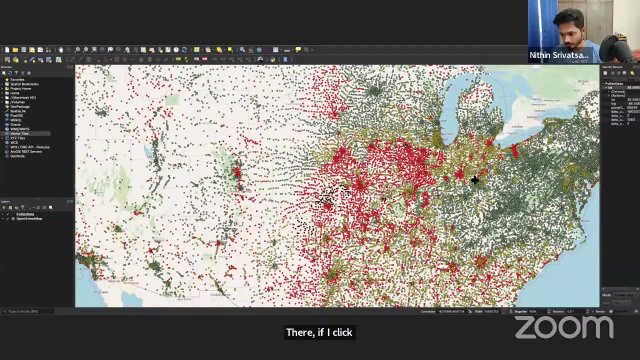 We add- uh, the polar layer. on top of it, We add classes, and that's how We are able to get this. Now, this is just a visualization. right now, I can actually look at the data present there. If I click on I and a single point, you can see the data that's present here. 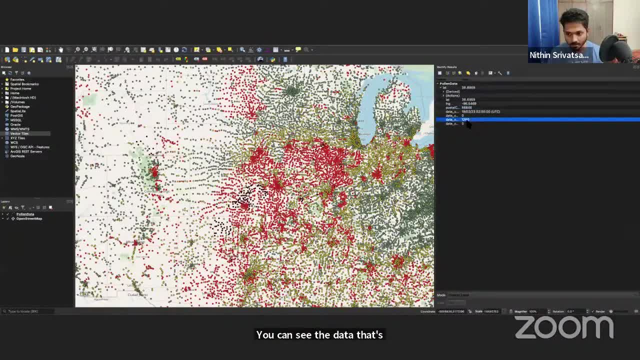 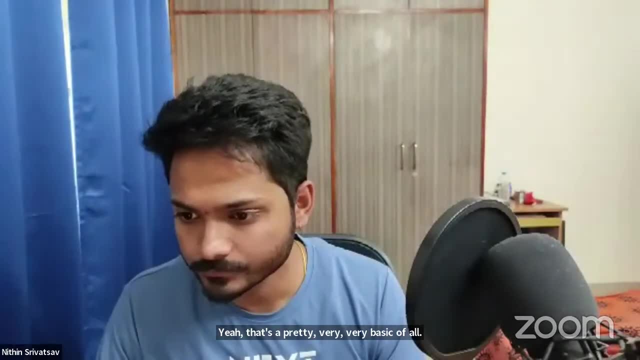 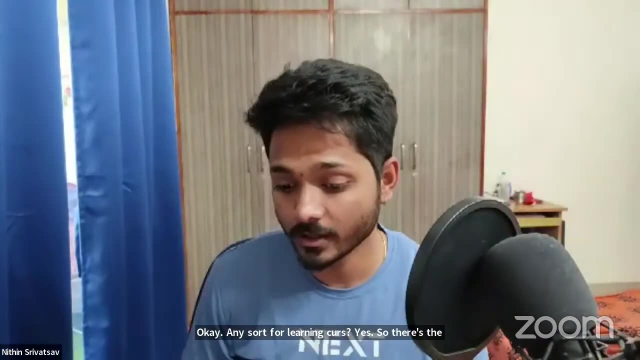 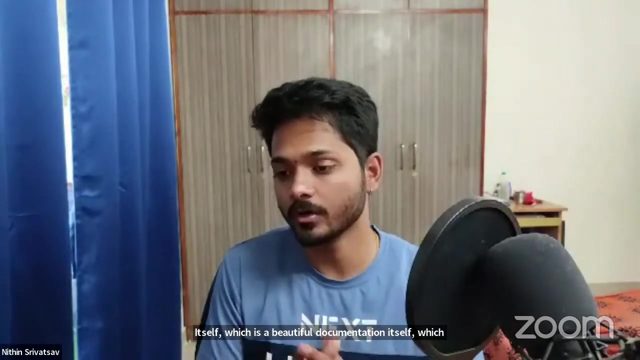 Okay, Okay, Okay, Okay, Okay. Any source for learning QGIS? Yes, Uh. so there's the QGIS website itself, which is, uh, a beautiful documentation itself which, kind of uh, gives you an overview of how QGIS tool works. 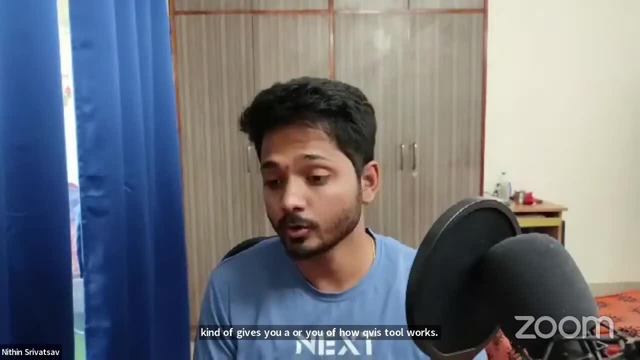 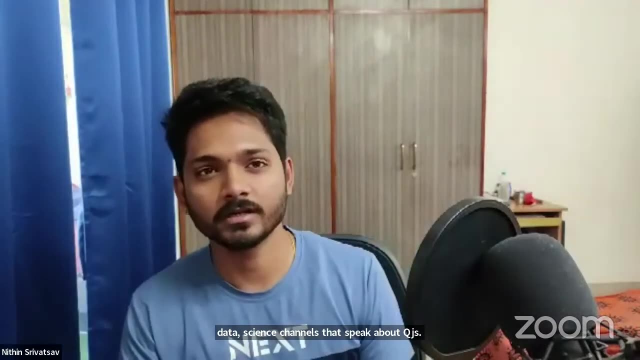 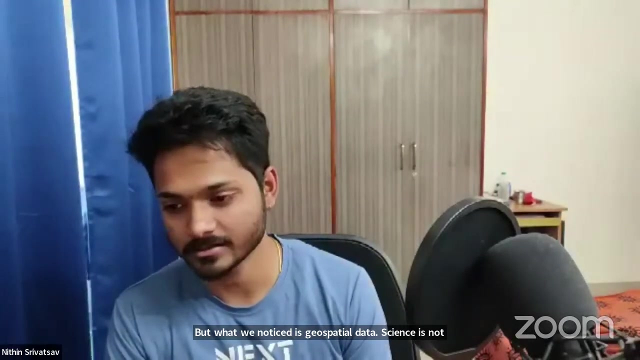 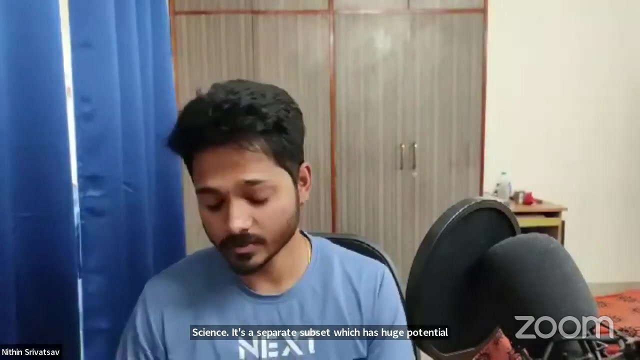 But apart from that, uh, there are a lot of YouTube videos, data science channels, that uh speak about QGIS, But, uh, what we noticed is geospatial data science is not as popular as your traditional data science. Uh, it's a separate subset which has huge potential of applications, especially with 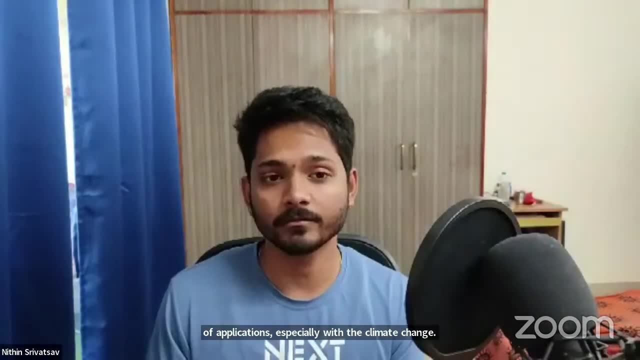 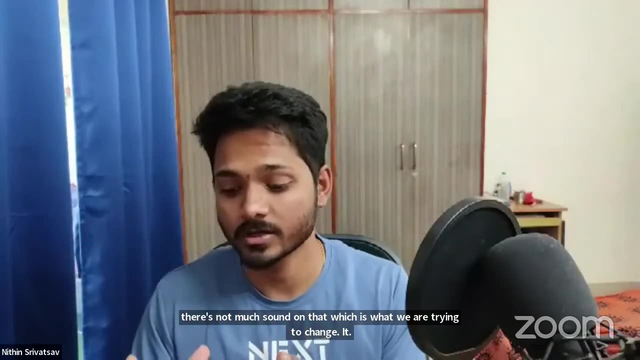 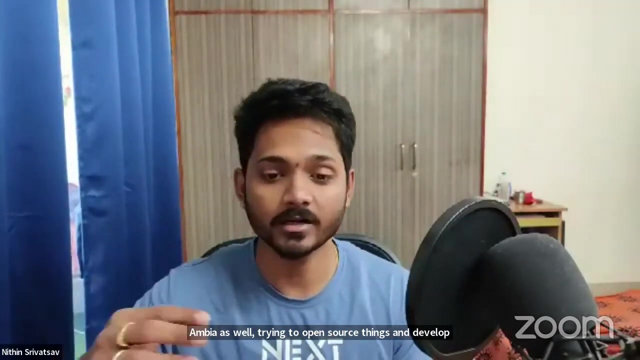 the climate change awareness that we are going into, But apart from that, uh, there's not much sound on that, which is what we are trying to change at Ambi as well: trying to open source things and develop tools that will enable enthusiasts like you to get started with uh. geospatial data. 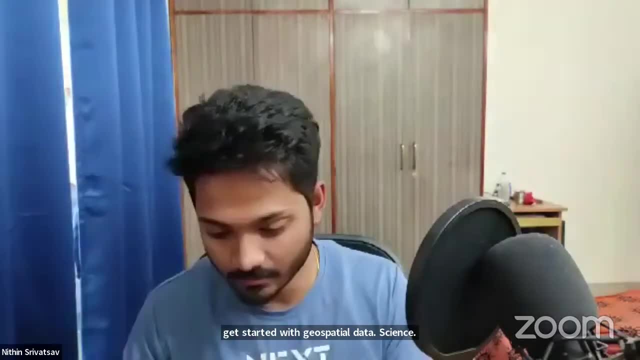 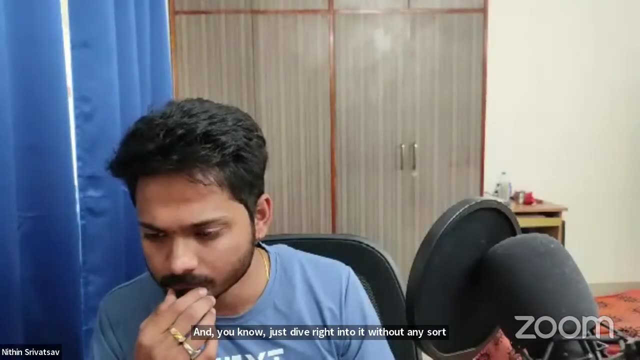 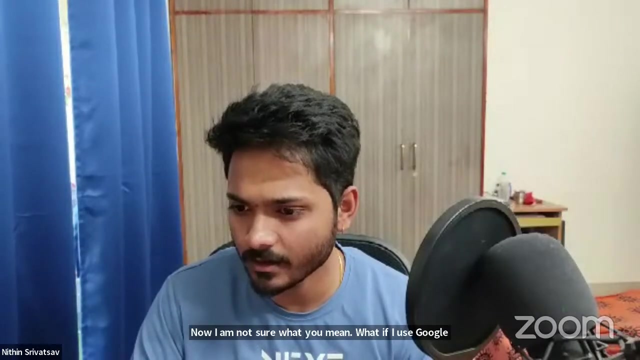 Uh, geospatial data science and, uh, you know, just dive right into it with uh, without any sort of resistance and complex stuff. Now I am not sure what you mean. What if I use Google earth engine for extracting data? 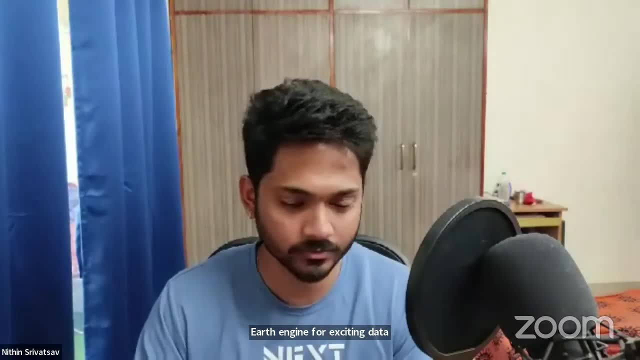 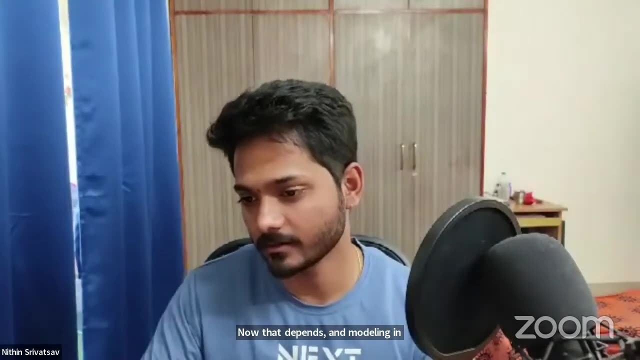 Uh now, what sort of data are you trying to extract? now, That depends, and uh modeling in Python is straightforward. I think Uh Probably, if you want data that you can uh map to, yeah, Satellite data, Yes. 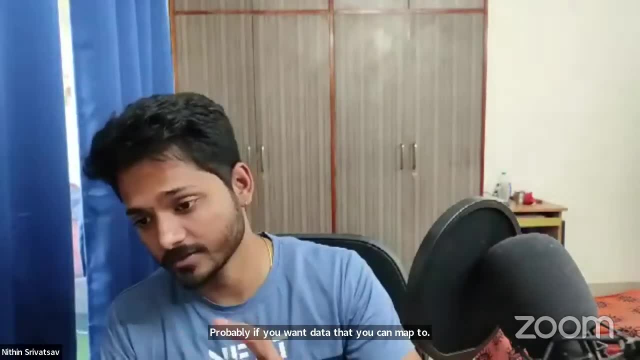 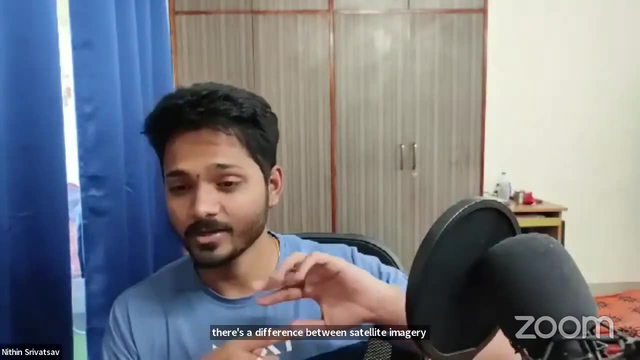 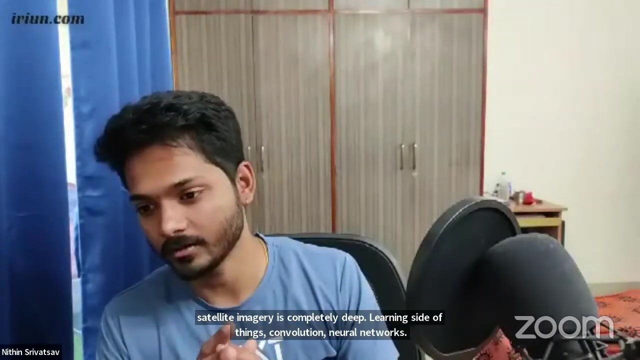 So if you want satellite data, no, there are two differences. Again there, there's difference between satellite data and there's a difference between satellite imagery. Now, satellite imagery is completely deep learning side of things- Convolution, neural networks- but this data is more Python oriented. 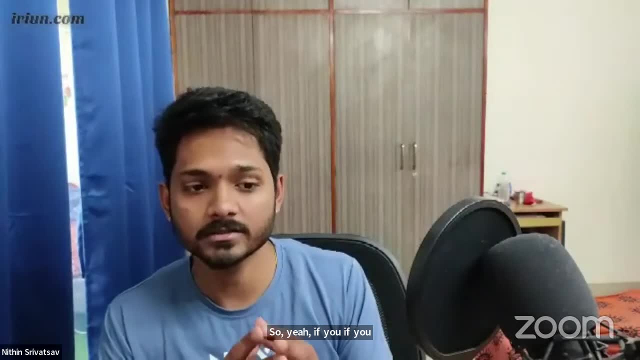 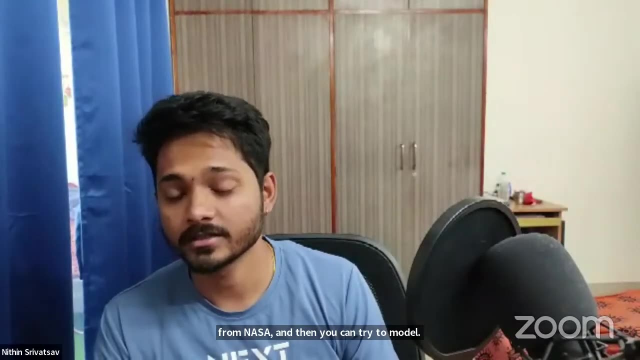 So yeah, if you go, if you can get your hands on data sets from NASA, uh, and then you can try to model. So there are, I think there are also a couple of uh data sets. There's one from Ambi. you can pull in weather APIs, pull in APIs and model on top of that.